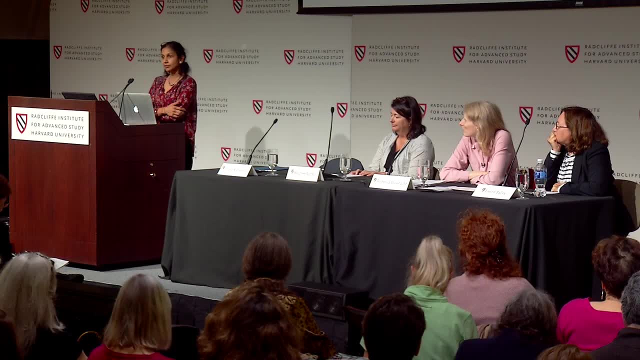 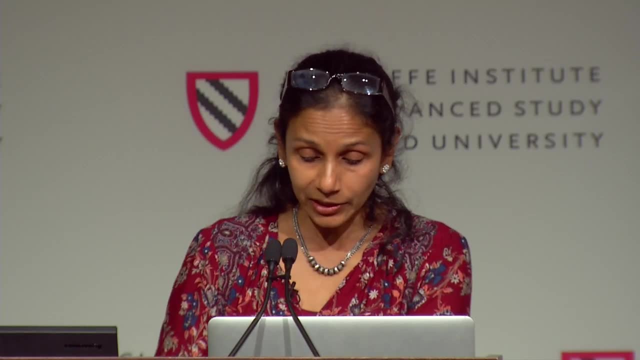 You know, we have seen that the inception of life, the evolution of life, happened on the ocean. But also the oceans regulate the atmospheric carbon dioxide and oxygen, And the oceans contain, for that matter, a very large percentage of the Earth's water- 97%. 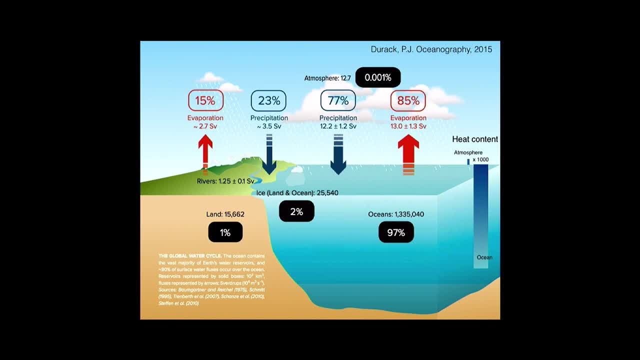 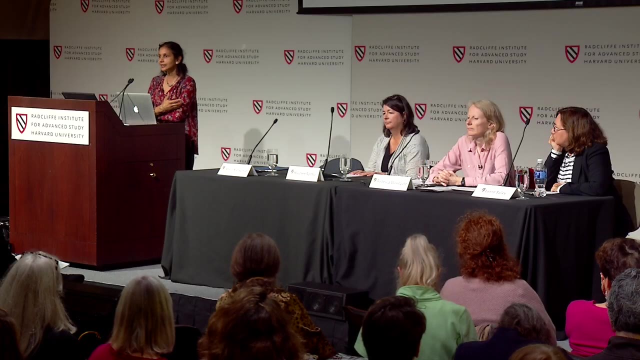 of the Earth's water is in the oceans. Just about 0.001% of the water is in the atmosphere. just to give you an idea, The oceans contain 98% of the carbon dioxide in dissolved form, of course. So when we say that atmospheric carbon dioxide is going up, 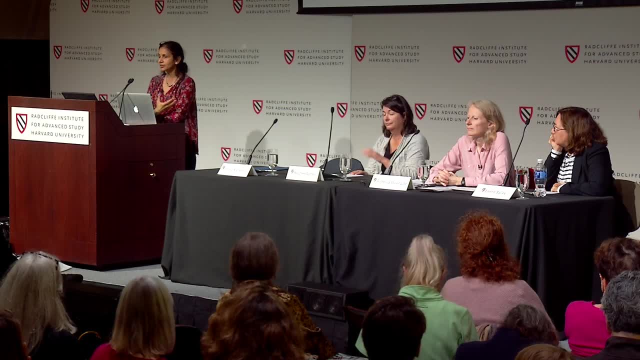 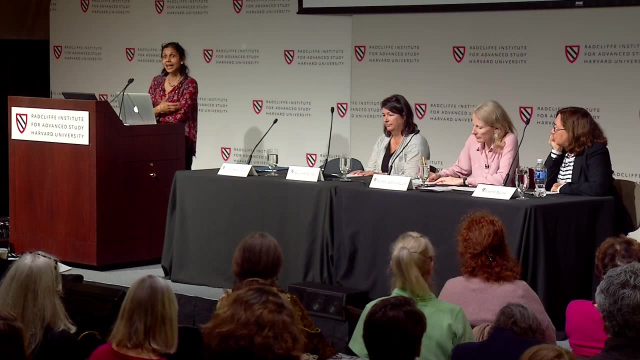 or going down. you have to realize that there is a lot in the oceans, And the oceans have in the past regulated the atmospheric carbon dioxide very well. Whether they can do that in the future is something that we are still asking. And the oceans, you know. if you think. 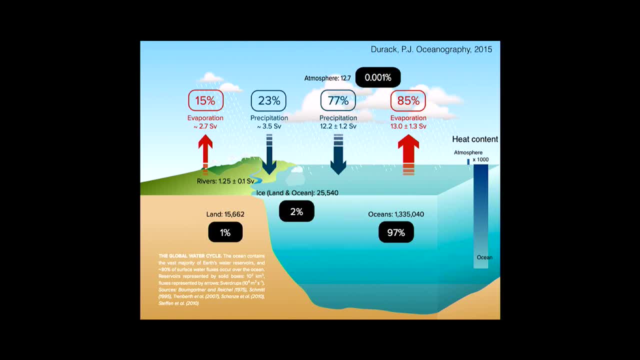 about heat. where is all the heat? Most of the heat, 90% of the heat, is in the oceans. So in many ways the oceans define the climate. The circulation of the oceans defines the climate And about half. 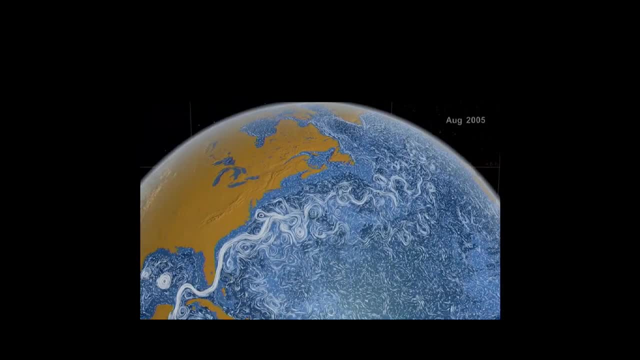 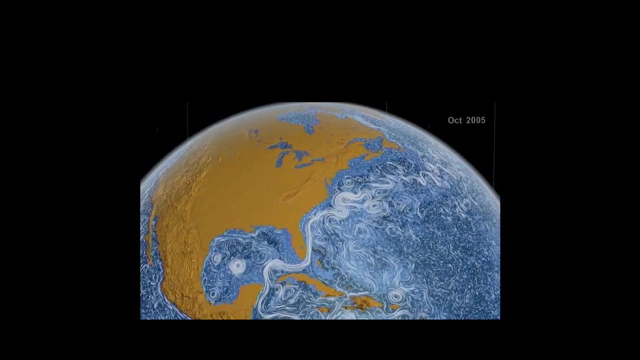 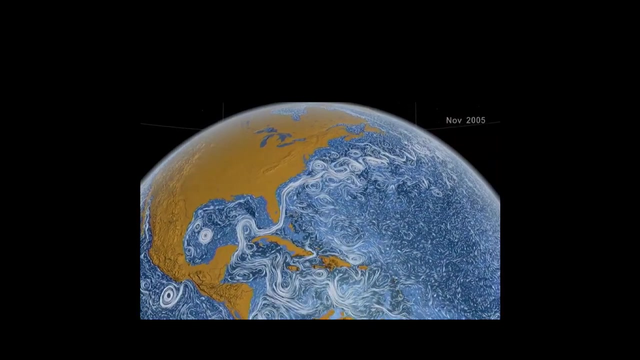 the primary production on the Earth takes place in the oceans, And we see that the oceans are constantly in a state of motion. These ocean currents, they transport heat across the oceans, They transport salt And in a very fundamental way, the oceans are different from the atmosphere. One is that they have a huge 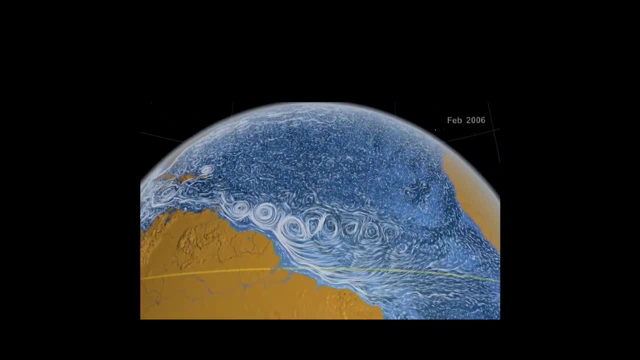 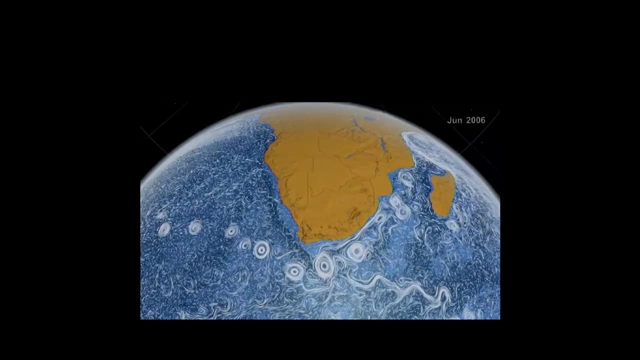 enormous heat capacity, But the atmosphere is heated from below, And so the energy of the sun is what drives the atmosphere, Whereas the oceans. when you heat them by the sun, in fact it stratifies the oceans or it creates a density contrast, because warmer water doesn't. 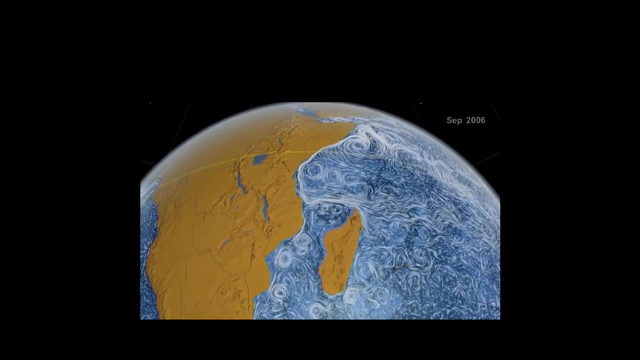 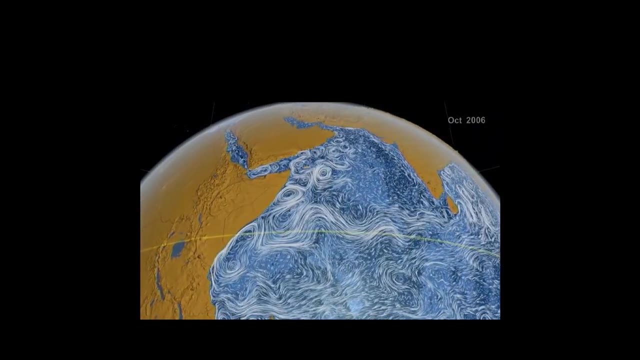 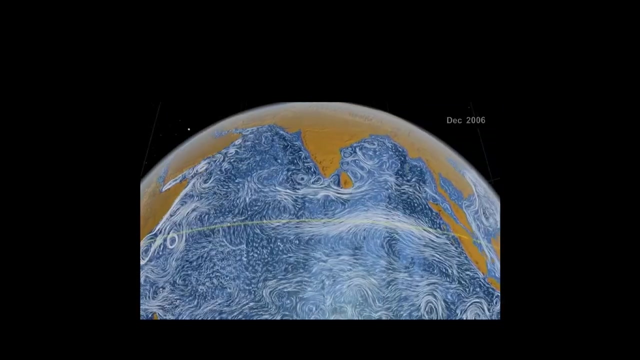 sink. So, in fact, you see that the winds are what drive the ocean to a large extent, And mixing or overturning the oceans is, in fact, very diff, difficult, because the sun, on the other hand, forms the oceans. So, in a nutshell, that tells you that it's difficult. 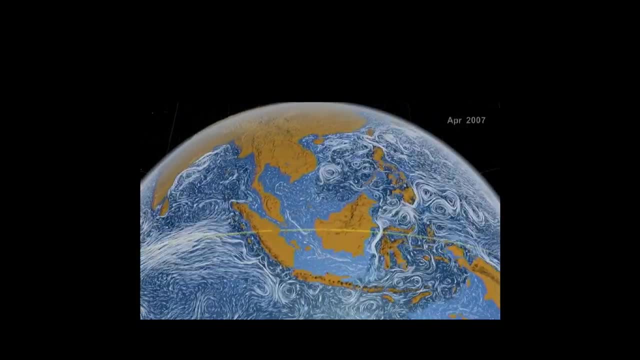 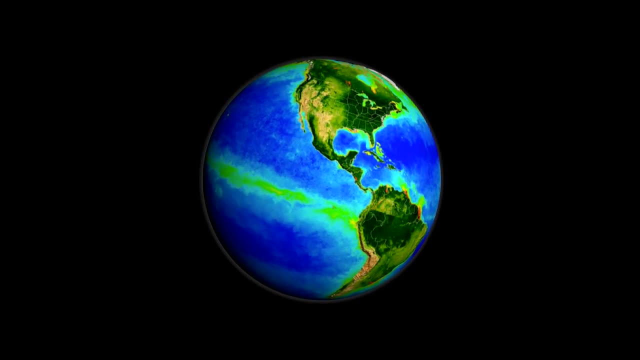 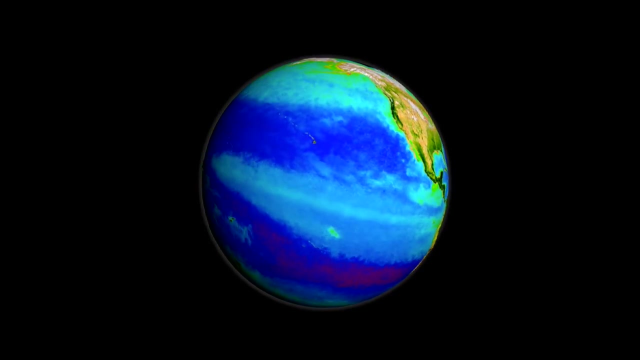 to communicate changes through the oceans. But the oceans really support a large part of our primary production on this planet And so about half that primary production takes place in the oceans And that organic matter, as we've seen in some of the previous talks, it sinks very gradually. Some of it gets sequestered- that carbon- to the oceans. 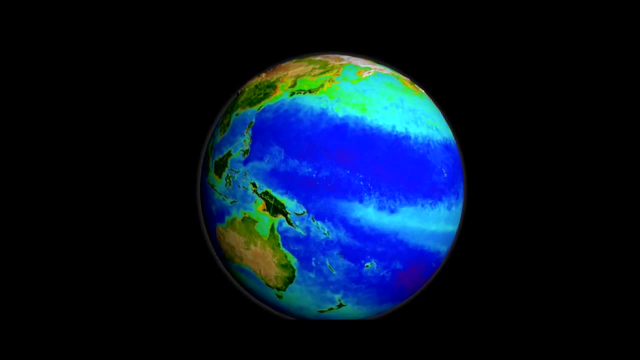 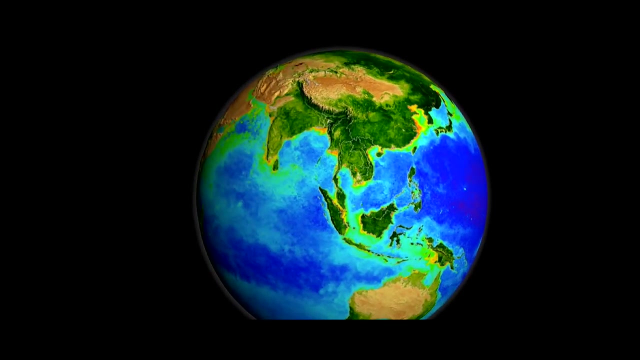 So the big perturbation that we've made, that humankind has made, is that we've made a lot of changes. We've taken out that carbon, that organic carbon that's fossilized for millions and millions of years. We've very abruptly brought it out into the atmosphere. 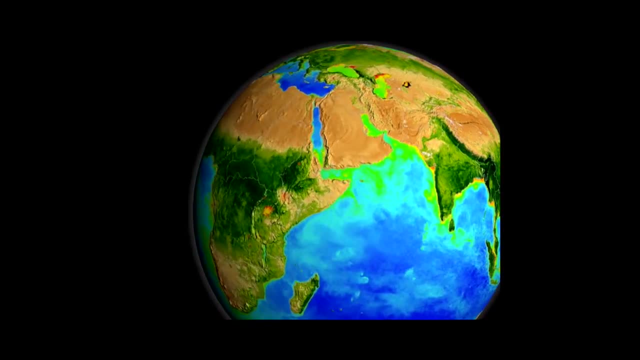 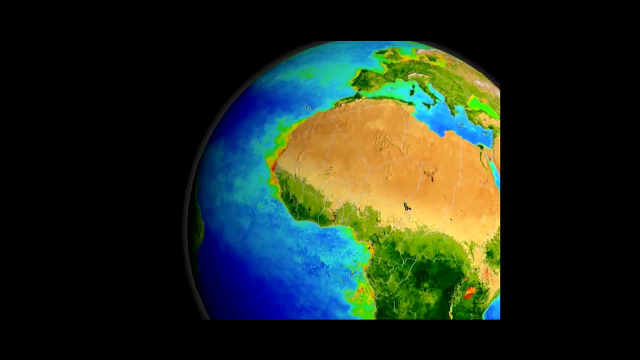 And we have created huge changes And I have to say that the ocean has buffered, is buffering a lot of that change that we might see. because of those abrupt changes, A third of the CO2 that we put out in the atmosphere has gone into the oceans. And when we talk about global 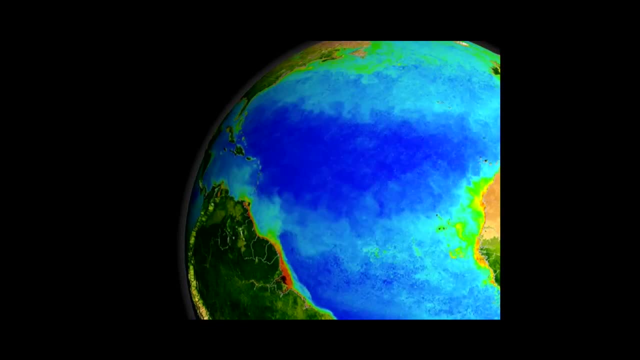 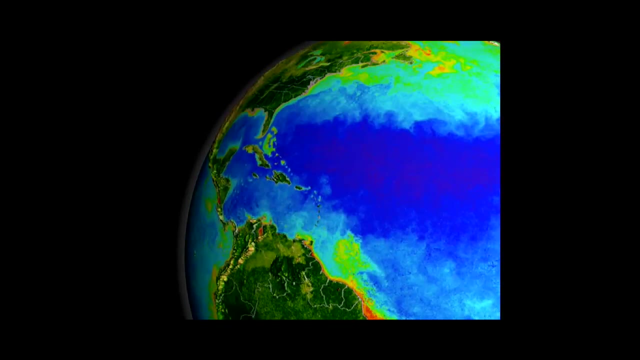 warming. and if you were to ask: where is all that heat that has to do with global warming. why is it that we don't feel very warm today? it's because 90% of that heat is in the oceans. So I'm really excited today to have this panel here. We have here three oceanographers whom 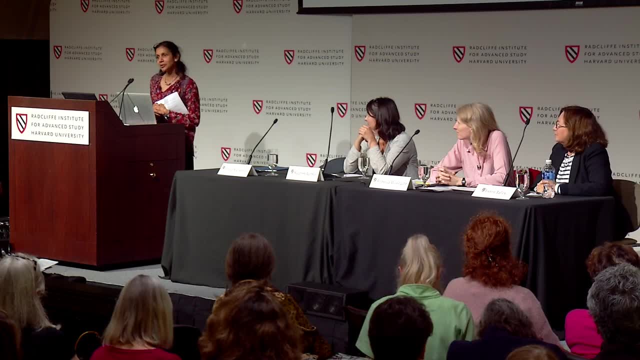 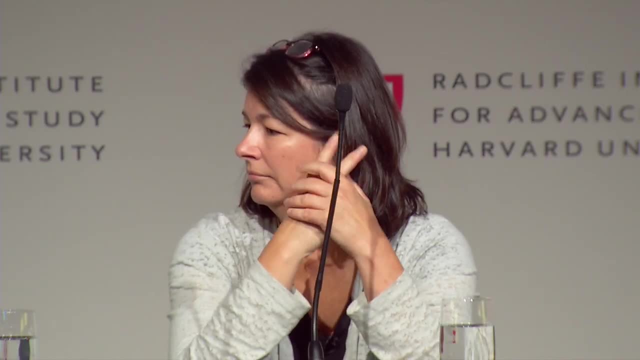 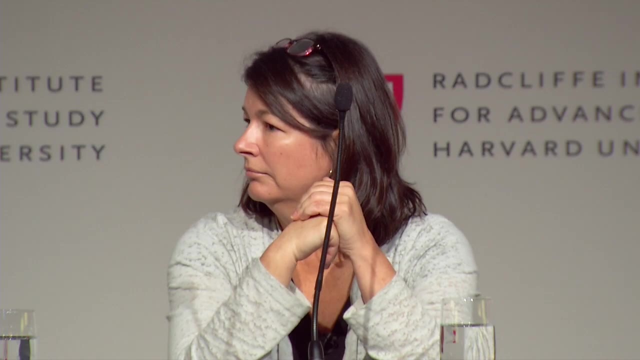 I really admire whose work I've really admired Maureen Ramo from the Lamont-DeHurte Earth Observatory at Columbia, And she has worked on the past climate of the Earth And her work has shown how important it is to think about past climates and how past climates 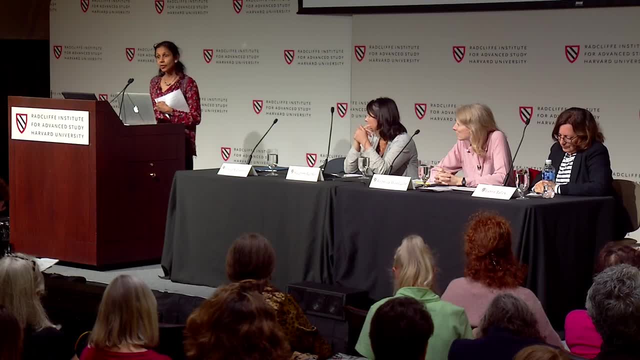 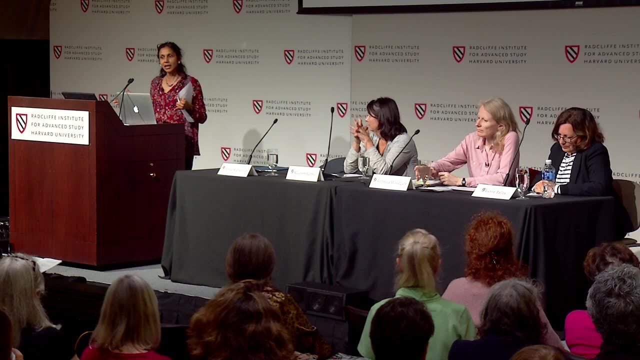 help us understand the changes that we are going to go through now or we are going through at present. That's because we have a very short observational window in this last few decades, And so understanding past climate is really important. And then we have 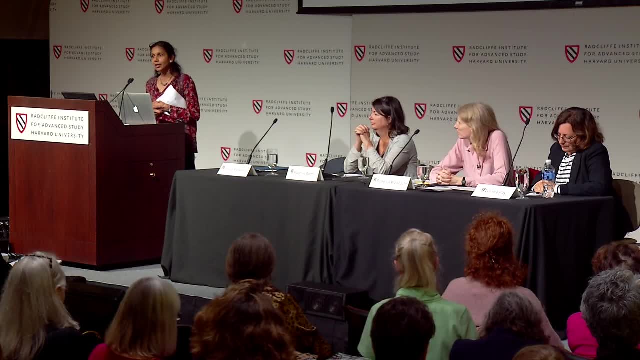 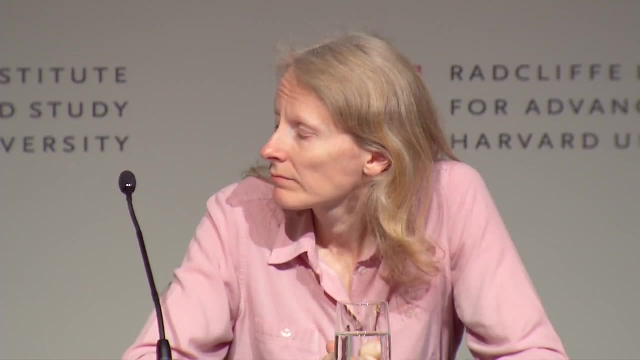 Rebecca Woodgate, who is an Arctic oceanographer, And she's done a lot of observations in the Arctic And she's really pushed our understanding of how sea ice and the oceans interact And the big changes that are occurring in the Arctic. it's one of the most vulnerable. 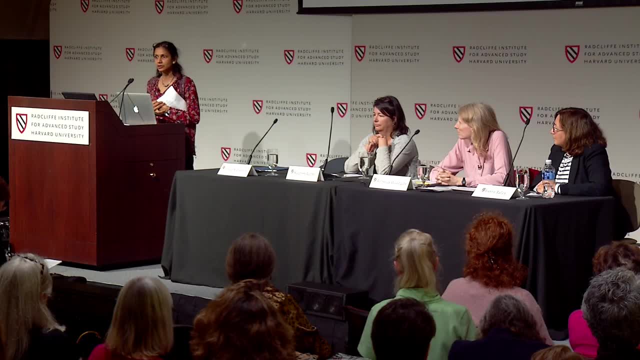 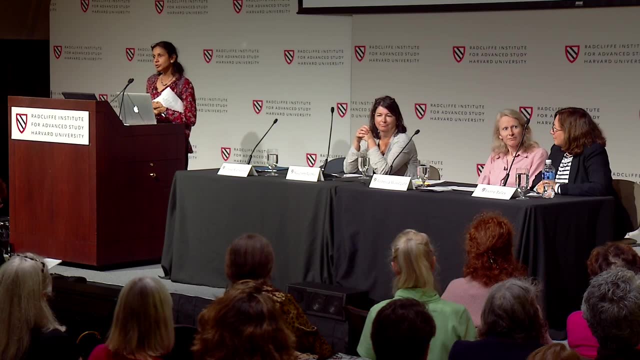 regions in the oceans because of the sea ice and the interaction with the oceans. And then we have Lynn Talley, who's been instrumental in understanding the large-scale distribution of temperature, salt and the global circulation of the oceans- How these things get conveyed. 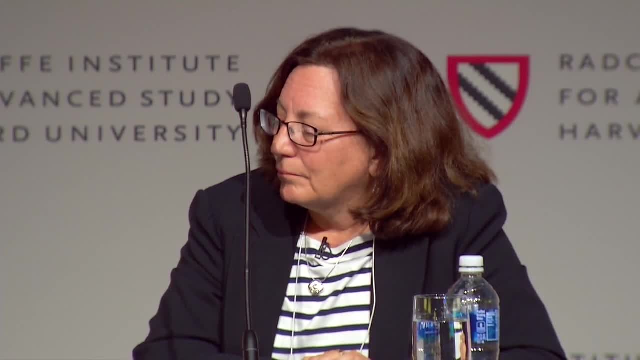 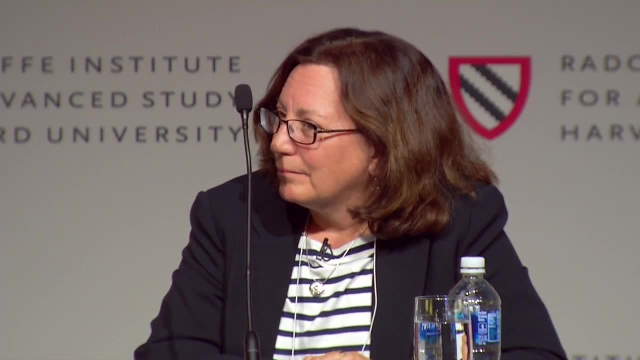 and transported across the oceans. What are the changes? And she's been instrumental in some of the very big ocean observing programs that have global and international programs, and her understanding of the global oceans through her work. So thank you very much, Thank you. 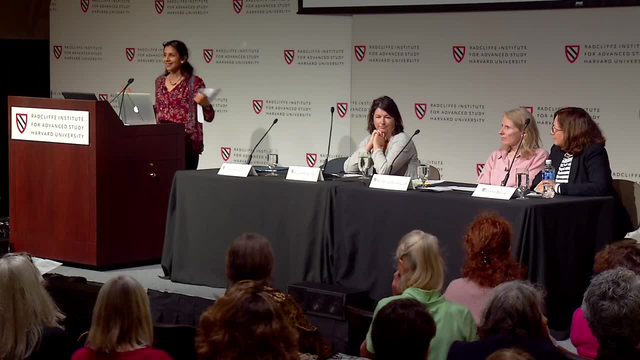 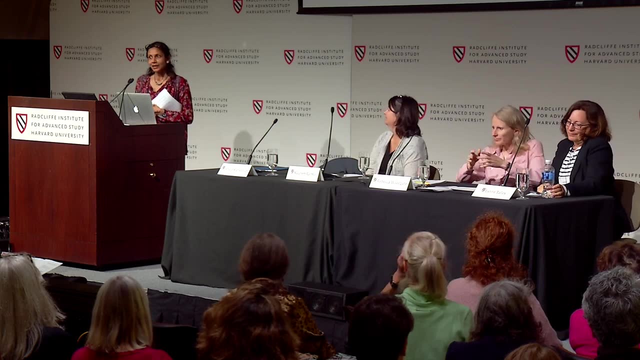 And so I think the opportunity to really do those programs has really changed a lot of our understanding as oceanographers. So it gives me enormous pleasure to have these three people here today. I don't want you to go away thinking that oceanographers are necessarily. 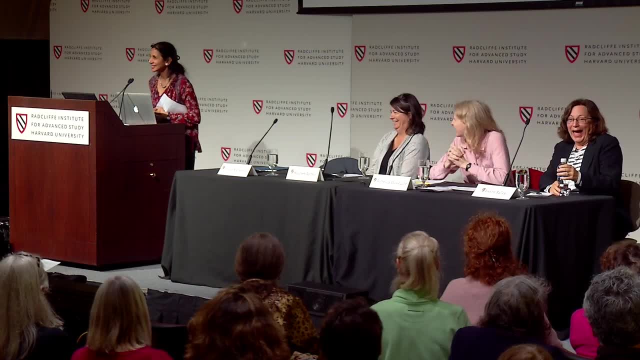 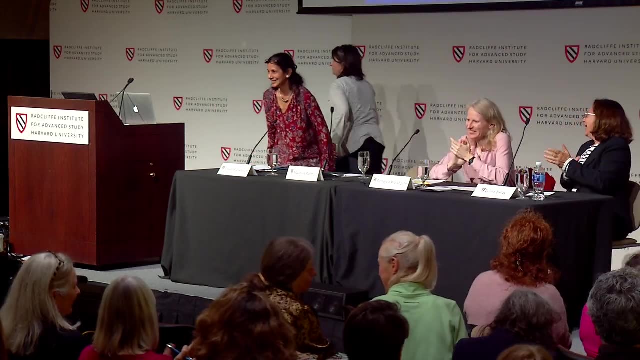 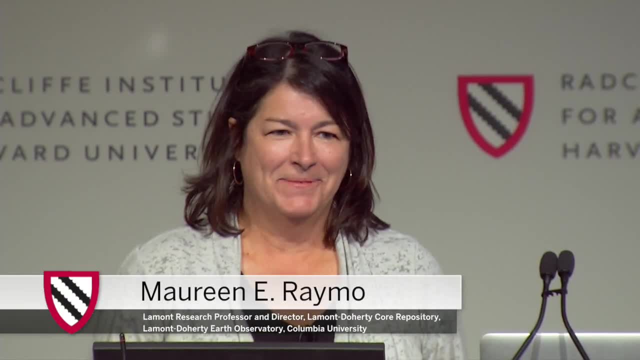 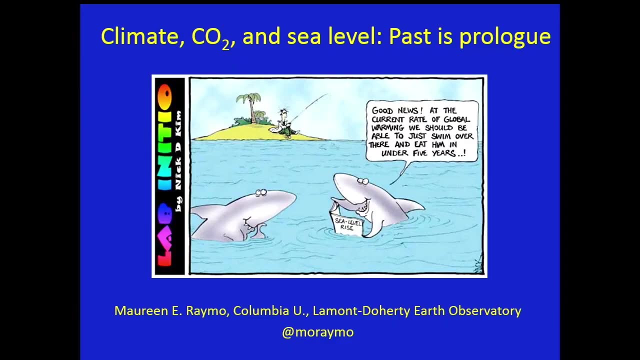 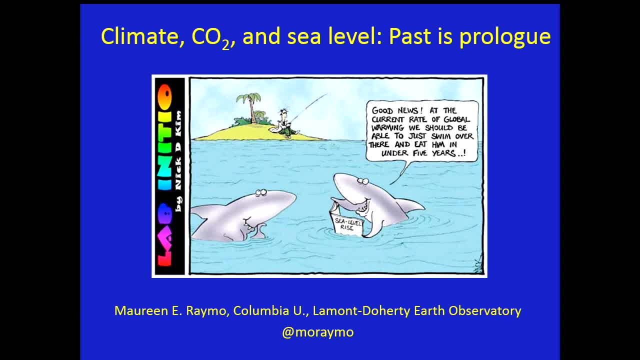 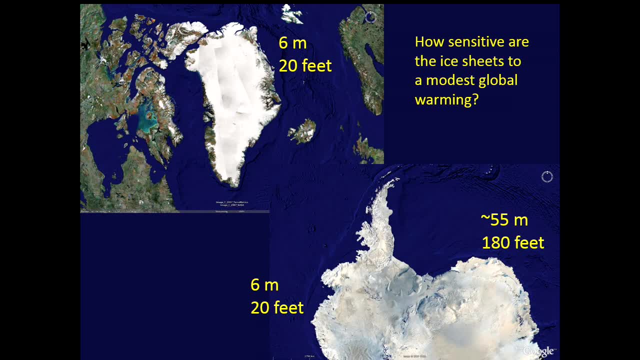 called perpetual ocean. if you want to pull it up and watch the whole world, okay. so I've spent most of my career studying past climate change and, in most of the last five to ten years, studying sea level as it relates to the past history of the polar ice sheets and- and today there's two major polar ice sheets- 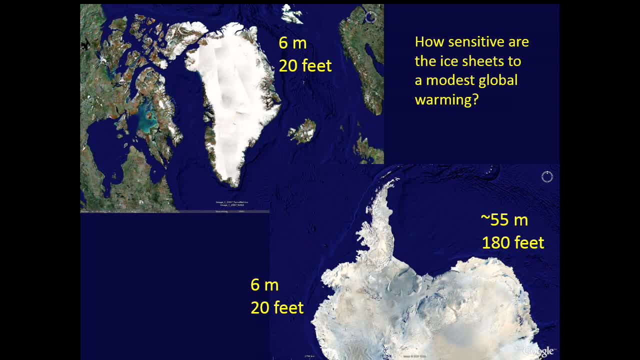 there's the one in Greenland which, if you hypothetically could melt it all and spread it in a single layer over the ocean- if you'd have, sea level would rise by about six meters or twenty feet. and then in the South Pole there's the West Antarctic ice sheet over here, which again is about the. 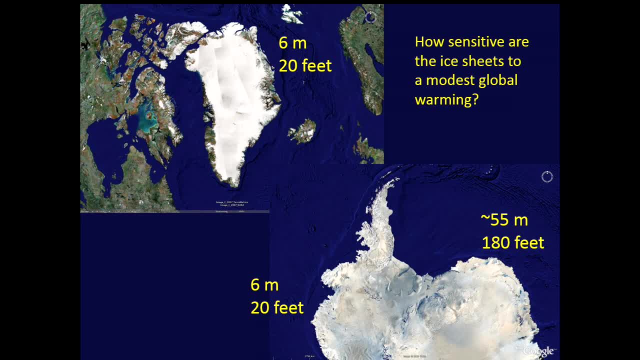 same size as the Greenland ice sheet and then the much larger East Antarctic ice sheet, which you have to go back 40 million years to find a time when that whole ice sheet had melted, and at that time sea level was about 180 meters, 180 feet, higher than today. so the question I'll just pose here is how sensitive are. 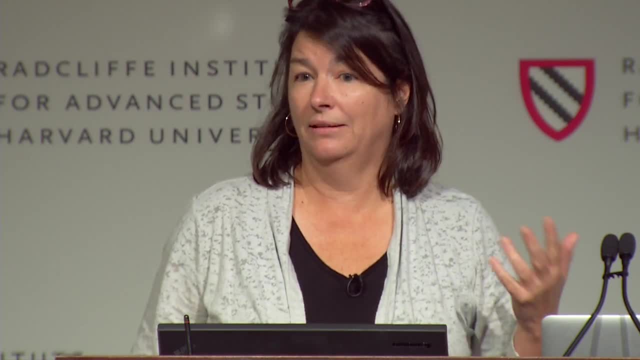 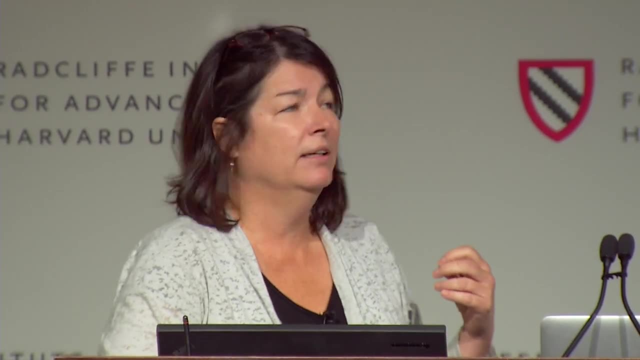 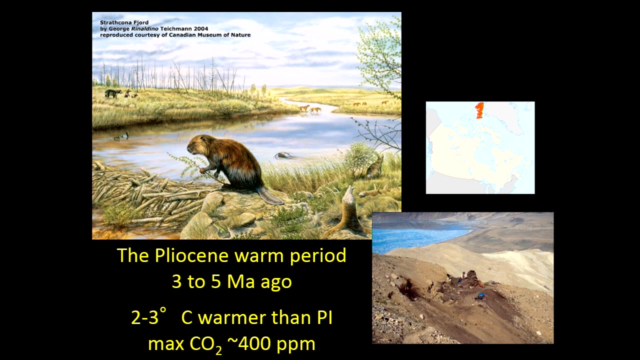 these ice sheets to a modest global warming, and by modest I mean, let's say, one degree Celsius warmer than today. I actually know a little bit about a time period that is widely agreed to have been two to three degrees warmer than pre-industrial, which would be one to two degrees warmer than today. 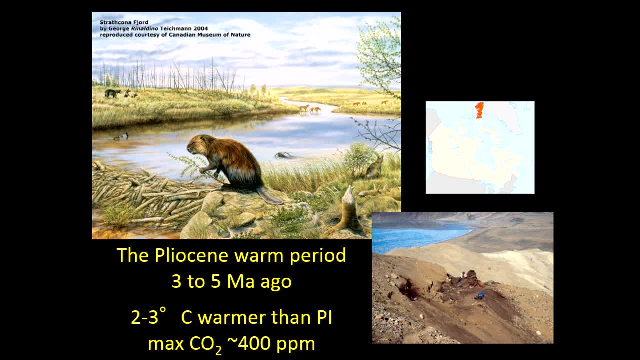 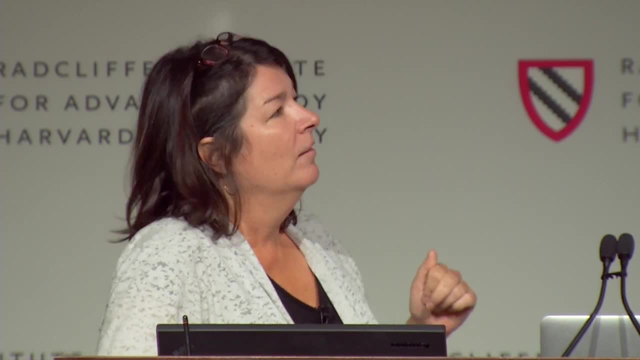 and at that time, geochemists using various methods have reconstructed atmospheric co2. it is about 400 ppm, which I know- at least some of the people in the room I recognize know that's exactly what it is today. it's about 401 this week ppm. it should be 280 ppm, but 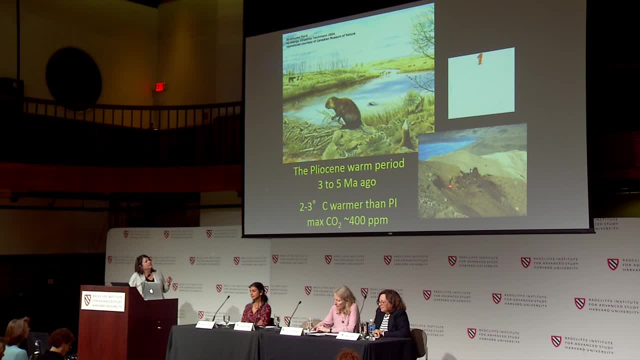 we'll come back to that, and what I'm showing here is a site on the north coast of Ellesmere Island and an artists reconstruction based on the fossils and plants and animals and pollen that have been taken out of that dig show a reconstruction of what the north coast of Greenland and Canada looked like. 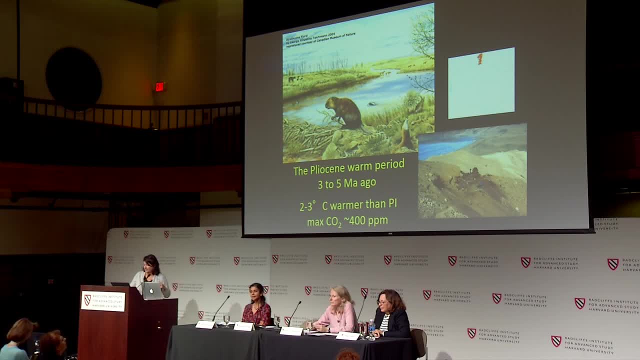 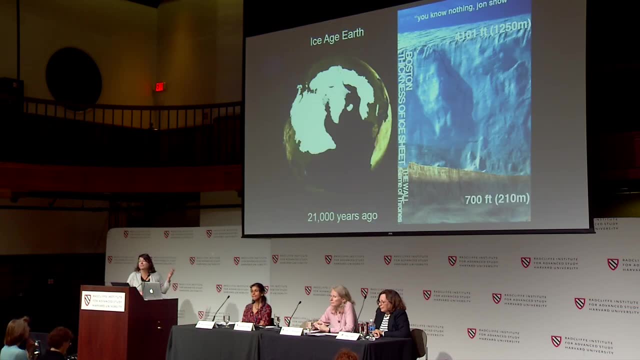 three million years ago, the Greenland ice sheet did not exist. okay, so climate is changing all the time. even more recently, there's been a profound change in climate. this is a beautiful picture of Greenland ice sheet here. this is a. this is 21,000 years ago- very recently- and obviously the Greenland ice sheet 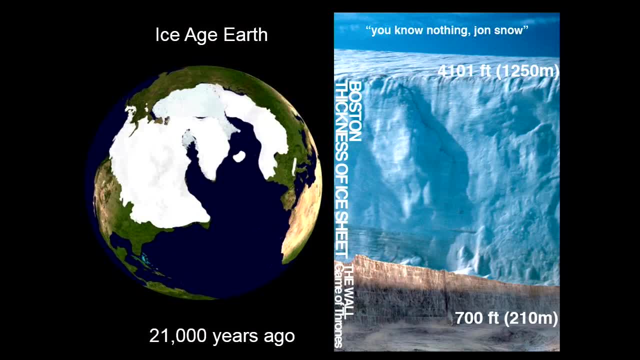 has jumped the Davis Strait and has expanded dramatically down over North America and Fennoscandia. I don't know if this is a big Game of Thrones crowd in here. if the people that like it will appreciate this quote. so that is the side: the height of the ice sheet over Boston at the peak of the last ice age. 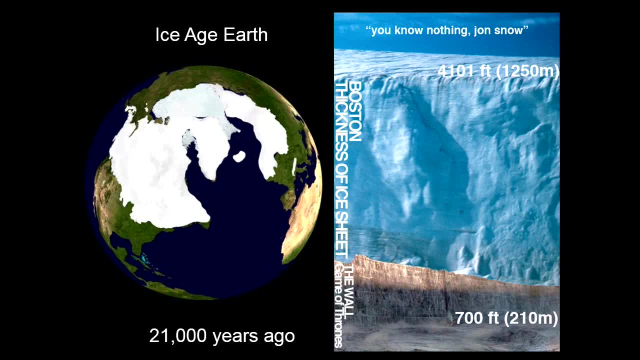 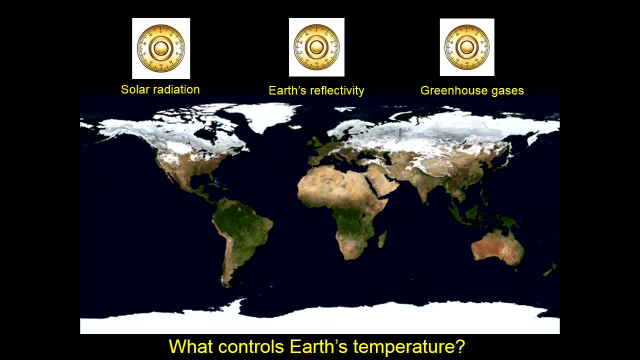 okay, and so that was just a blink of time ago, obviously. so why do these changes happen? the climate system is infinitely complicated and there's no scientist on our planet that can be an expert at every part of the climate system, and but at the same time, it's somewhat very simple, and you know you. 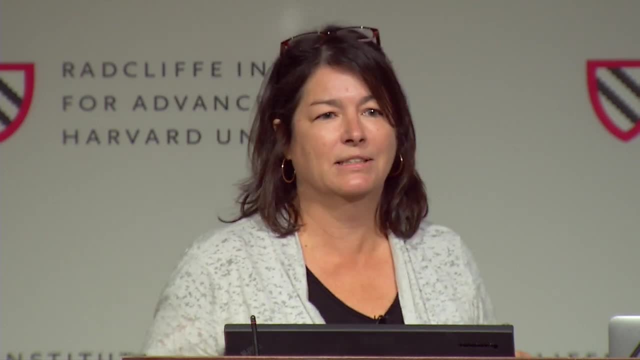 can go to the radiation chapter in a physics freshman physics book and see a very simple example of a climate system. and you know, you can go to the radiation chapter in a physics freshman physics book and see a very simple equation to calculate the effective temperature of the earth. we 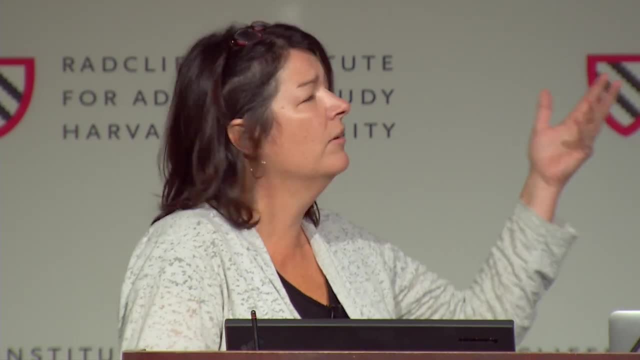 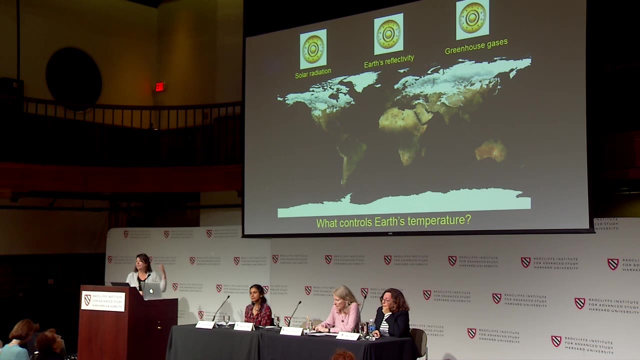 don't need that, but all you need to know is it's very simple, and this and the surface temperature of the earth just adds one more variable, which is the concentration of greenhouse gases, and so I like to think about it when I talk to a general audience is just say: look, you know the Earth's climate, the temperature, 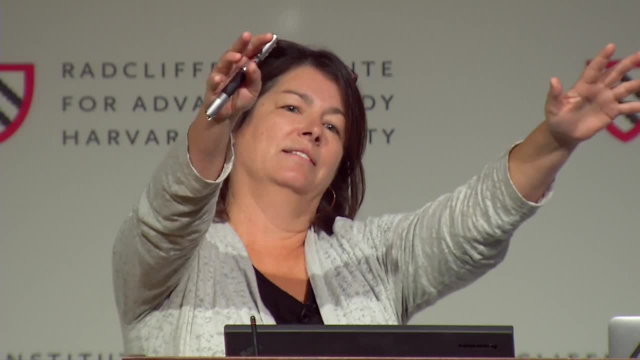 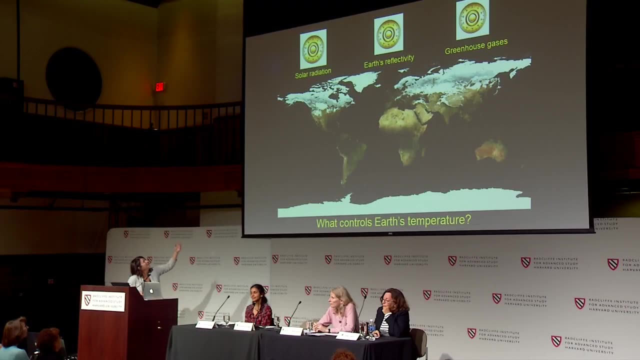 of the earth. we were a ball of rock. we get heated by this star that's, you know, a distance away- one light year, I don't know- and and there's three variables that control the Earth's temperature: how close we are to the Sun, and that actually varies subtly through time because our 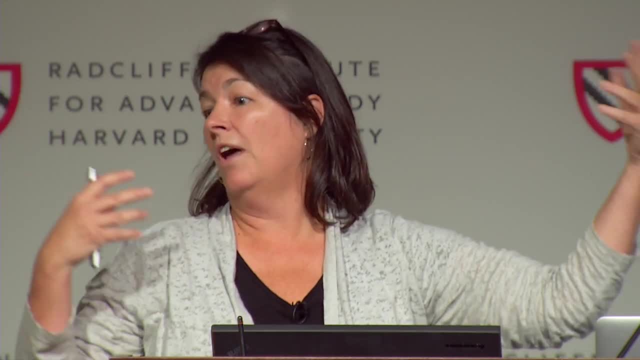 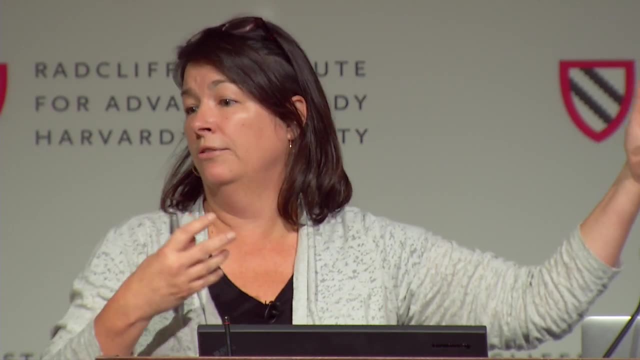 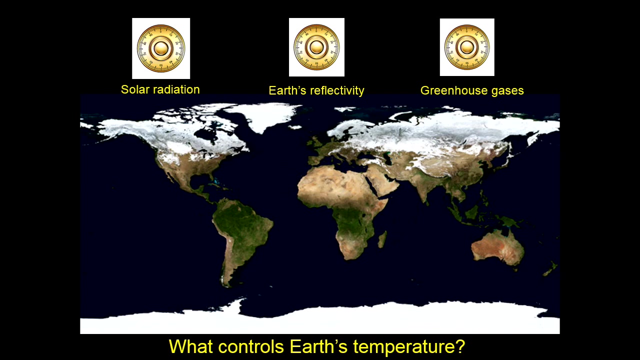 orbit isn't perfectly circular. circular and other large planets perturb our orbit, like Jupiter and Saturn, on time scales of tens to hundreds of thousands of years, in very predictable ways that can be calculated, and sometimes over billions of years. the solar output of the Sun can change, but on 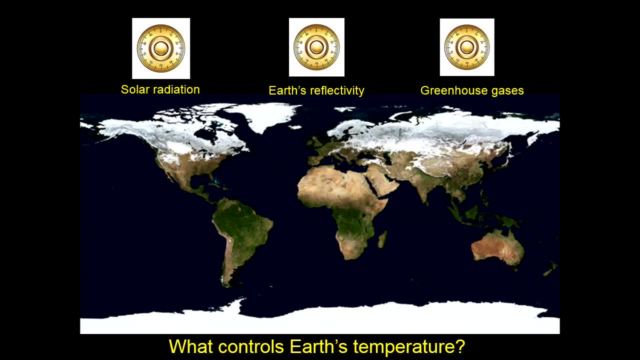 human time scales. it's essentially constant, which is why we call it solar constant. so that's one big knob you can change that can control Earth's temperature. the other is the Earth's albedo or reflectivity. if you expand the snow and ice coverage at high latitudes, you make the earth more reflective and 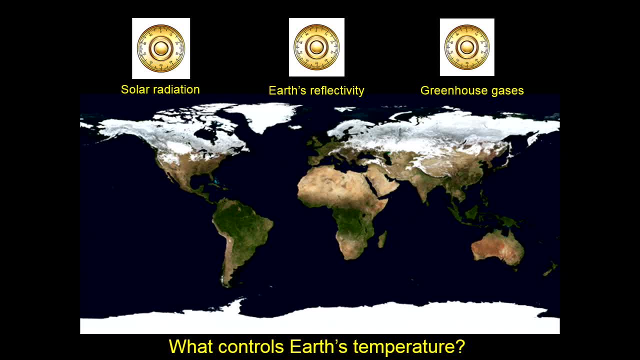 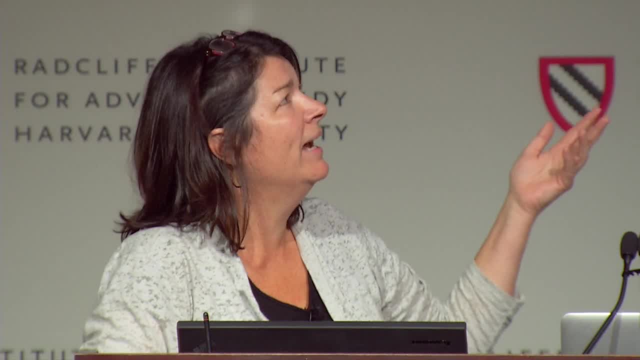 so more. the solar radiation is just lost to space, it's reflected to space. it's not available for heating. I'm sure we'll hear a lot more about that in the Arctic talk. and then, finally, we have this thing called greenhouse gas. is and you know so we have all this heat coming in from the Sun. it's warming. 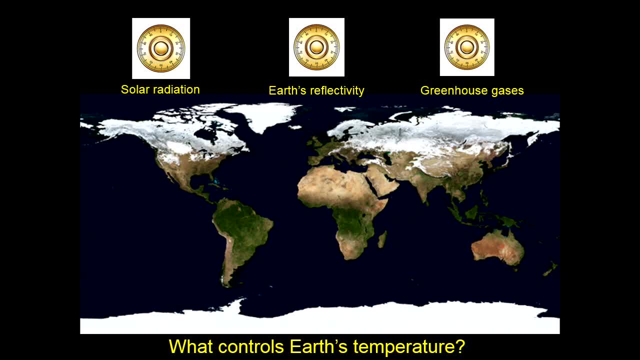 the Earth's surface. the surface is cooler than the Sun, so it radiates outward at longer wavelengths and it just happens to interfere with the molecular structure of certain gases, especially co2, which can prevent it from escaping. and then we radiates it back to the surface. you know, just like throwing. 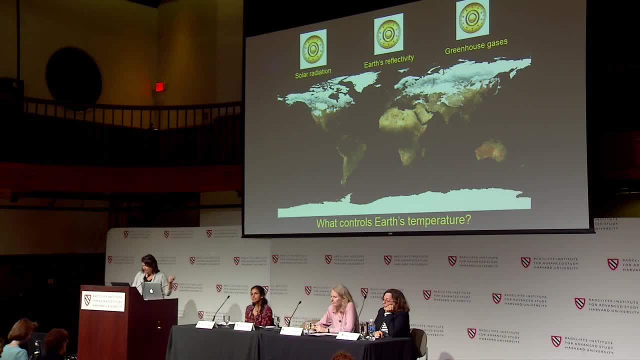 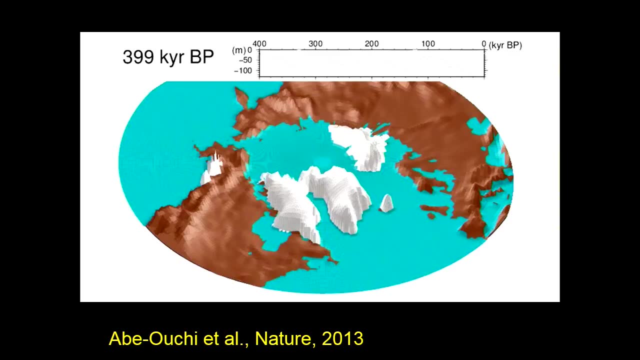 more blankets on on a cold winter night. so these are the three knobs and you know everything I know about. every climate change that has happened in the past and in this I will show you- can be explained by just changing these three variables, and I'm going to show you a 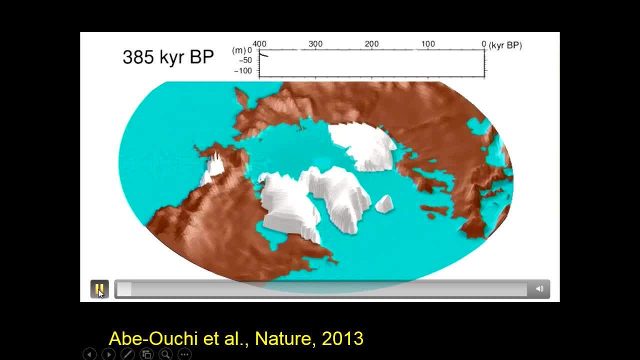 model. this is the climate model with an ice sheet embedded in it, and it's the last 400,000 years. this is a sea level scale, and this is what the climate of the last 400 years has looked like, just the only variables being our variable. 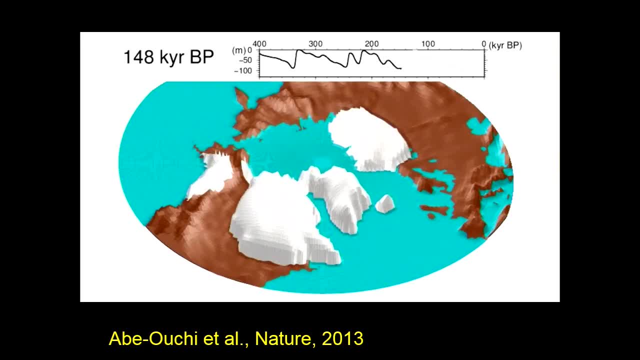 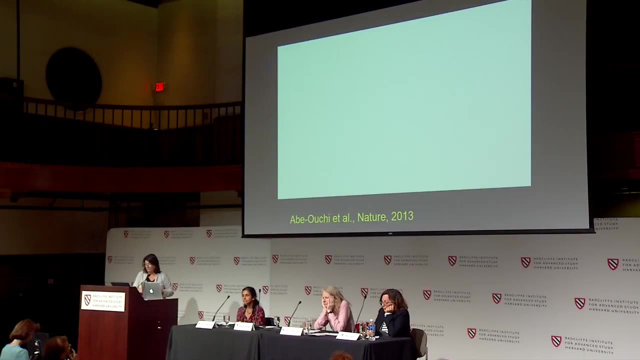 orbit around the Sun, changes in the Earth's precession and tilt of the Earth's axis, and the co2 changes that we know occurred from Ice cores and it actually this is a model result, but it looks remarkably like what we know climate did. You want to see that again? 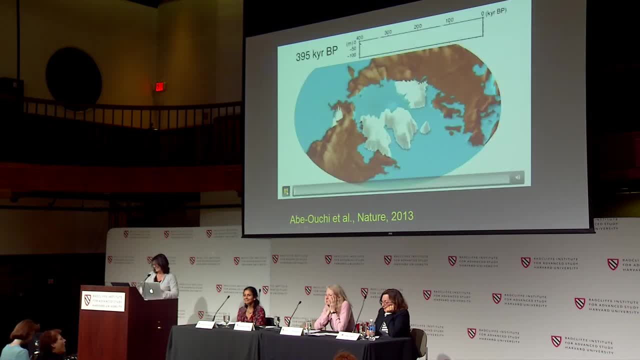 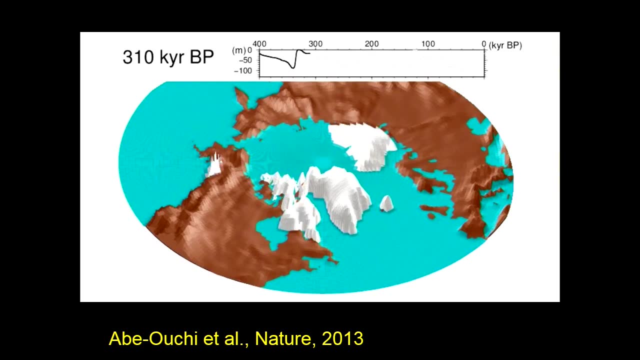 I could watch it all day. this is a. this is a paper we published in nature by Ayako Abeochi, who is actually the only female scientist I've ever met in my field, from Japan, so I'll show you. so one of the things you may notice is: 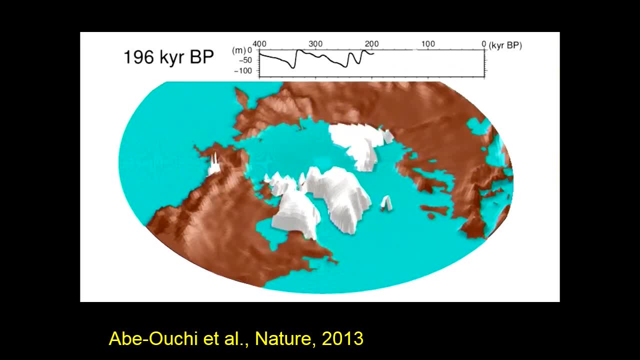 that ice sheets grow much slower than they melt. it's very easy to melt an ice sheet quickly, and the reason is is because, as you see, as it starts to retreat, the ice sheet has depressed to the land under it, and so the ocean can flow in very quickly and destroy that ice sheet from below as well as from. 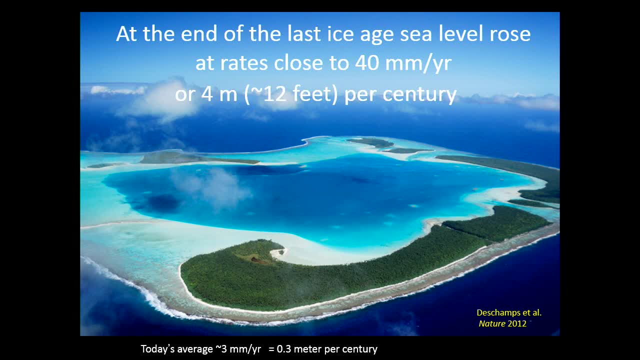 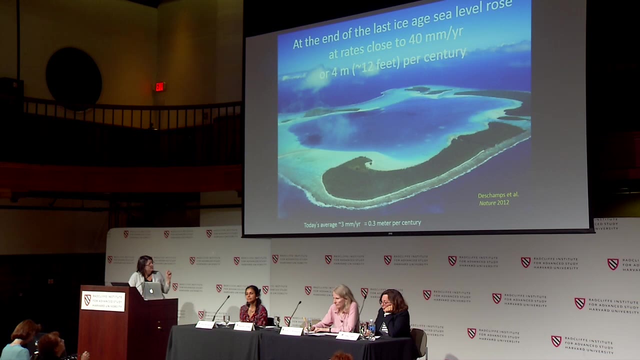 above. so ice sheets can melt very quickly because they can become unstable and warm ocean can flow under them. how quickly this is data. well, this is the results of a study of Tahiti in the Western Pacific, and what the scientists did was they went offshore and they drilled down, and they can with very 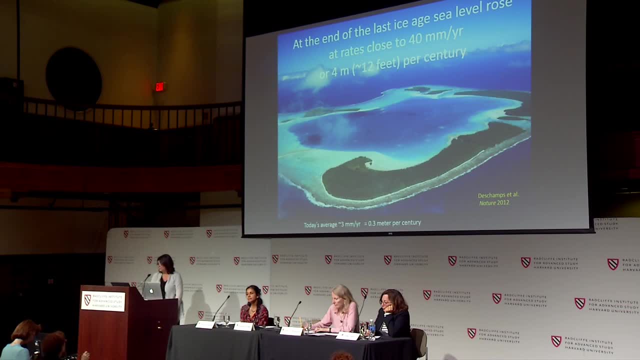 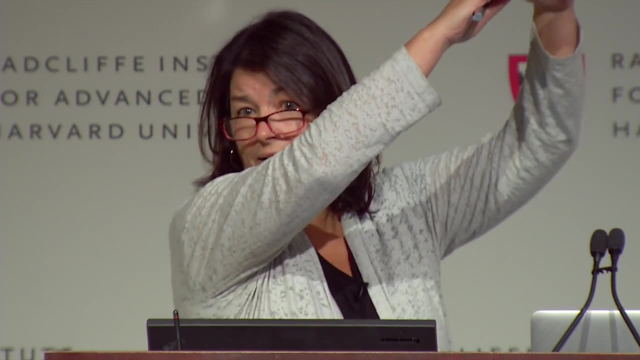 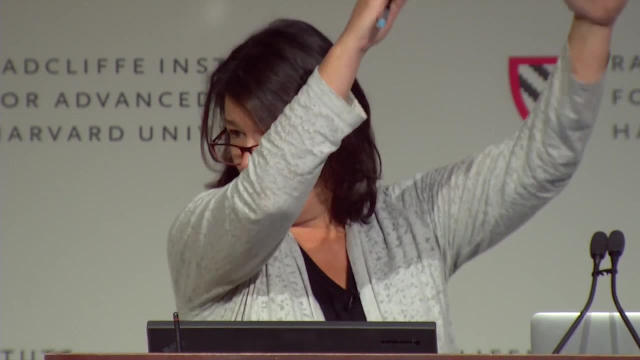 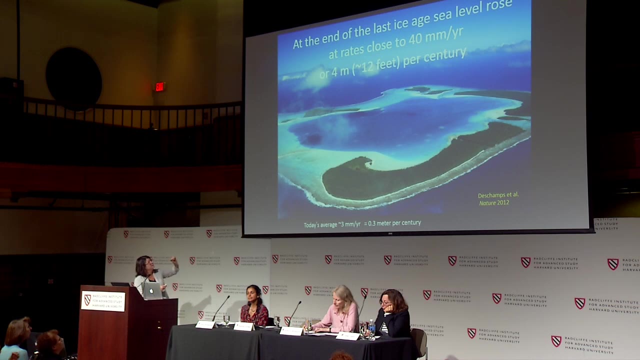 seas are rising. the coral is keeping up. okay, it's very it can do that. and they were able to determine that at the as the last ice sheet deglaciated sea level was rising at rates of 40 millimeters per year, or 12 feet per century. so keep. 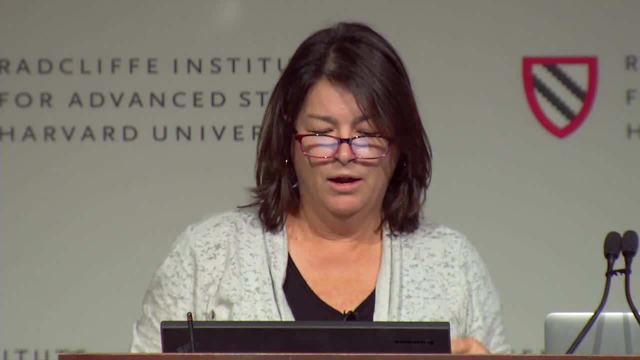 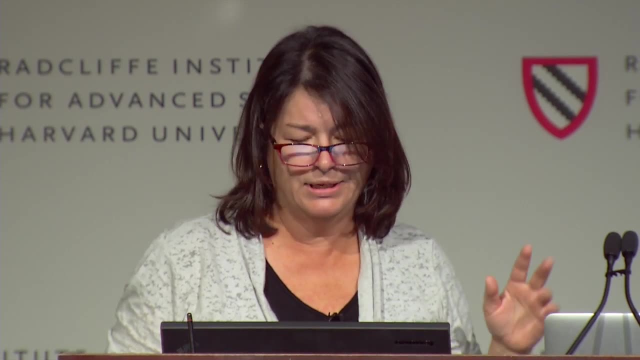 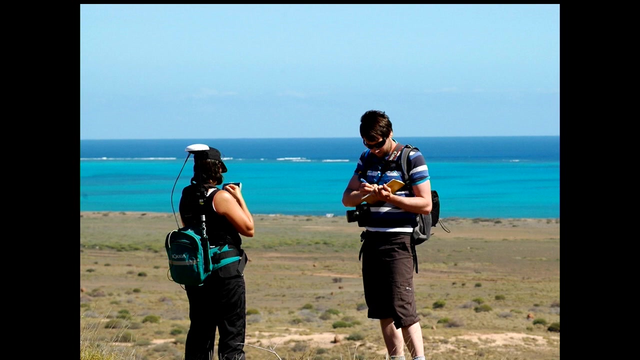 that number in head, in your mind, as we move forward here right now: sea levels rising at three millimeters per century. sorry, per year, did I say century of that year? three millimeters per year? so, but how high was sea level during some of these little periods in the past that? 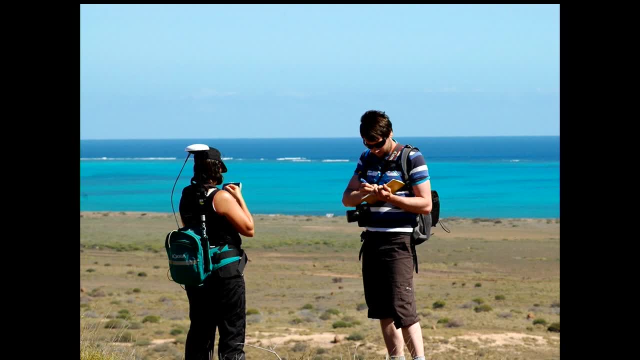 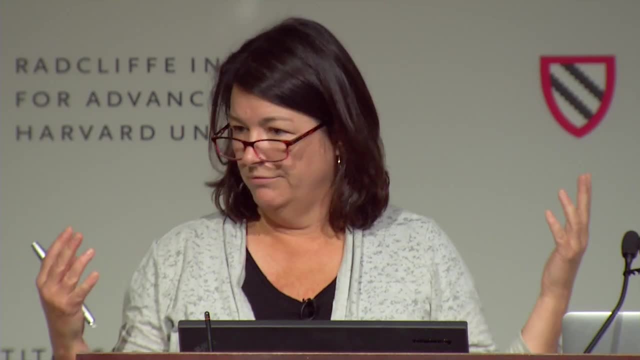 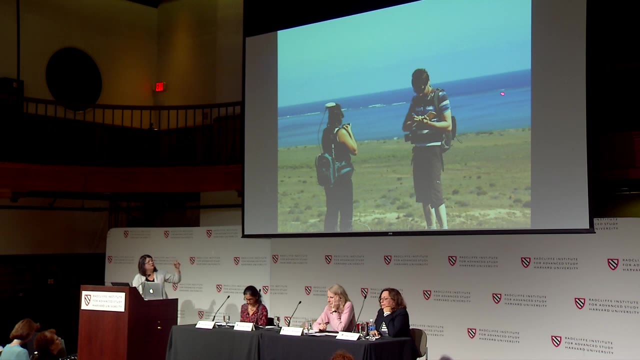 were just slightly warmer than today. this is a question that's very easy to answer and also very difficult to answer. it's very easy because the evidence for higher sea levels during the recent past is all around you. this is me standing with my postdoc, mickle leary. this is the modern Ningaloo reef system in Northwest. 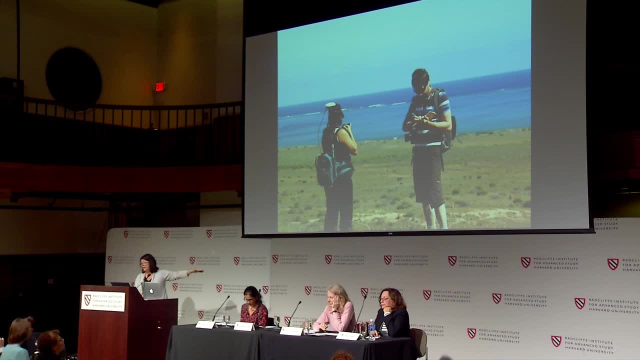 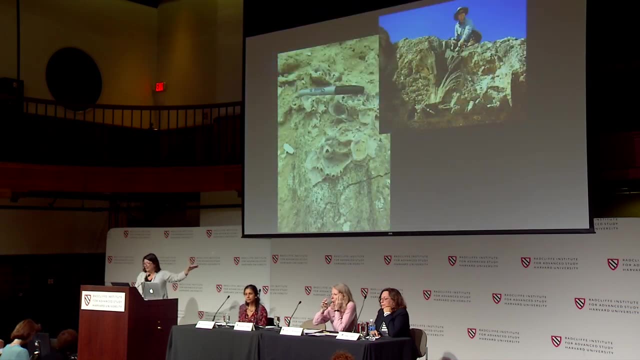 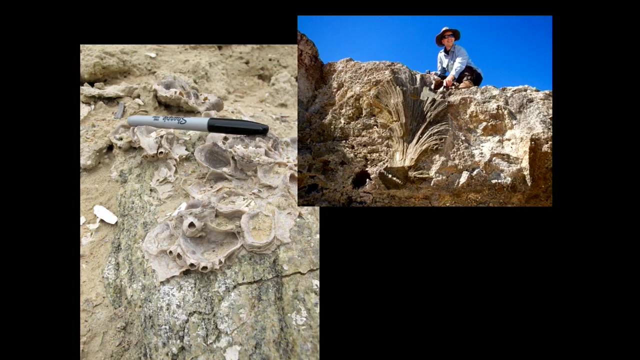 Australia. we are standing on a stranded fossilized reef that is probably about 400,000 years old, from a time period that was slightly warmer than today. This is a reef. This is a fossilized coral. It's my student, Mike Sandstrom, from the Cape. 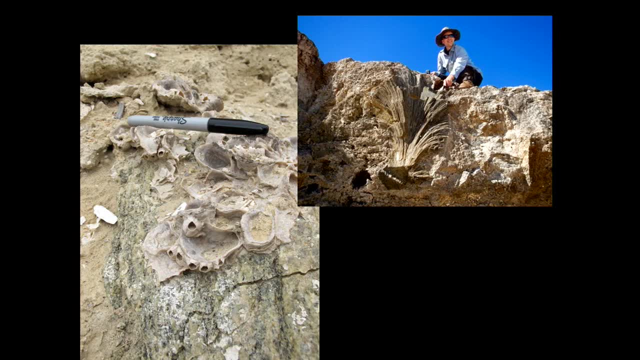 Ranges of Western Australia. That's from the last interglacial warm period, 125,000 years ago. It's a few meters above present day sea level. This is from a 3 million-year-old deposit in Pliocene, the Pliocene warm period in Africa. 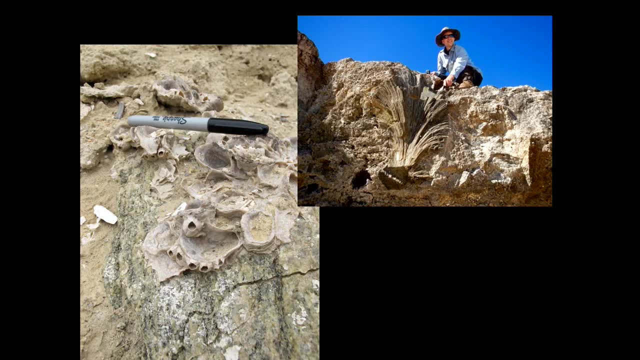 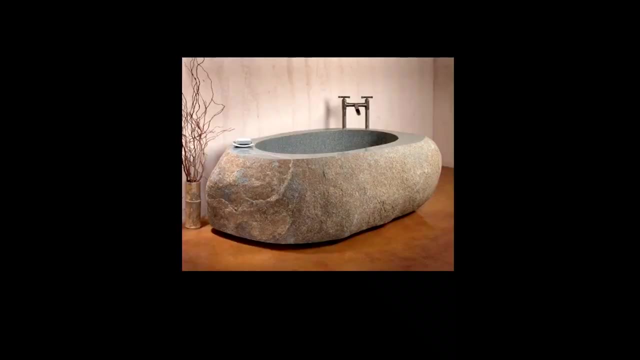 No coral, but we have fossil oysters with fossil barnacles still on the fossil oysters. I mean, whew, you're at sea level. But why is it difficult? We see this evidence for high sea levels everywhere. The major reason it's difficult is because the ocean 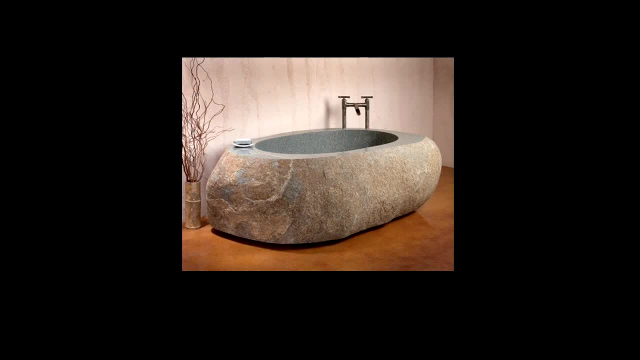 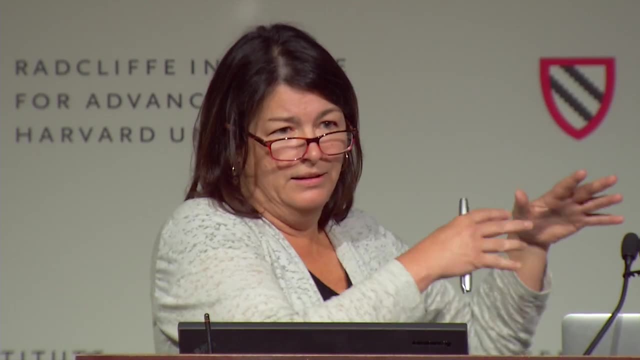 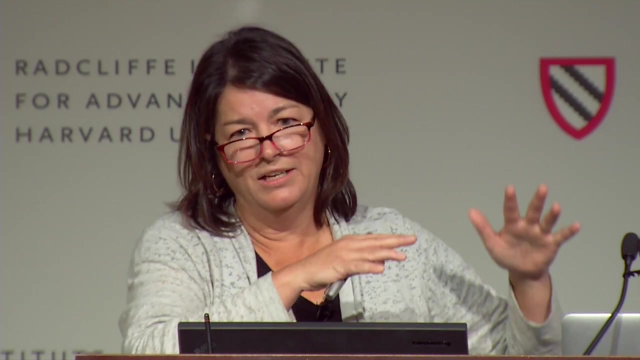 unfortunately, the ocean basin is not like this tub. We can't just look at these as oh like bathtub rings from the past, The continents, the crust of the seafloor and the land. they're constantly in motion. They're being loaded and unloaded by ice sheets. 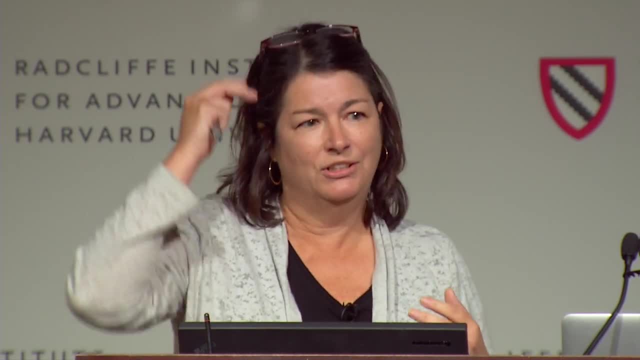 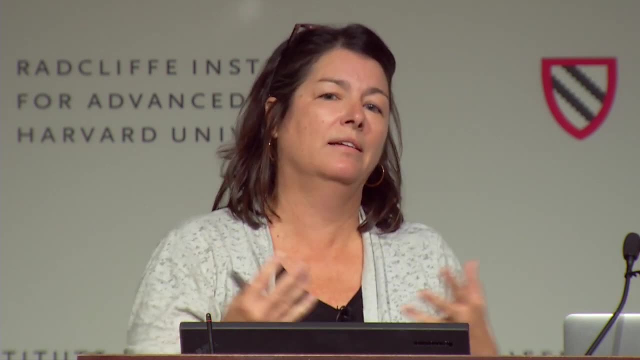 by water. It's constantly moving, So it's quite a challenging problem, And there's a fantastic group here at Harvard led by Jerry Mitrovica that's been working on this, And many clever scientists around the room have made huge progress in unraveling these challenges. 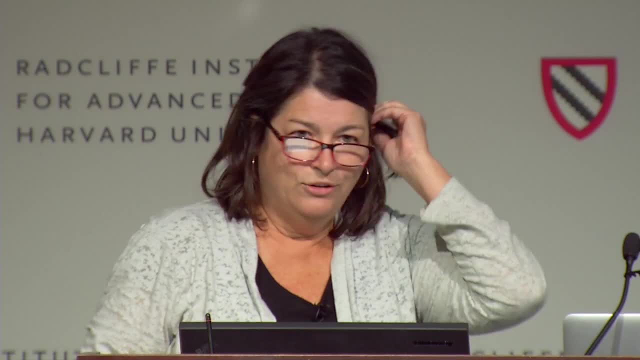 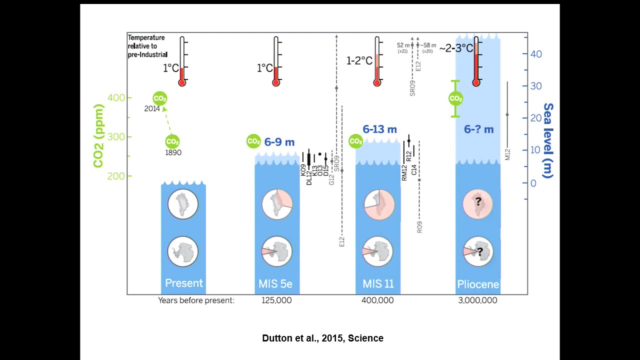 over the last five to 10 years. So I'll jump right to a summary slide which is in a paper we published in Science last year. And so here's- and this is kind of a complicated slide, but it's really cool too. 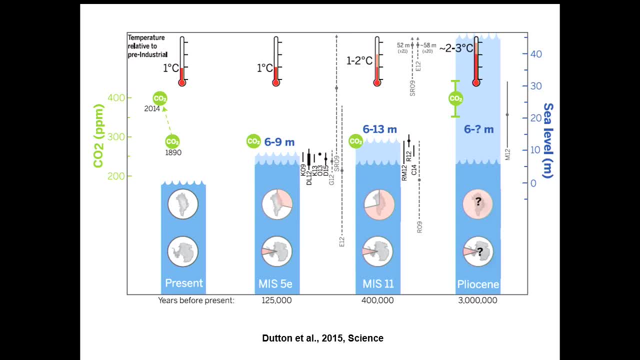 So here's a CO2 scale. There's pre-industrial CO2.. Here's present-day CO2.. And here's a sea level scale. And here's today's ice volume: one degree warmer than pre-industrial right now. Here's 125,000 years ago. 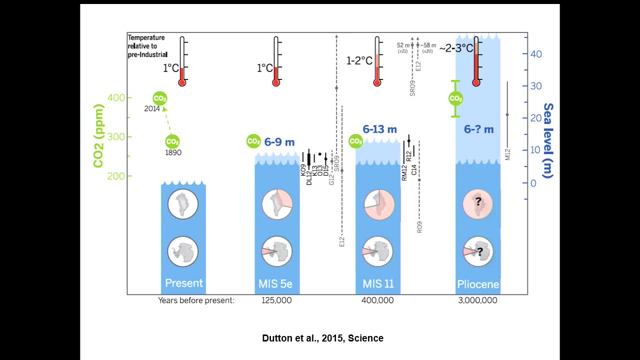 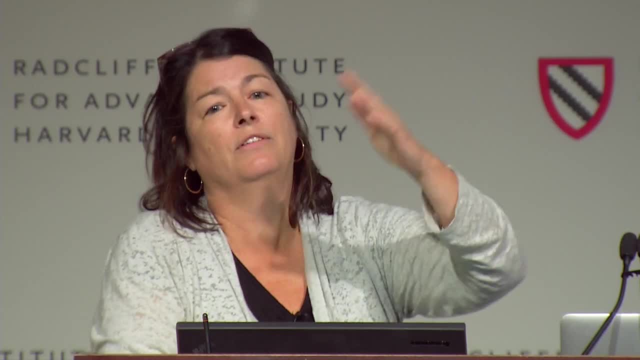 The CO2 was the same during 1921. During that warm period, But we were just so slightly closer to the sun, it was warmer. It was about one degree warmer, a smidge, because of the precession, of the Earth varied. 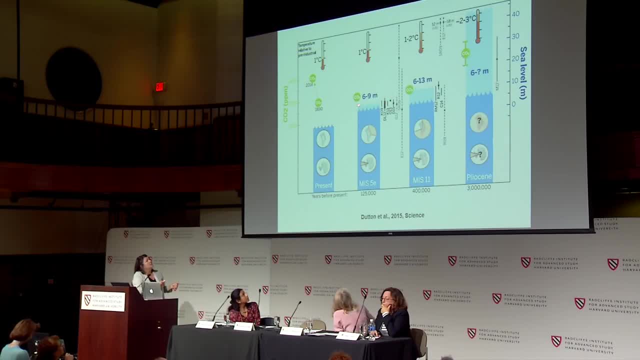 And all these different studies estimate. the estimate of all these different studies is the sea level is six to nine meters higher than today. So this is a window of time that's 10,000 years long. 400,000 years ago it was a little bit warmer. 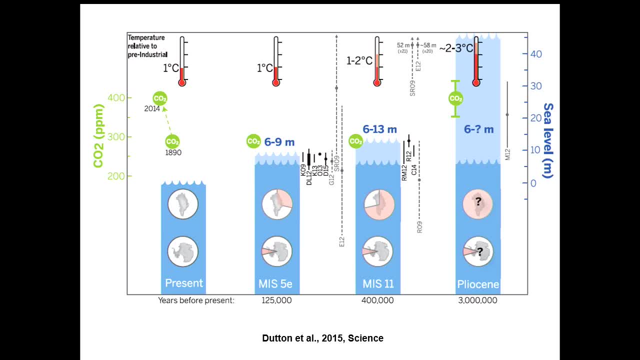 six to 13 meters, Best estimate, And then in the Pliocene. it's been so long, The continents have moved so much. We have a very hard time, Huge error bars. We don't really know But two to three degrees warmer. 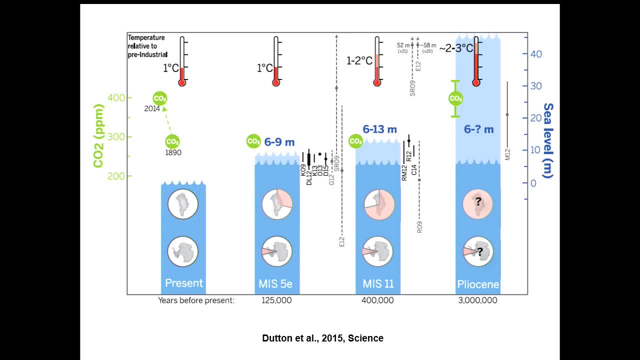 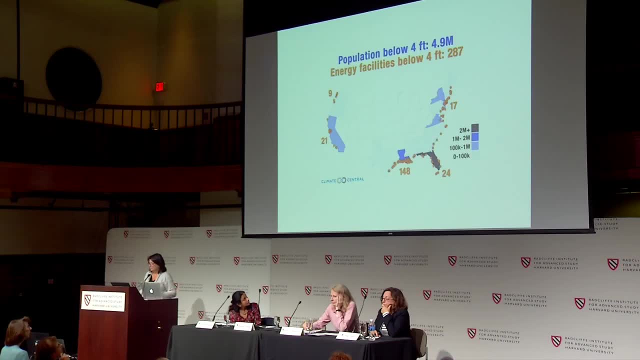 Higher CO2, 400, same as today, And I wish I could tell you more exactly what sea level was at that time. I can't, Okay. so this is six meters 20 feet. Let's take it back to just four feet. 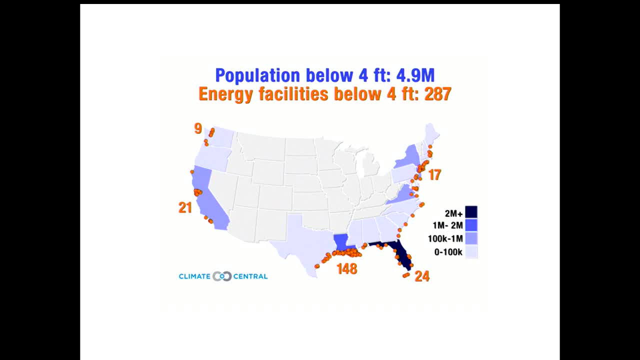 which is completely within the realm of what could happen by the end of this century. I'm perfectly comfortable with this as a prediction. I'm sure there are others that are as well. So four feet above present, that's five million people live within four feet. 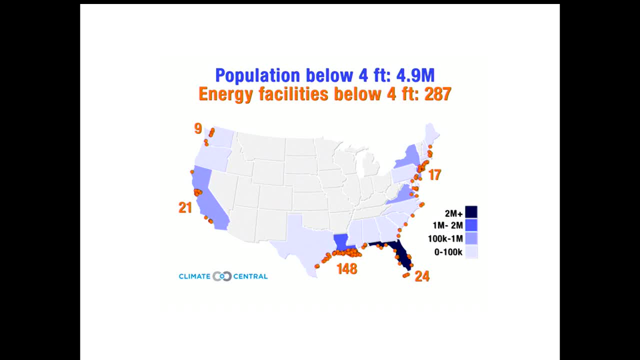 of sea level in the US today. It's a huge amount in Florida, obviously, And in terms of our national infrastructure- energy facilities, ports, naval bases, there's a huge amount of real estate which is in this zone of risk. 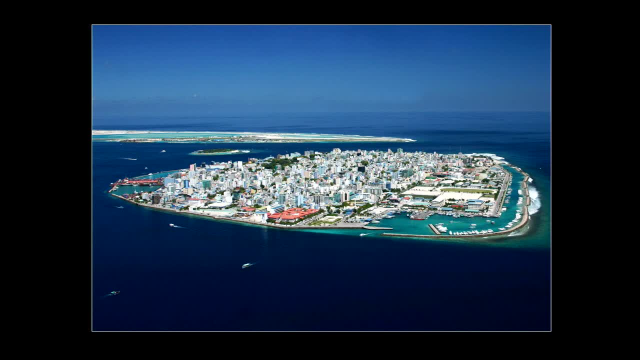 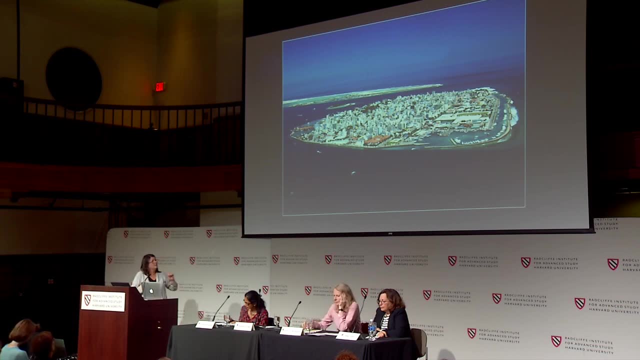 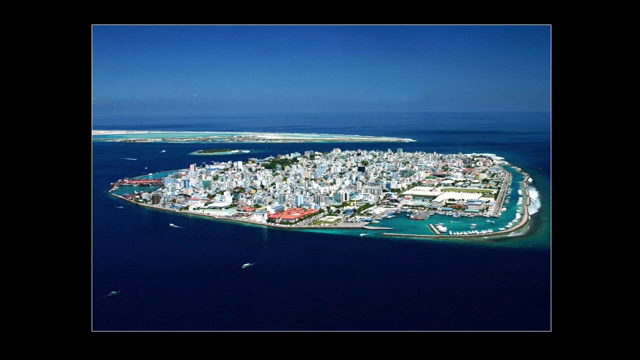 Obviously, sea level rise is not just a problem of the United States. it's a global problem, And we may be hearing more about the Marshall Islands later too. Does anyone recognize this capital city? It's Mali. it's capital of the Maldives. 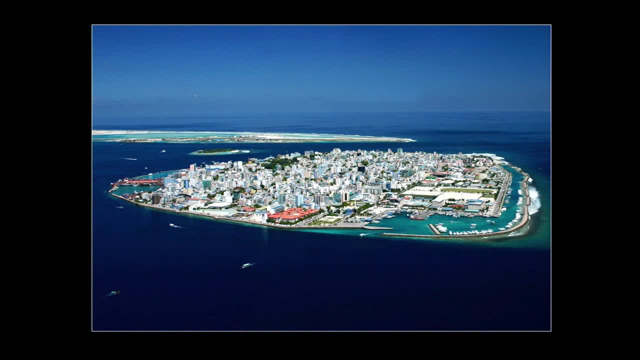 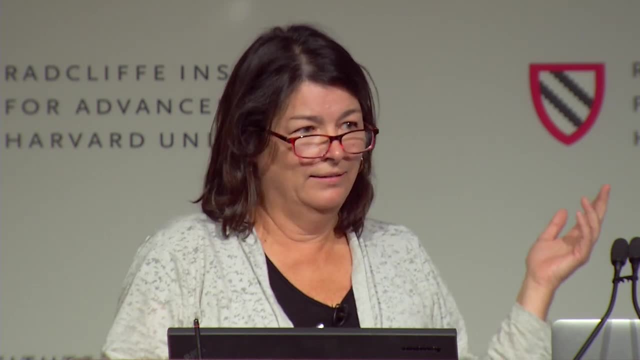 And so you have over 300,000 people living on an island that's a meter and a half above sea level, And this is just one of thousands and thousands of inhabited islands around the world. And when you hear the expression climate refugees, this is what these are: people just like us. 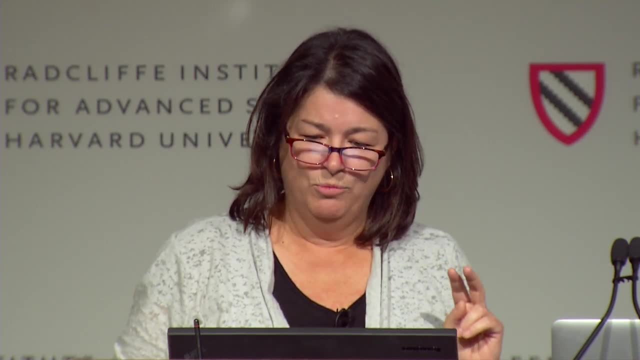 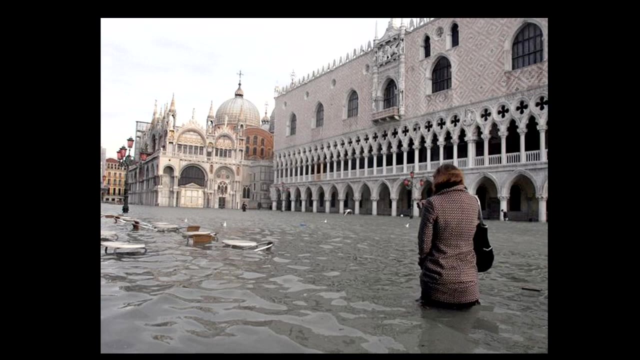 that you're hearing about. okay, So I'm gonna leave two more possibly depressing thoughts about sea level rise, And that is first of all. I think a lot of people have this vague idea they'll be able to deal with it like keep it back. 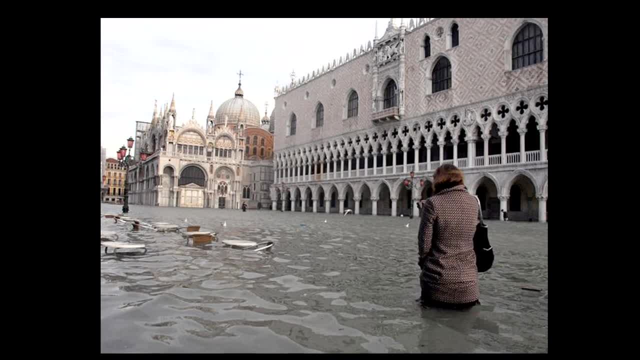 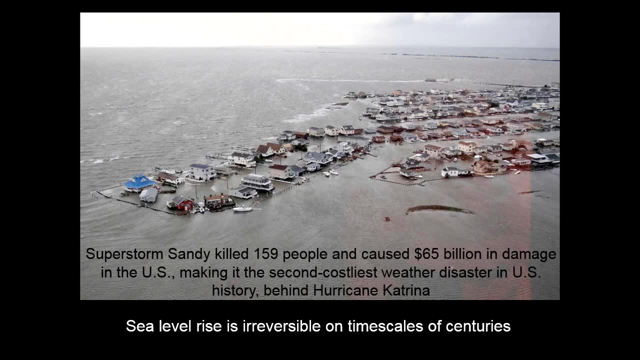 I don't believe that's very realistic, just based on my observations and various places I love. And the other thing that's really important, I think, for people to come to grips with and tell themselves is that sea level rise is irreversible on the timescale of centuries. 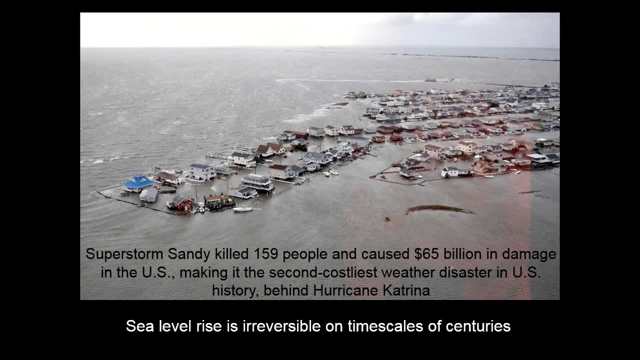 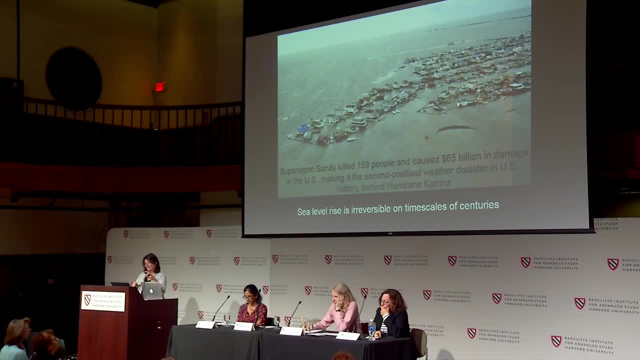 There's. you know you could probably cool the earth- it's atmosphere- easier than you can regrow an ice sheet. So every year, the increment of water that's going in from the melting of polar ice sheets and the thermal expansion of sea water, 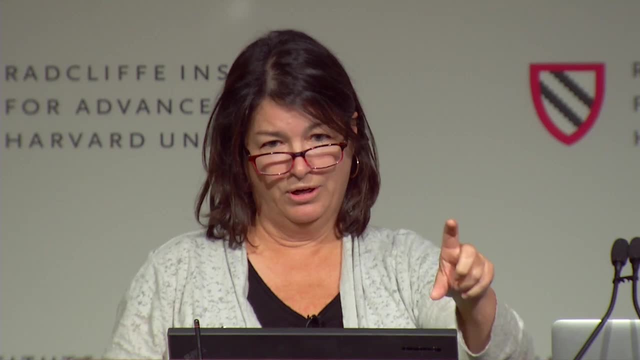 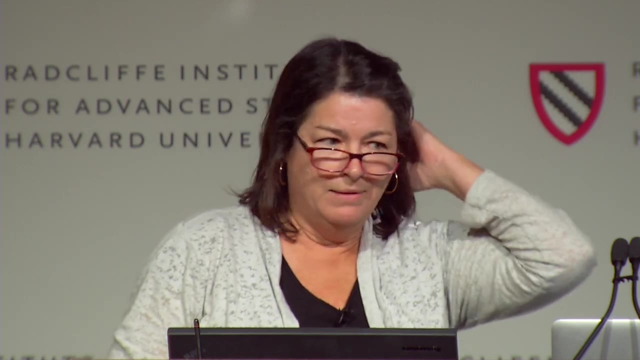 that's an increment of sea, of sea level rise. It's there and that we're gonna have to deal with for centuries to come. So to wrap that up, what I know for sure: climate is changing naturally all the time. Small variations, very small variations. 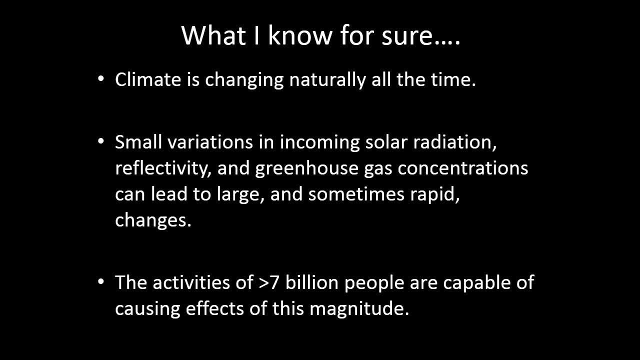 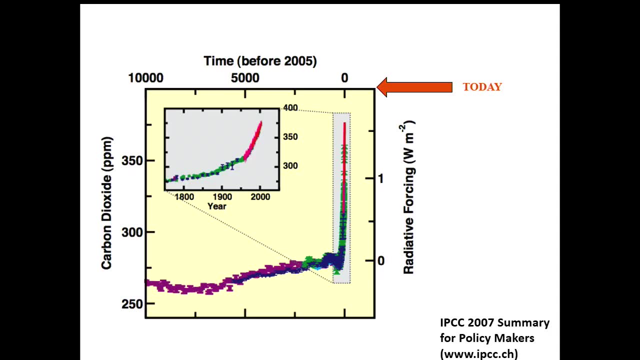 in incoming solar radiation, albedo reflectivity and greenhouse gas concentrations can lead to. some can lead to large and sometimes rapid changes. The activities of seven billion people are capable of causing effects of this magnitude, And here's a CO2, carbon dioxide record. 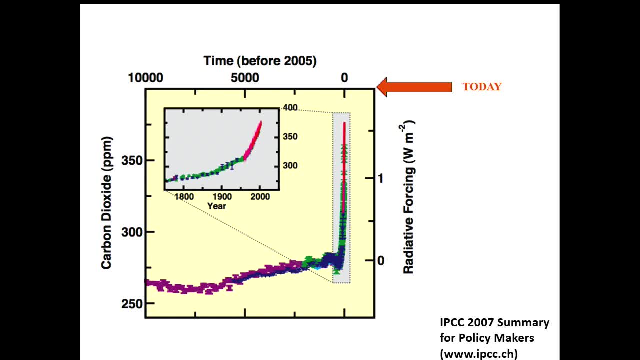 of the last 10,000 years, The Holocene, the warm window of time within which human culture, agriculture, flourished. It was about 270 parts per million. A subtle rise starts about 5,000 years ago. Many scientists believe this is due. 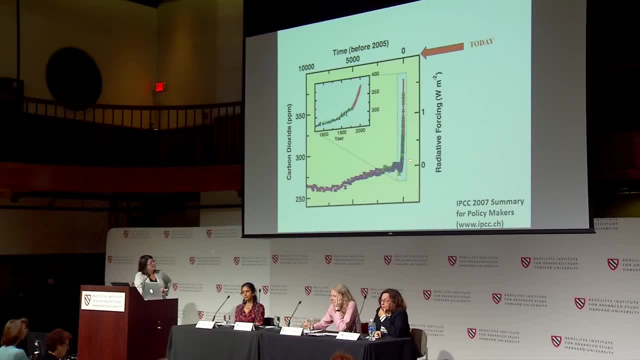 to early agricultural deforestation. And then here, this interval, right here, blown up right here, Here's the 18th century, the beginning of the industrial revolution, And this rise is the addition of CO2 to the atmosphere from the combustion of fossil fuels. 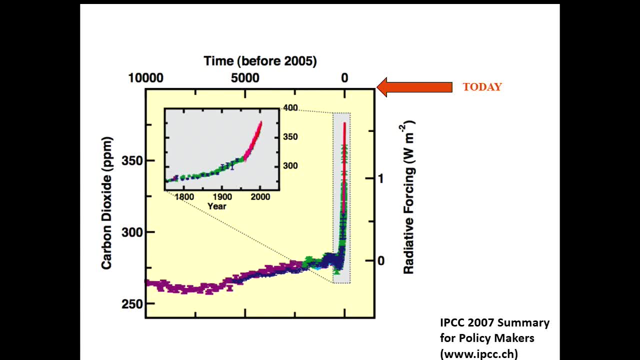 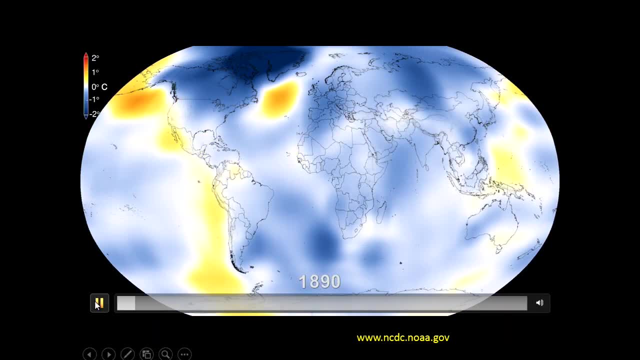 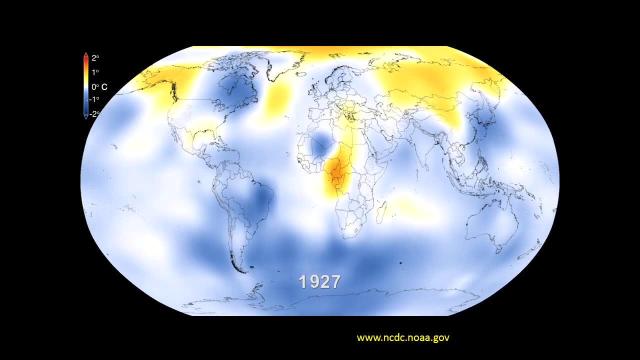 And obviously this is out of date. We're already over 400 ppm. I have another video here. There it is. So this is what that CO2 has done in a very nice visual. We humans have cranked the knob. They've taken the CO2 dioxide. 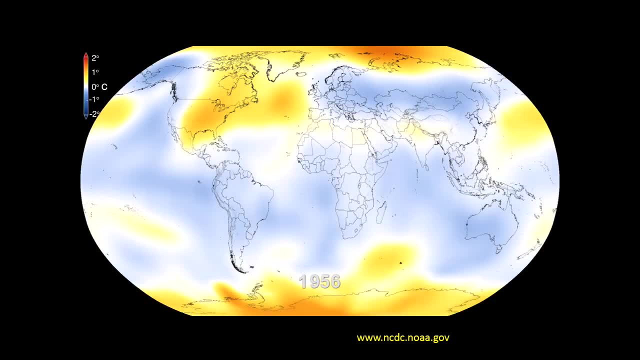 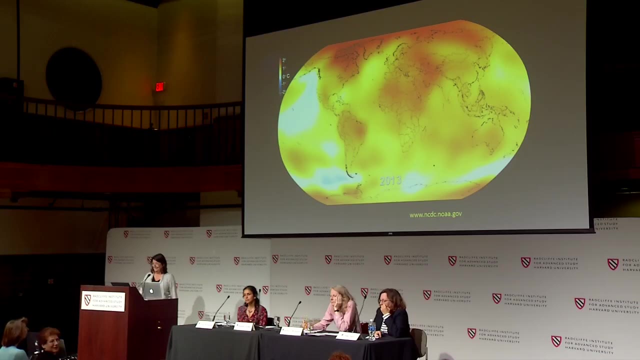 and they've turned it hard to the right, very hard. This is a temperature. this is a surface temperature anomaly map based on instrumental data from around the world. Want to see that one again? Yeah, Okay, that's cool. So what you're looking at is the mean is defined as 1951 to 1980.. 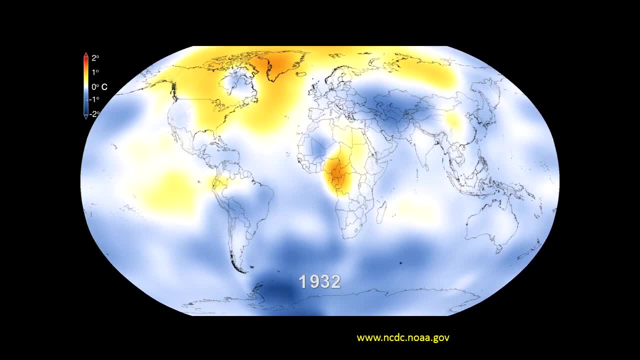 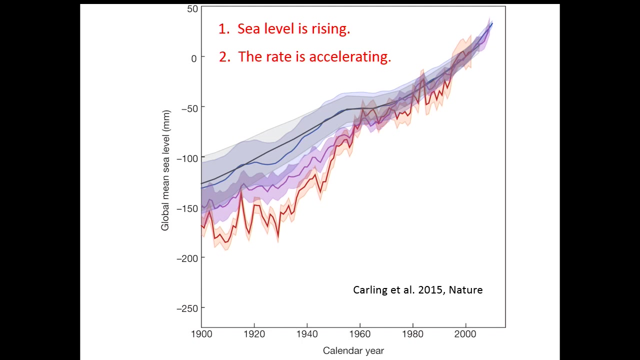 And so what you're looking at is every surface anomaly relative to that mean. So the beginning's generally lower than the mean And, as you see, when you get towards the end you're generally hotter than the mean, In partnership with that warming atmosphere. 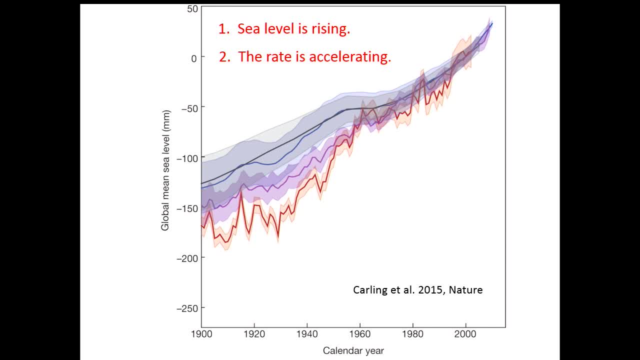 heat penetrating the ice sheets, heat penetrating the ocean, causing thermal expansion of the oceans and melting of the ice sheets. Sea level's been rising. These are various different studies based on different techniques, including tide gauges and they you know. 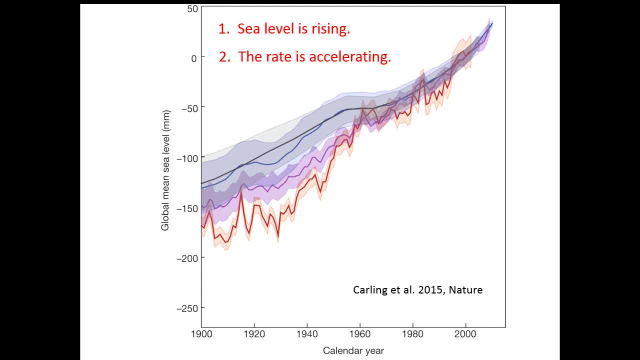 they're in more disagreement the further back in time you go. But I think the what everybody is in agreement about is that sea level is rising and the rate is accelerating. This is from a post-doc at Harvard, Carling Hay, And just to take this time window, 1900 to 2000,. 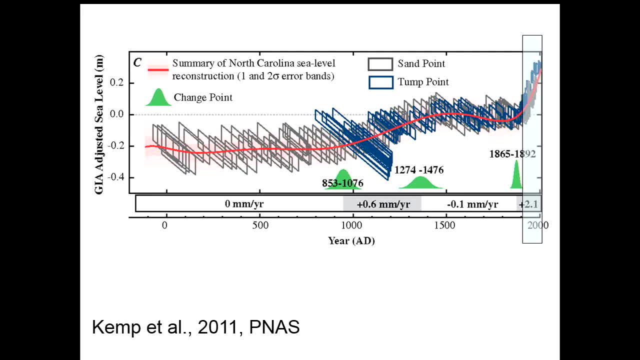 and put it on the a time scale of the last 2000 years. right, it's all about perspective. right, Here's that same curve. You would put it right here. So, natural variability, the rise in sea level due. 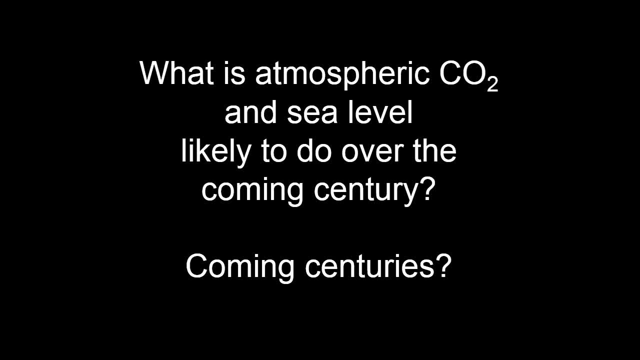 to human induced global warming. So what is the? I'll just wrap up here one more slide. What is the atmospheric CO2 in sea level likely to do over the coming century, And of course it's not just the next 100 years? 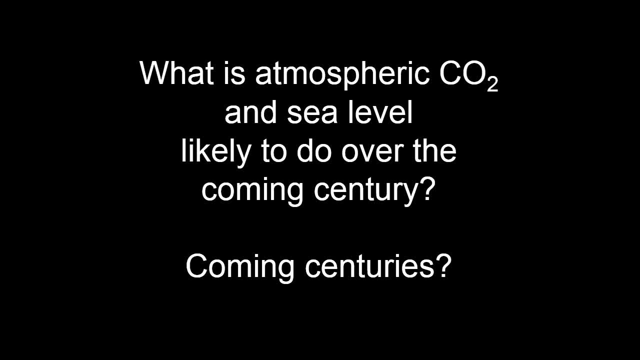 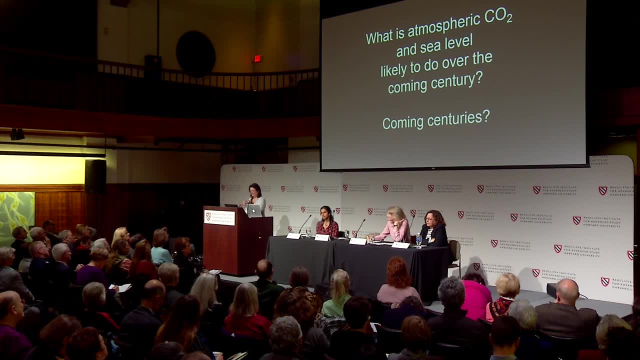 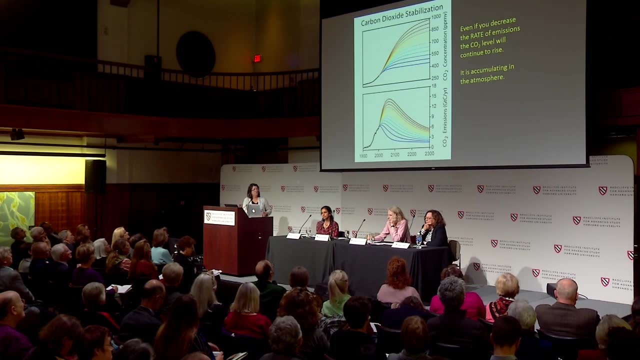 it's many hundreds of years into the future. This is not a scientific question that scientific scientists can answer. This is a question that's going to be completely dependent on the individual and collective actions of citizens and their governments. But I will say that, if you look at this, 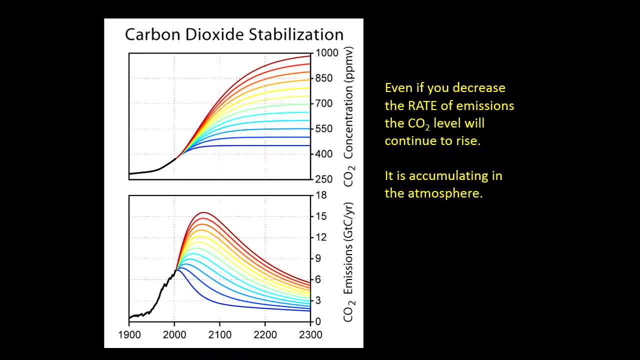 here is our current CO2 emission rates, And what this is showing is these are the paths that you know, as a planet, we have to choose to be on. Can we turn around global CO2 emission rates quickly, or is it going to take longer? 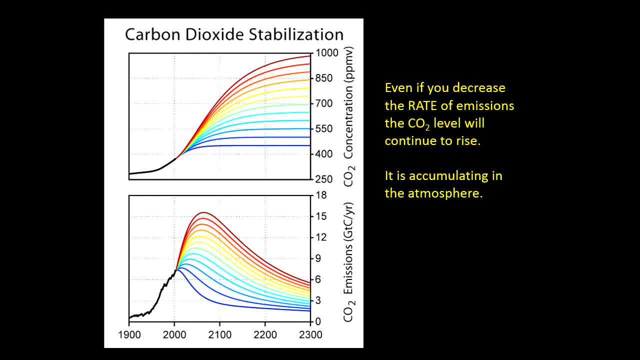 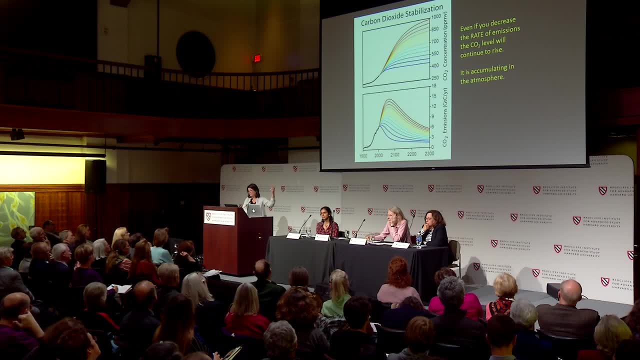 And the point to make here is: even if you turned it around today, You're still putting CO2 into the atmosphere. Much of it's going into the ocean, but most of it stays in the atmosphere and it will stay there for hundreds of years. 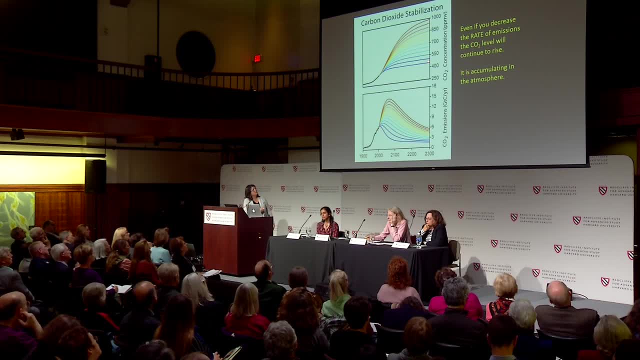 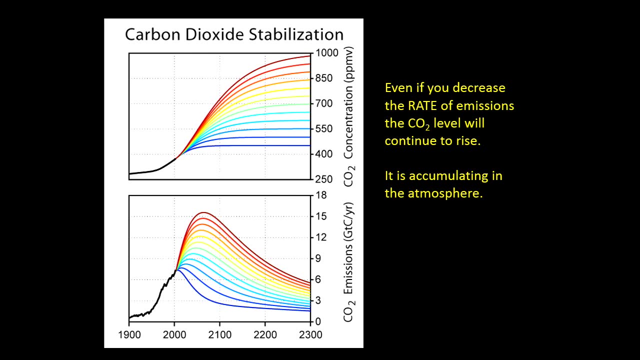 So, even if you turn it around, today, you're committing yourself to CO2 levels up around 500 parts per million Every decade. you put it off, you commit yourself to higher and higher sea levels down the road. So, as someone who knows what these changes in sea level have done, 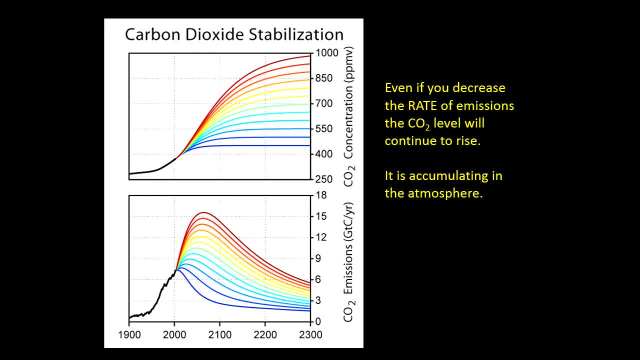 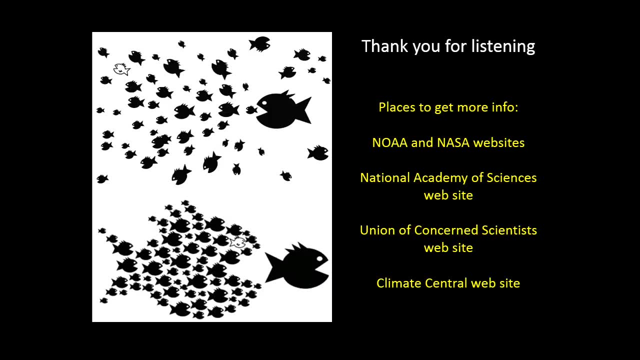 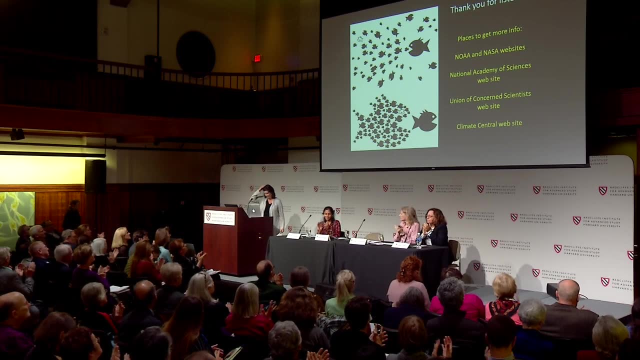 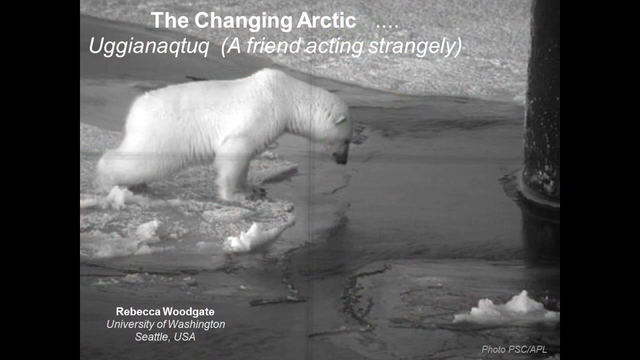 sorry these changes in CO2 have done in the past. you know this would be of great concern. Okay, so I'll just thank you for listening and happy to take questions later. Well, good morning. I'm from the University of Washington, Seattle. 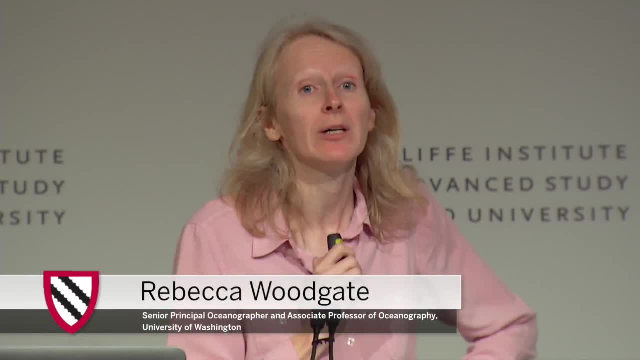 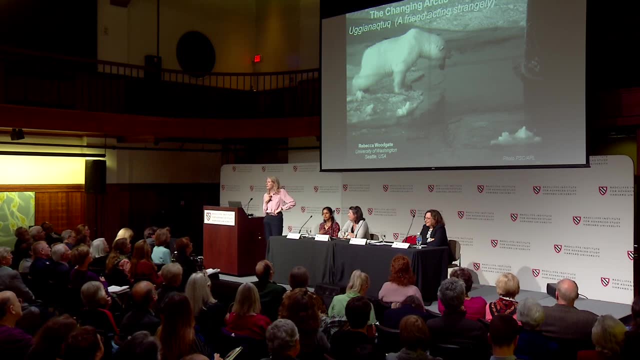 And for the next 20 minutes I would like to take you up to the top of the world. Please join me in a moment of silence, Thank you, I'm going to be, And you know, the thing I've always liked about the Arctic. 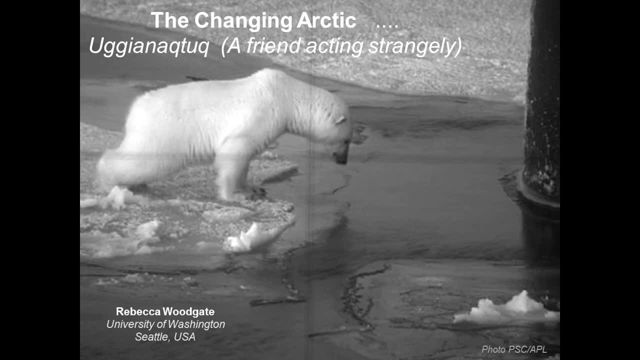 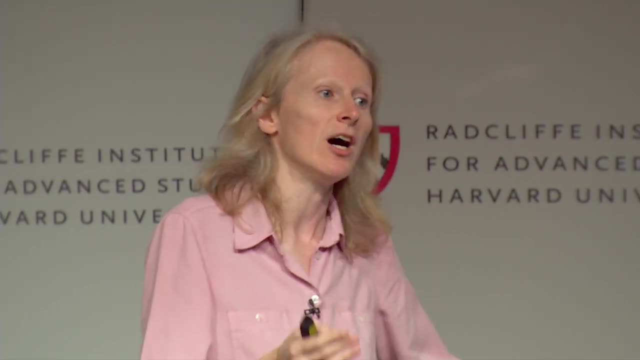 is that when people appear into the Arctic, like this polar bear is appearing into her Arctic in her case- she sees a submarine come up to her, something she doesn't understand. probably There are things about the Arctic we do and do not understand. 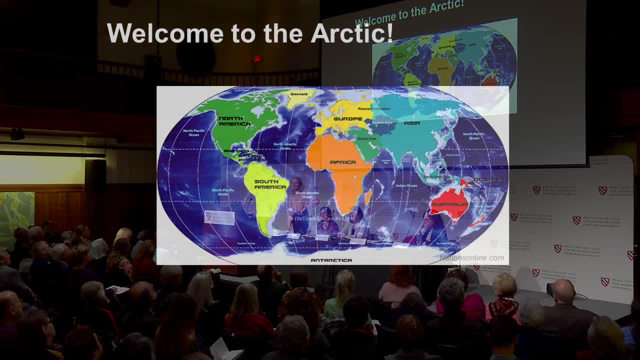 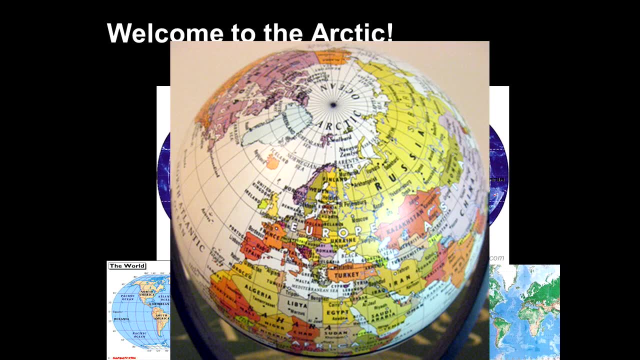 This word here, ugnianuktuq. it's an Inuit word. It means a friend acting strangely off a lot of maps. Here it is at the top of these maps. It turns up squashed into a little layer at the top. But if you take a globe and you peer down from the top of it, you 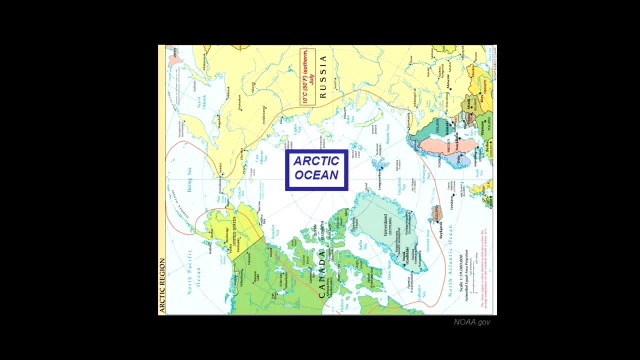 can see there's a proper ocean up there. I'm going to twist this map round, because it is usual when you're talking about the Arctic to put the country you're talking in at the bottom. Lots of countries here, lots of countries vying for owning the Arctic. This picture. 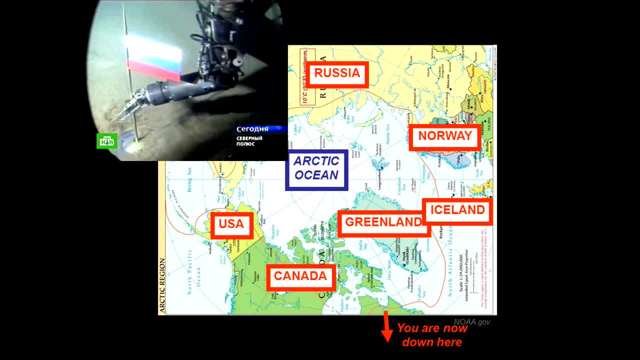 anyone know this picture? This is the Russians putting their flag at the North Pole, three miles down under the ocean, in 2007, saying it's theirs. We're not going to go there today, but there's interesting debates about that. To give you some idea of scale, this is relative. 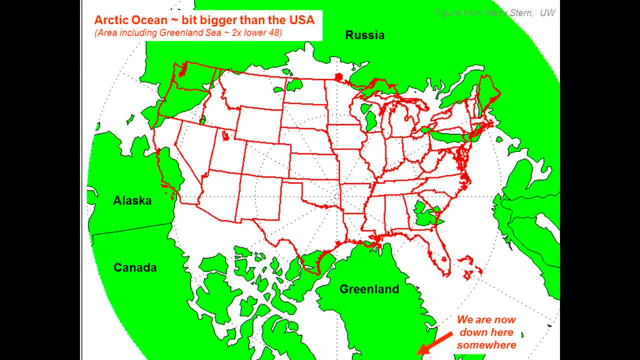 to something I hope you recognize: It's bigger than the US. If you want some numbers, here's some numbers on it. It's the smallest of the world's five major oceans, but it's famous in many, many ways, even before the changes of recent days. 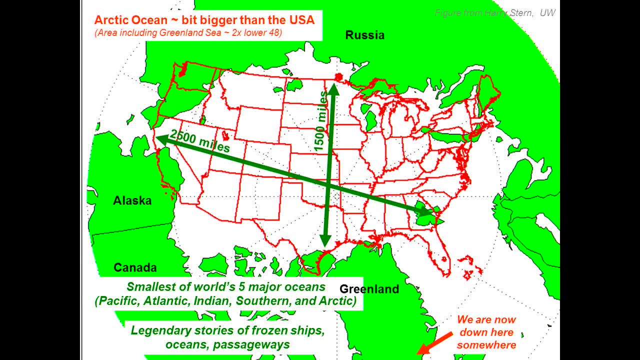 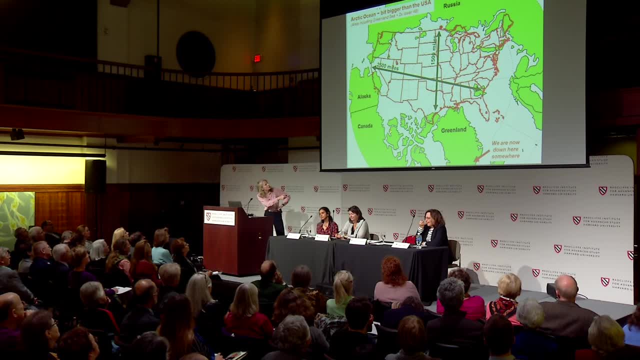 For frozen ships, for passageways for the North Pole, etc. Perhaps one of the most poignant is the Northwest Passage, which is this route between the Atlantic Ocean, which is down here, and the Arctic. the search for the Northwest Passage, And let's start there, 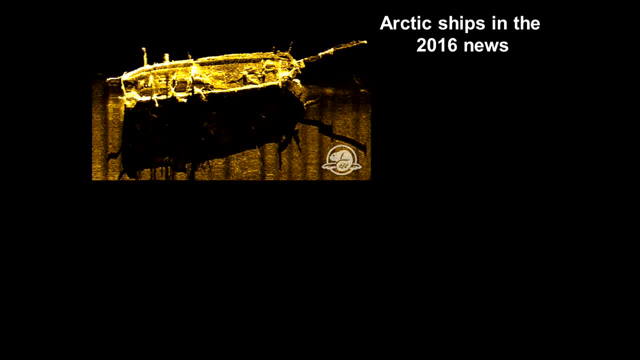 Let's start with some recent Arctic ships. Can anyone tell me what this is? This is the wreck of the HMS Terror. This was one of the ships which set sail from England in 1850, 1845, looking for the Northwest Passage, The Franklin expedition, the lost Franklin. 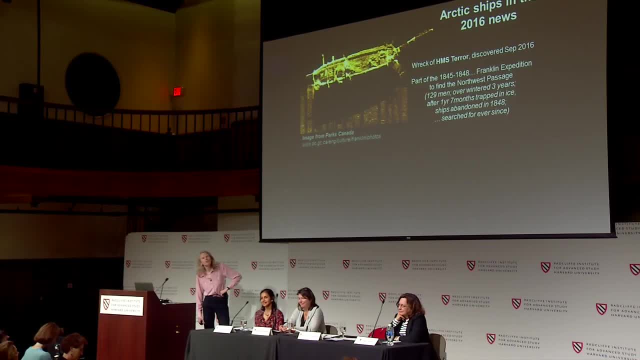 expedition. It's not a happy story. They overwintered three years in the archipelago trying to find a way through. After more than one and a half years stuck in the ice, they left the ship trying to walk south and none of them survived, And since then we've been 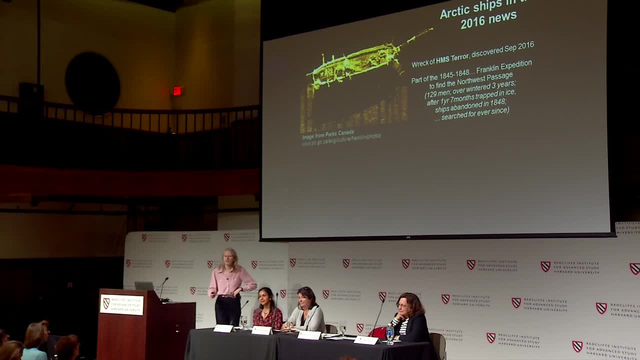 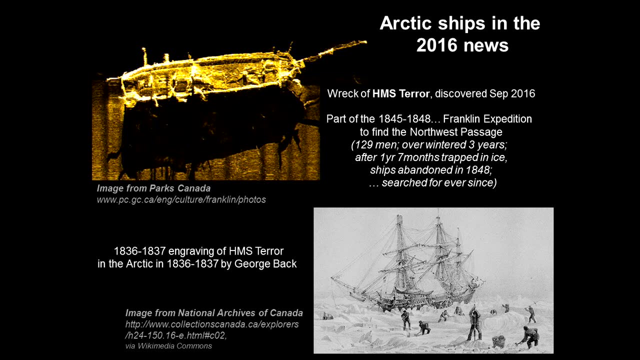 looking for those ships. We found those ships in the last year. I say we- this is Parks Canada. The Canadians put a lot of effort into doing this. This is the ship on happier days some years before this, 1836.. Getting stuck in the sea. 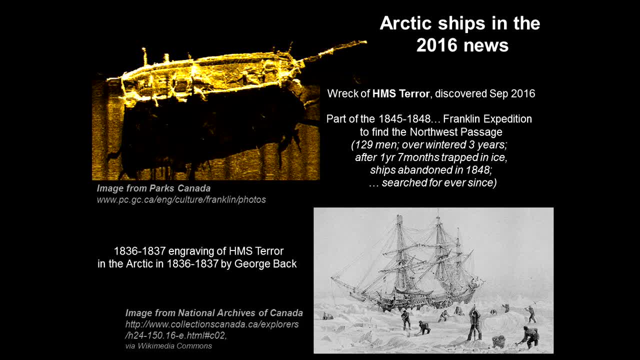 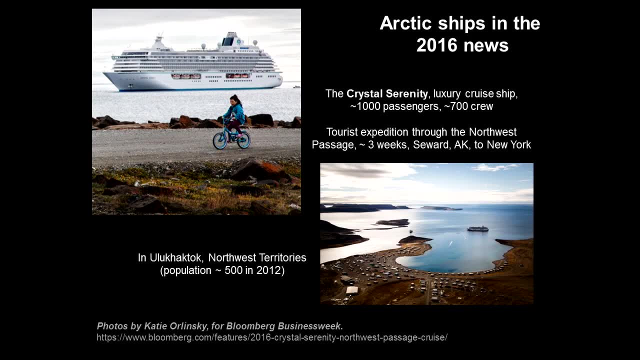 ice was an occupational hazard of being an Arctic explorer in those days. So another ship in the news this summer. Anyone know this one. This is the Crystal Serenity, a luxury cruise liner, 1,000 passengers, 700 crew, which had just gone through the same. 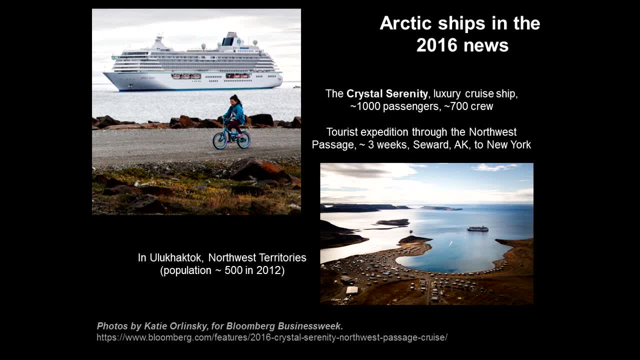 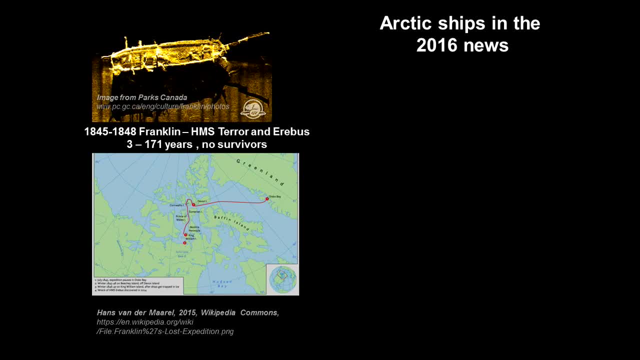 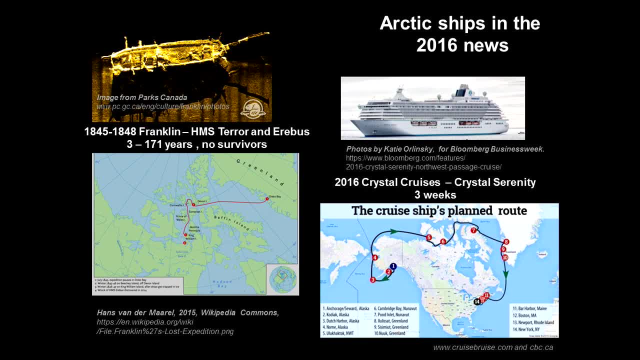 they see the whole crew perish, Nobody came home. And the Crystal Serenity, which has gone through a nice planned trip of three weeks, come out in New York. What's the difference? The difference between this is ice, Let's talk about ice. So if I take sea water and 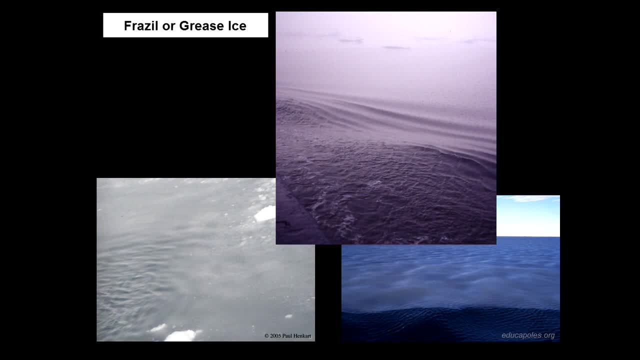 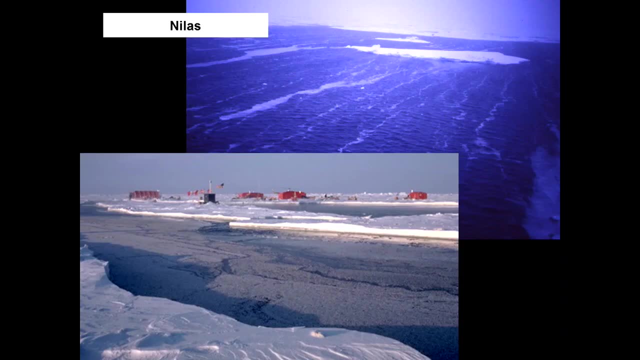 freeze it, I start to get very little crystals. They float up to the surface of the ocean, form a kind of a oily layer on the top of the ocean which gradually pushes together to form a sheet of ice. okay, this is has some resilience. I wouldn't. 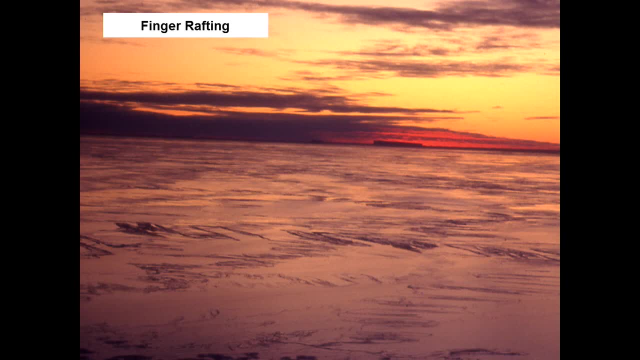 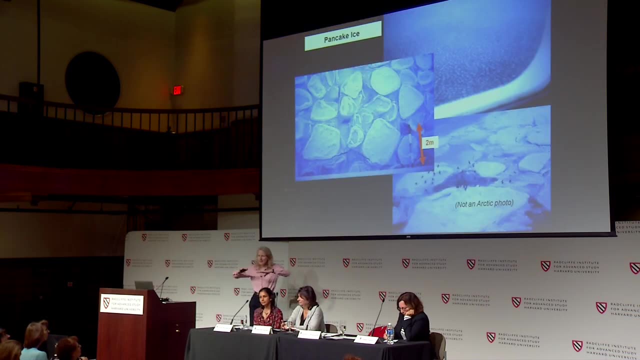 walk on this at this stage, but it'll push together and you can see the edges. you can see here the striations of the layers push against each other. let it go a bit further and these layers form into more sheets for a penguin. you can walk. 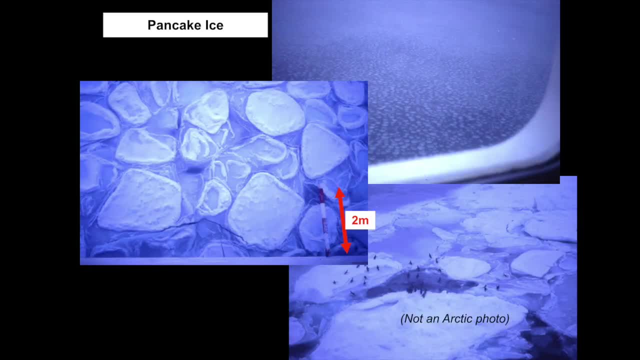 on this. no, there are no penguins in the Arctic. as these sheets come together, we call this pancake ice. people at sea will think of a lot of things, and if we they form, they get thicker and come together or appeared a few more days to make it. 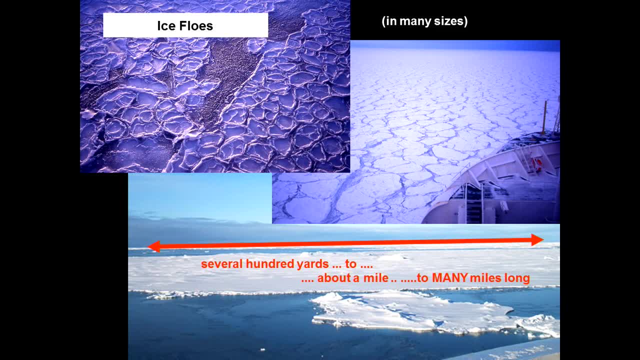 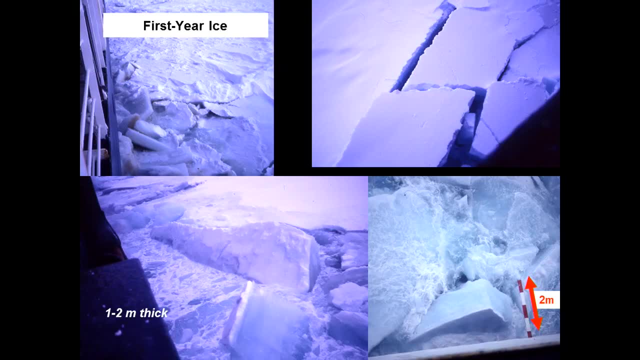 to ice flows. nice flows can be several yards to a mile to several miles across. I don't know how you got here, but this gives you an idea of scale. this is the first time that I would walk on this stuff. this is about one to two meters. 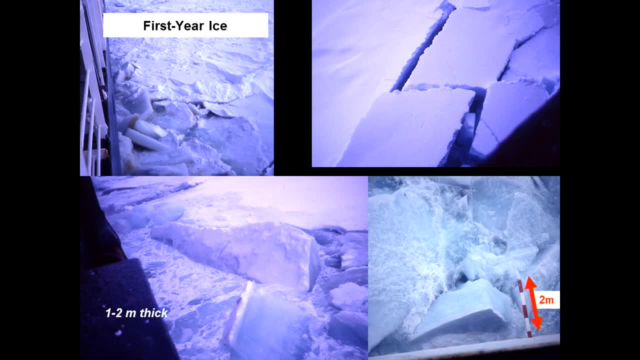 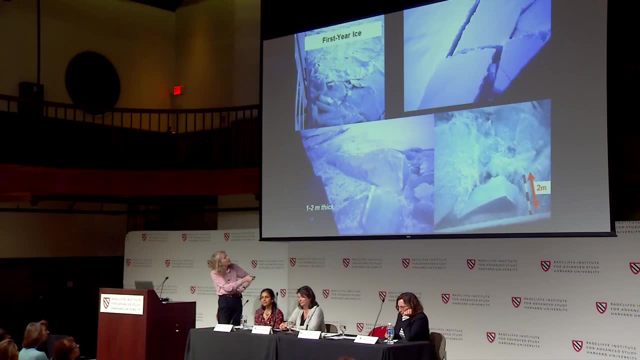 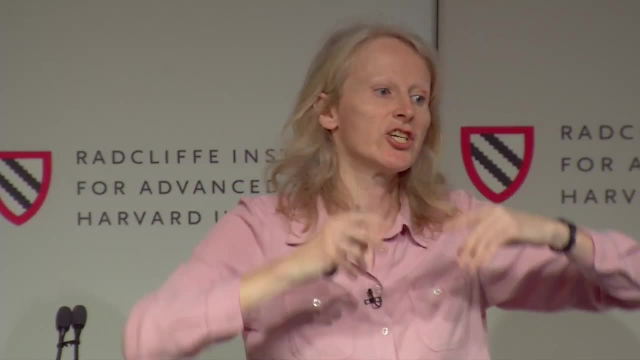 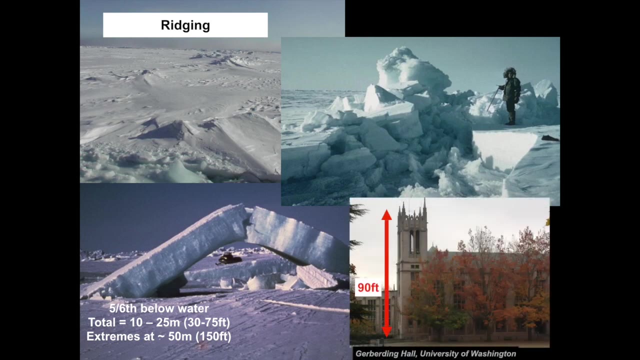 ice pushed together, they've Ridge just like a mountain range or Ridge, and this is what makes our thickest pieces of ice. I put here a picture from one of the pretty buildings from my university and I've got a picture of a building that's 90 feet tall, as this tower, and that is a not a typical height for a ridge. that. 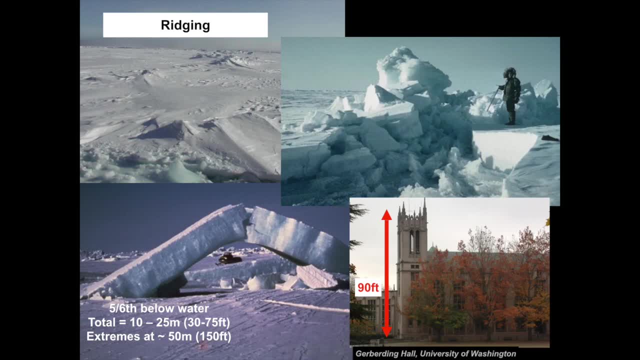 you would get in the Arctic just like an iceberg. there's more below than above. so if we have this chap standing here beside the ice and we measure how far above the water he would be and how far below the keel, you're looking about an ice keel, about the height of that building. so these are common sizes of. 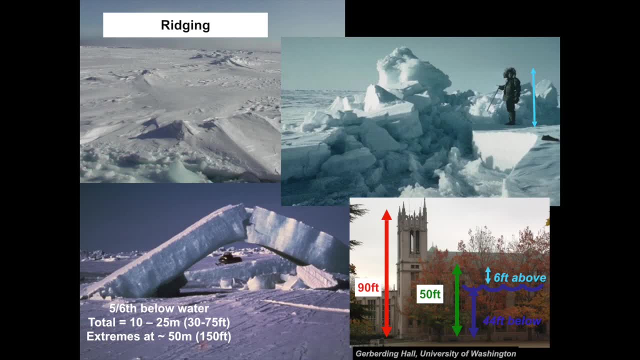 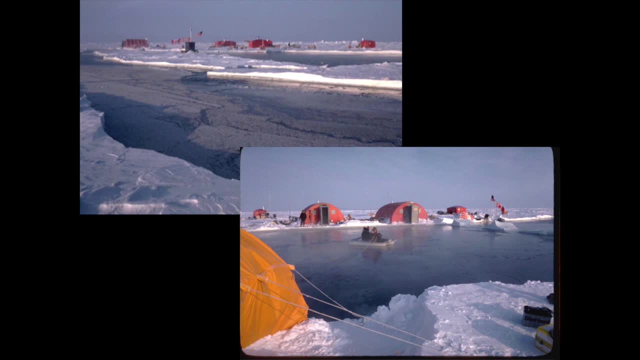 thicknesses of ice in the Arctic. now, while this is pushing together here, it's coming apart somewhere else and this gives us what is called leads in the Arctic, The ice cracks in the ice which can appear overnight very, very quickly, sometimes in inconvenient places. this is a hazard, current hazard of Arctic. 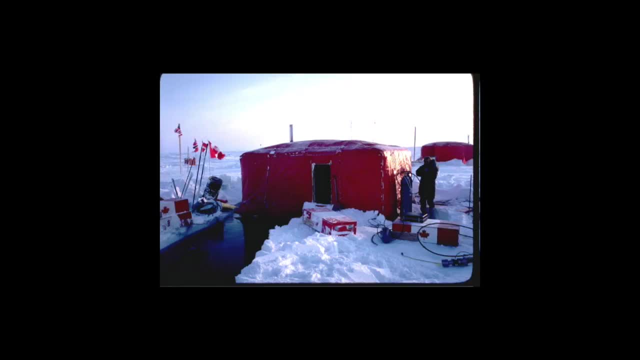 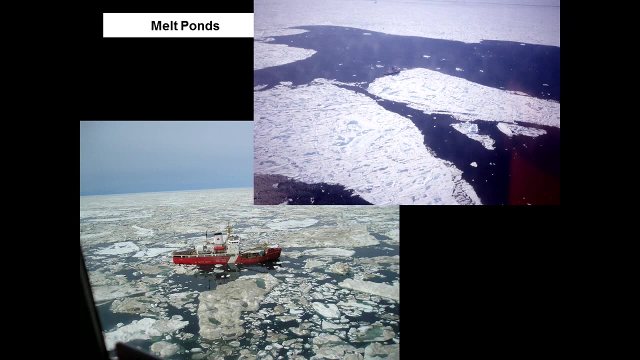 exploration as you might get a lead, come to your camp in the middle of the night with interesting consequences, didn't fall in, we don't really mind. I prefer to work off ships for that reason, and you can see some ships here. here's a ship that's giving the scale of the ice flows as the summer carries on, the Sun melts. 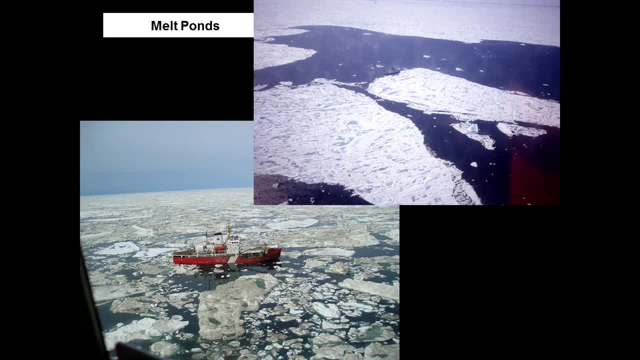 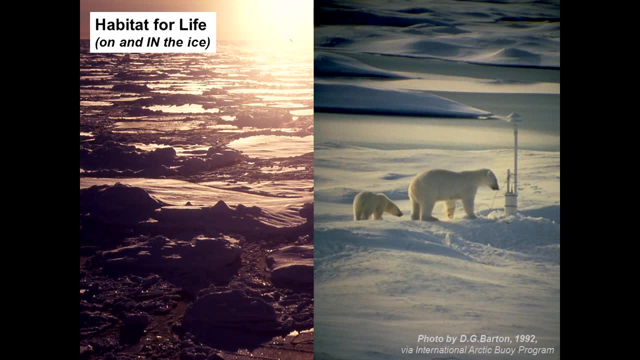 the snow on the top of the ice gives you melt, ponds on the top of the ice and the ice flows which will eventually decay the ice away. it is a habitat, for life is ice. we have our charismatic mega fauna and we have our perhaps not so charismatic tiny. 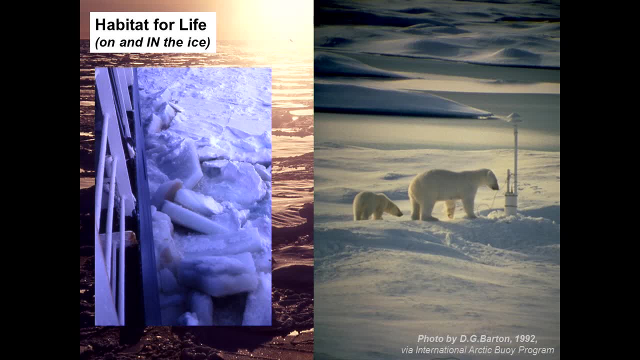 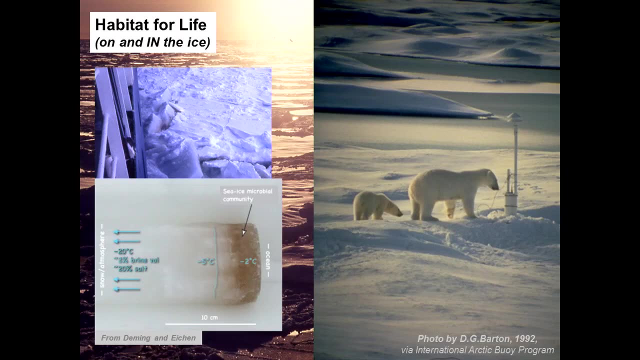 fauna, this little brown striations you see here. that's not mud and that's not paint off the ship. that is actually little ice, microbial community plankton which are growing in the channels of ice. you can do this yourself. go home, take some salty water, chuck it in the freezer and tomorrow morning put drops of food. 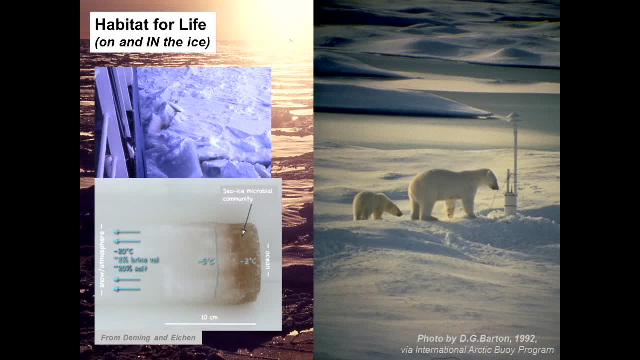 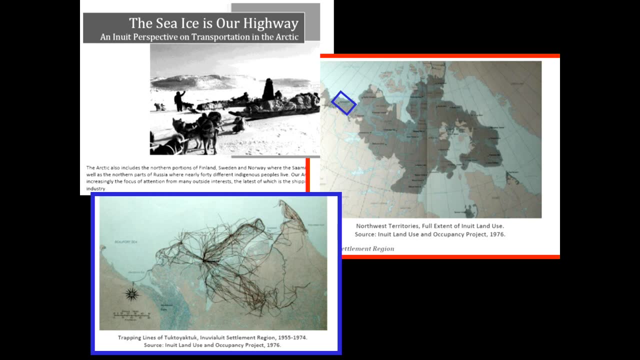 coloring in it and you can see the channels of the ice and you can see the ice that goes through the sea- ice, which are channels for life. it's also home for people. the Inuit have made their history in the Arctic for 10, 10,000 years and to 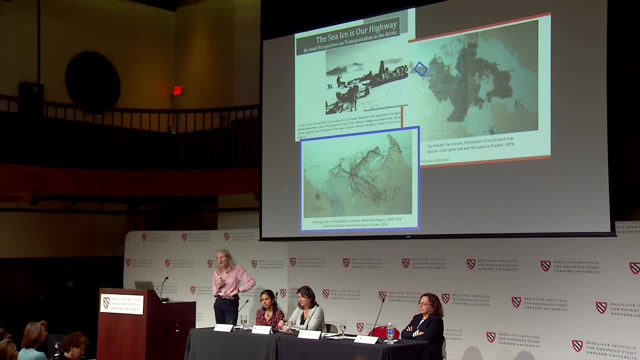 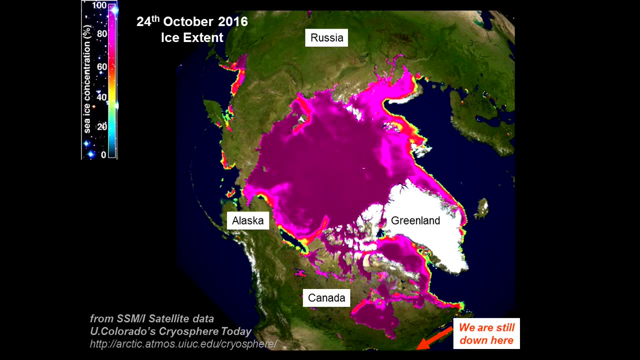 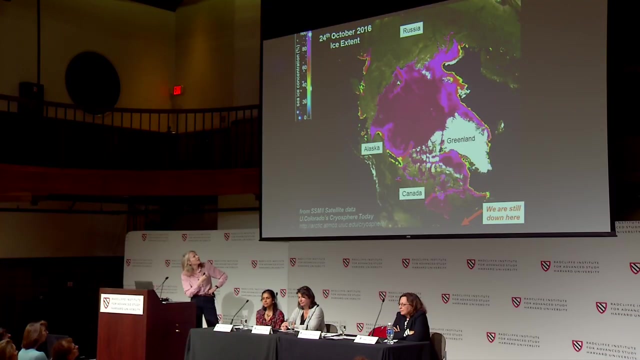 them, ice is not a hindrance. ice is their way of getting around. ice is their highway. so where are we today? this is almost today's sea ice edges. in a satellite image, Greenland's here. the colors give you the ice concentration, these dark areas of water. you can see the sea ice now building up from its. 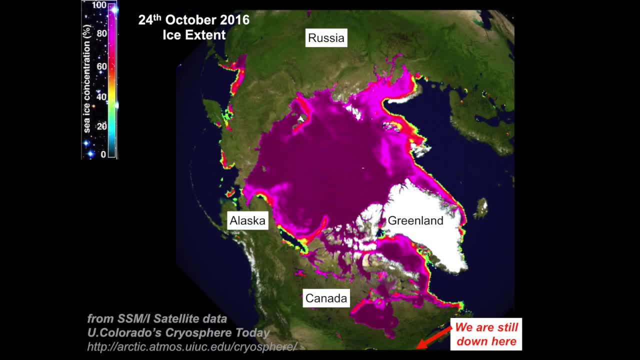 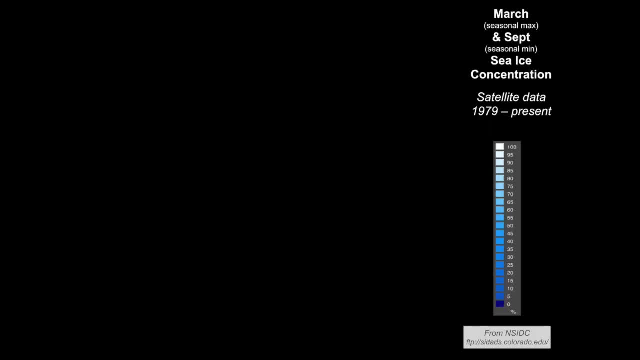 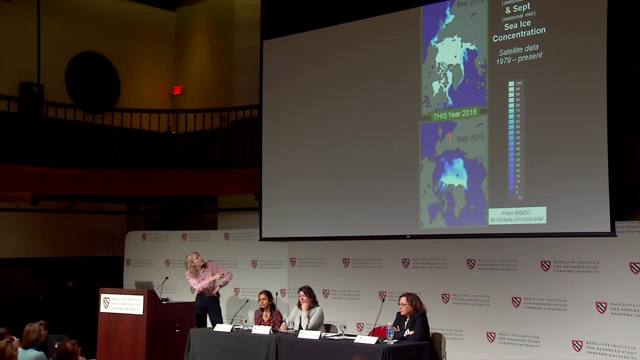 expanding. as the winter has started in the north, it's expanding back out to the coast and down into the lower latitudes. that's a snapshot of today. it's a large seasonal cycle in sea ice. this again satellite data- we're over here again now- showing the maximum extent in winter and the minimum extent in summer: calm March. 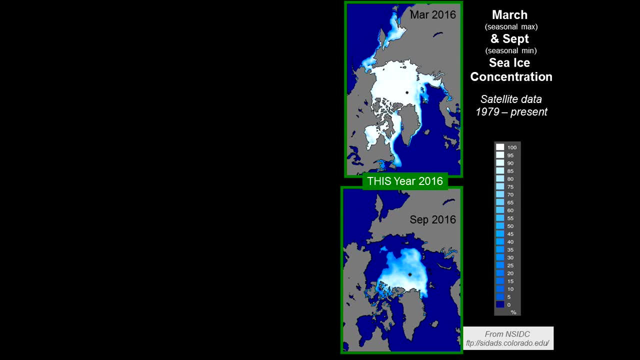 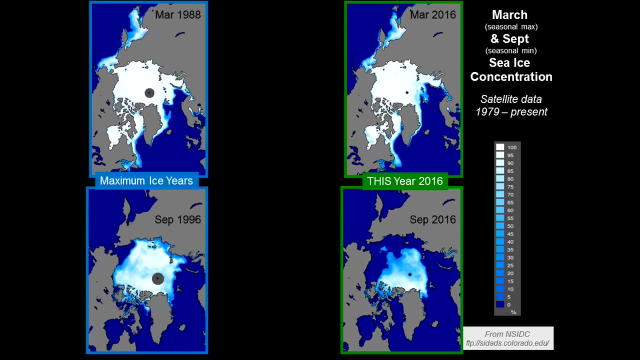 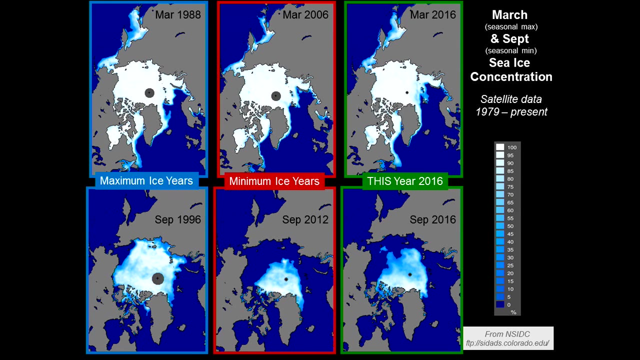 in September respectively. large seasonal change cause because the Sun comes up and melts the ice. well, how does this year compare with the past? we have this satellite data back to 1979, and I pulled out the years which have the maximums in the seasons and the minimums in the seasons and to make it a bit easier to 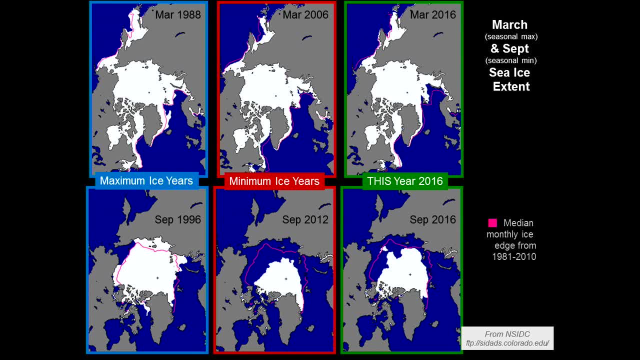 see, I'm going to change it now to sea ice extent. and this pink line in both of these map shows the monthly median edge from 81 to 2010, so what we thought was standard for most of our satellite record. so in the winters, you know, we're. 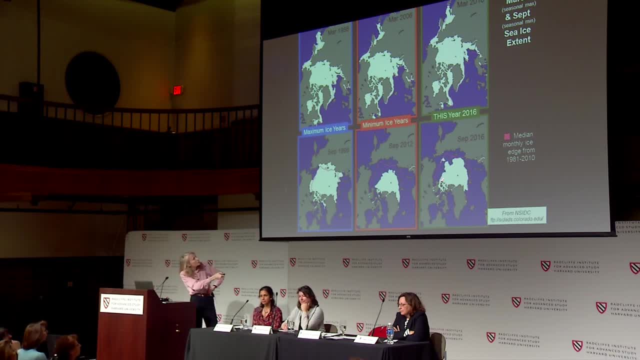 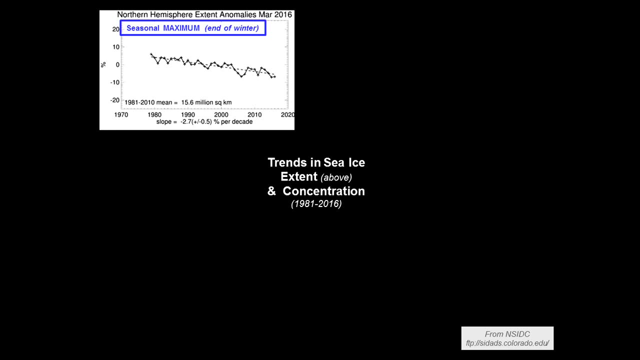 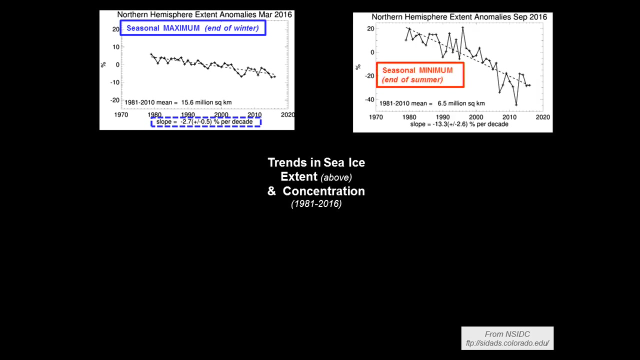 kind of close to that, getting a few changes. but the summers we're seeing this very dramatic loss of sea ice. let's put those on time scales here. we have the whole time series, we have and the trend line through that and it's not very much, it's a few percent per decade. this is the winter, but in the summer 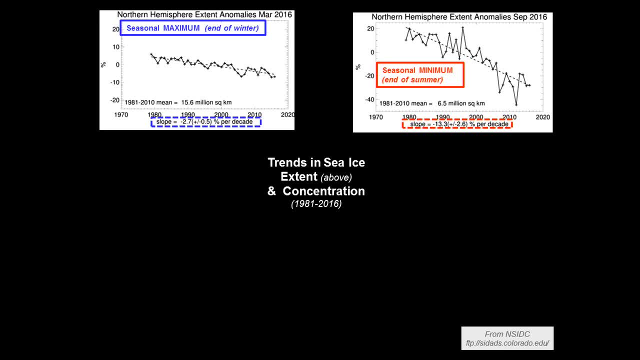 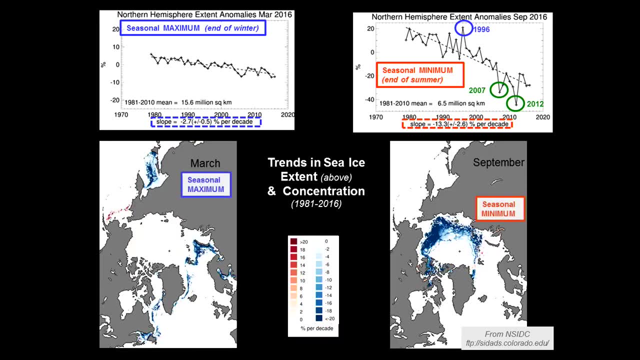 we're getting a very much greater change: 13% per decade. okay, that's, we're losing 13% of the ice per decade. we're losing in the Arctic. to look at where we're losing it in the winter, we're losing it around the edges and the 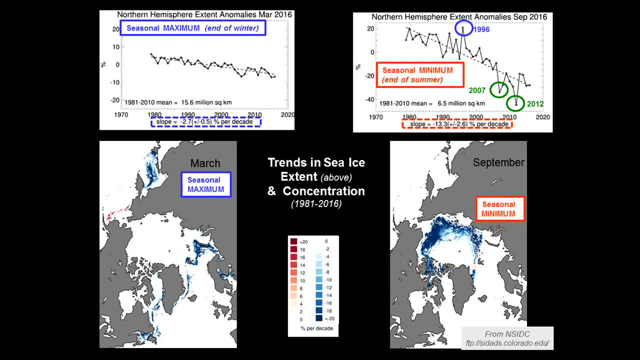 summer we're using it in the middle. we'll come back to these patterns in a moment. so we're losing ice area. oh yeah, the area that we've lost so far is about a third of the area the US. we've probably lost about 50% of the old. 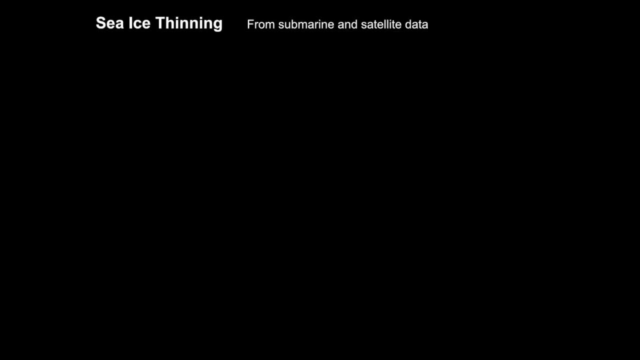 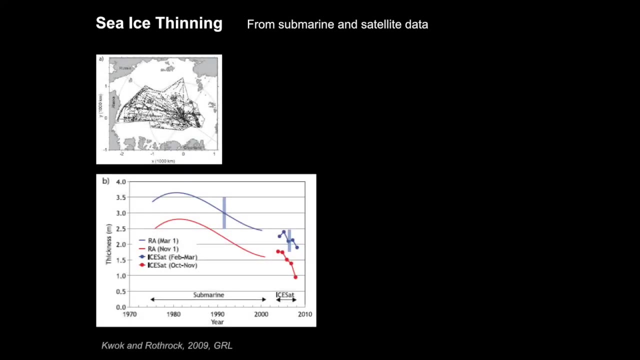 summer sea ice extent from about the 1980s. it's not just that that we've lost, we've also thinned the ice, so it's harder to put this together. we put this together from satellite images and submarines and satellite images and- but this gives you an idea- in the 1980s this is winter and Southern. 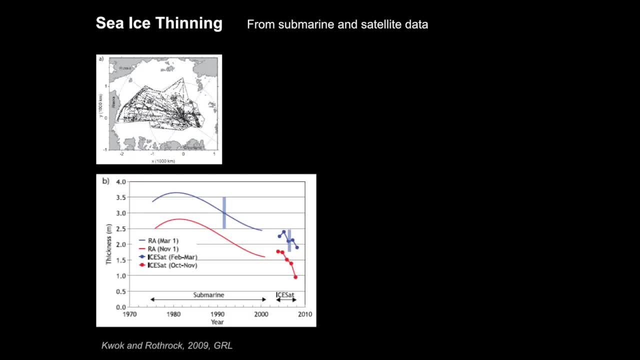 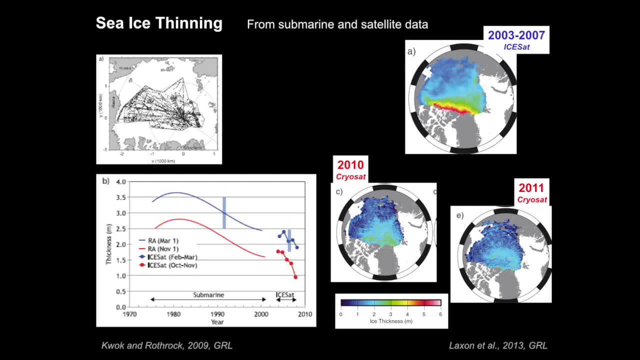 summer we had about, you know, three metres of ice, and now, in more recent era, we're down to about half that. There's satellite pictures showing you how that's distributed. there's lots of statistics have to go into this, but this is confirmed by everybody who 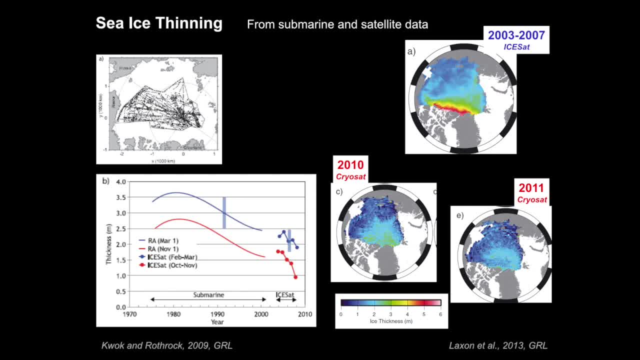 goes up there, the people who live there who talk about saying: you know, we no longer get the strong, thick ice we used to have. we only have feeble, weak, young ice. So we can say sea ice has thinned from very roughly about 50%. Put that together: we've lost extent. 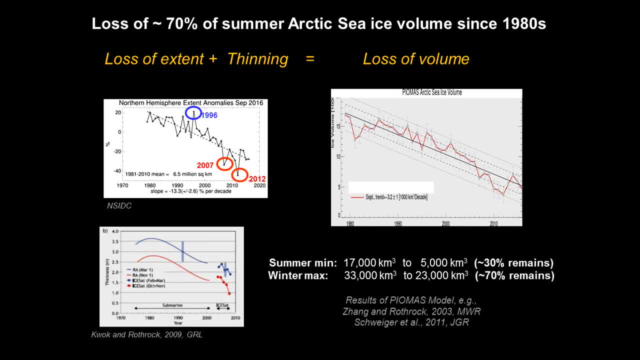 we've thinned, we end up with a loss of volume. This is our best estimate. try and put that all together, which is a model and which says we have lost basically 30%. No, we've not lost 30%. we only have 30% left of the summer ice that we used to have. Okay, Some. 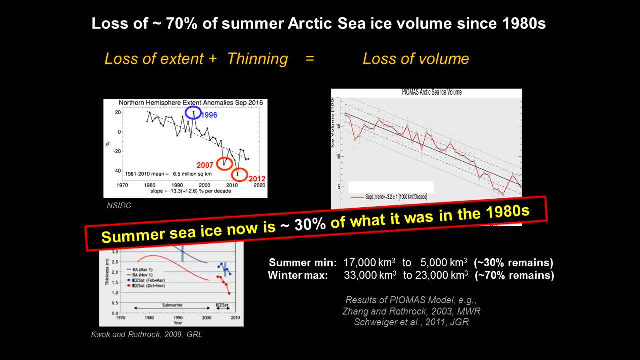 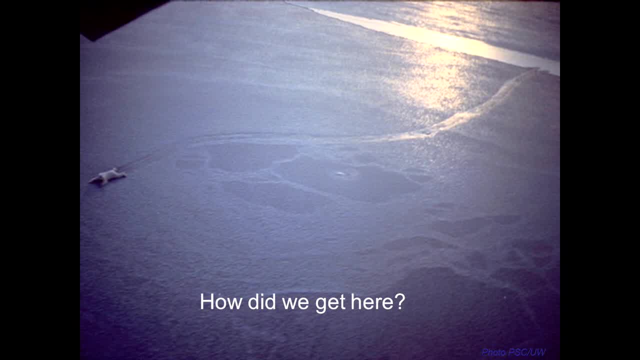 people would say this is a quarter, but it's around that magnitude, So it's a huge change we've seen in the Arctic in the last decades. How did we get here? Polar bear Always got to have a polar bear. How did he get there either? 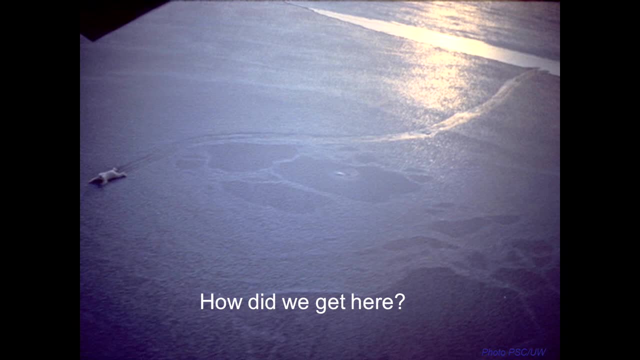 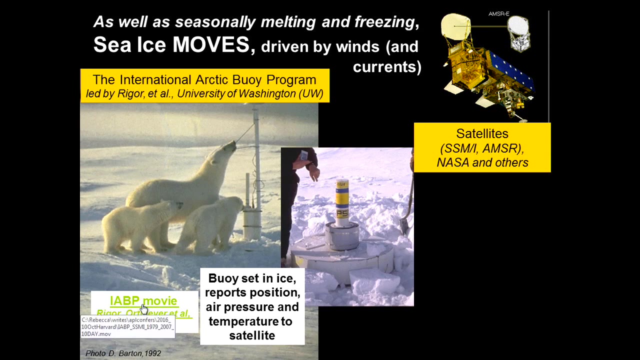 So we got there in many ways, things that we understand and things that we don't. We understand now how well the ice moves. So if we put a pole in the ice- the North Pole, the ice, the flow drifts around and the ice moves with it. To be more useful than that, 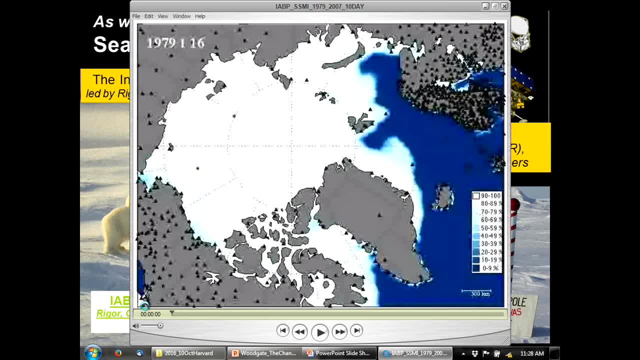 we can put in a set of instruments which will tell you their position. So dates rolling in the corner here. White is the satellite sea ice extent Going from the summer to the winter, to the summer to the winter, The little red dots. 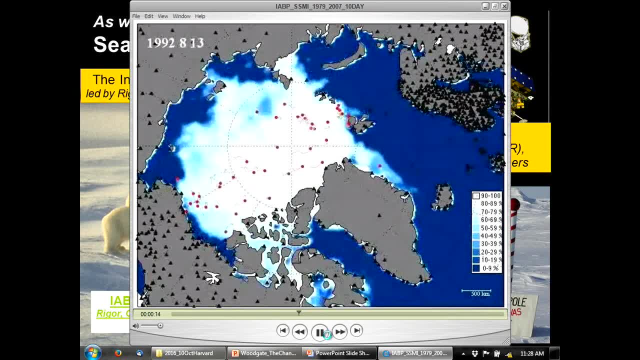 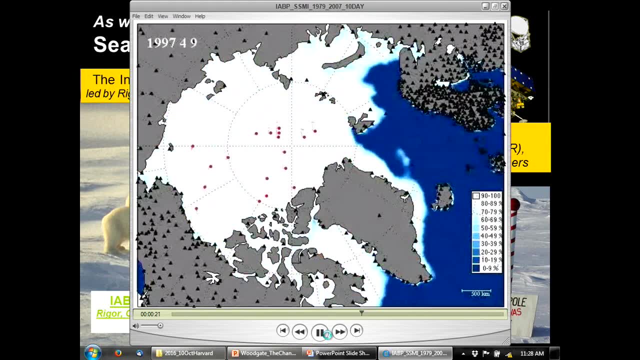 are buoys that have been put on the ice and registered their position. You see they go round in a kind of circle around here. Some of them run down the edge of Greenland like this. This is how the sea ice is moving. They're just sat on the sea ice. They jiggle around. 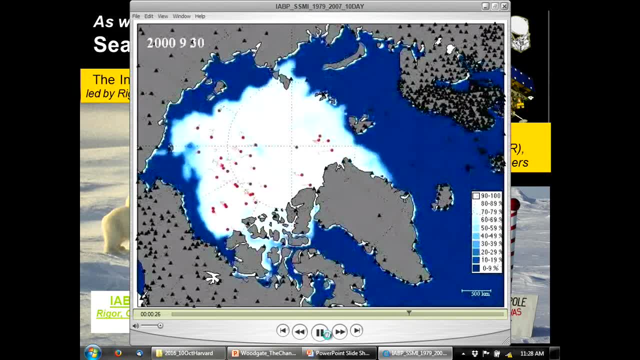 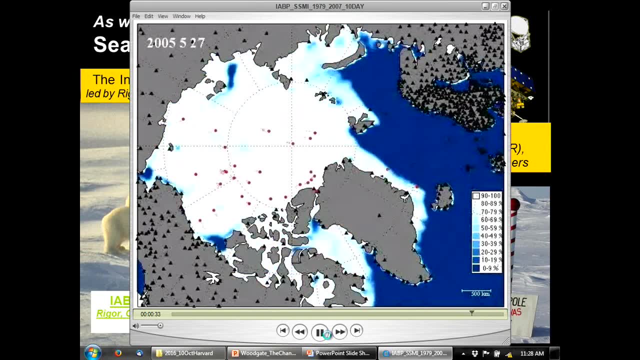 together because the wind is forcing them And we can see this pattern of a circulation there and then ice coming around here and coming out down this way, And as we come to the 2000s we see the summer extent getting less every year. 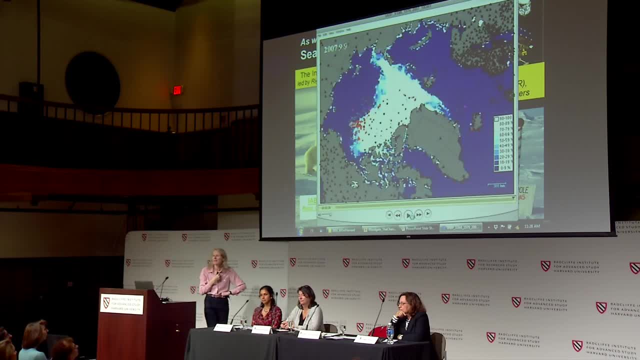 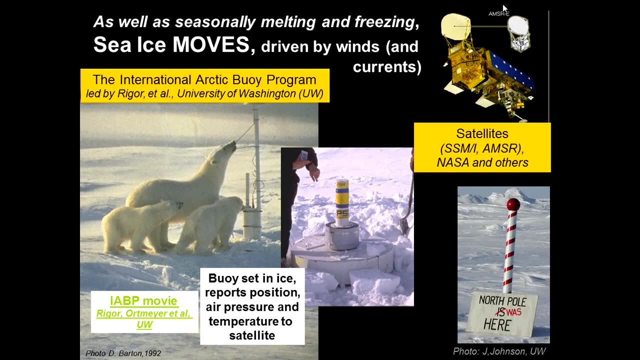 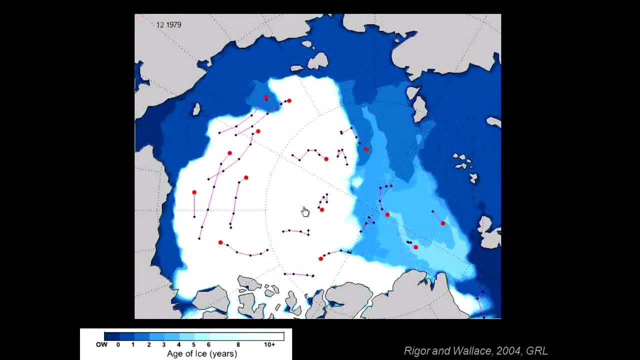 And we can see this melting back to this incredible ice melt in 2007,, which really was something that nobody expected or saw coming. So from that data we can go on and say: well, we can see how this is moving, We can tell how old the ice is. And this is a similar movie. 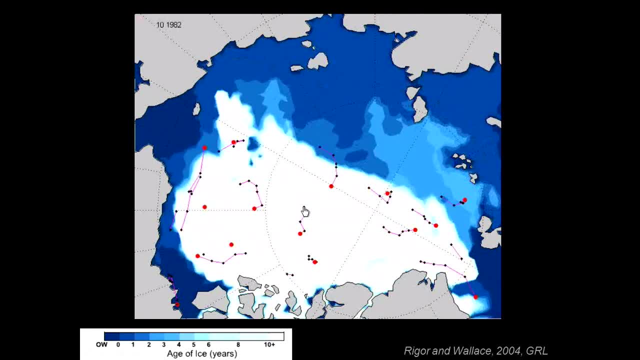 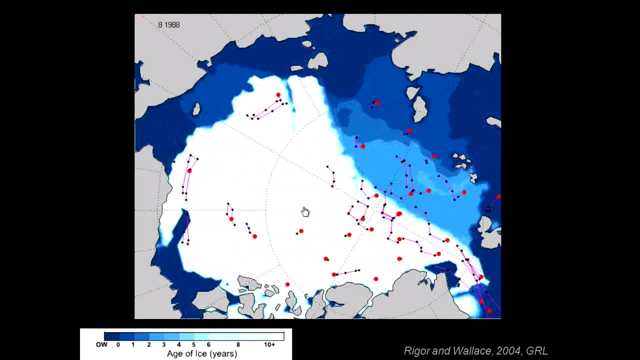 where the colours are now the age of the ice. So white is now greater than 10 years and these bluer colours are more recent, younger ice than that. It's the same buoys as you saw before We're seeing here in the 1980s. most of the ice is moving And we can see. 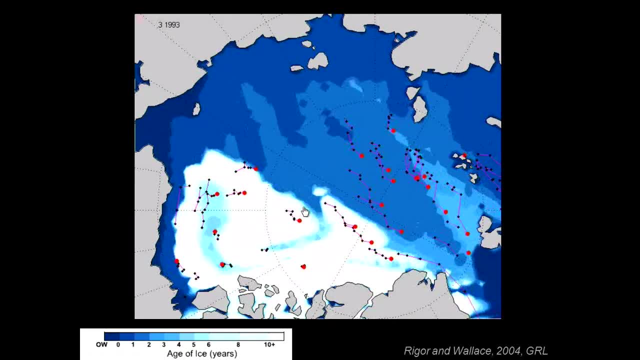 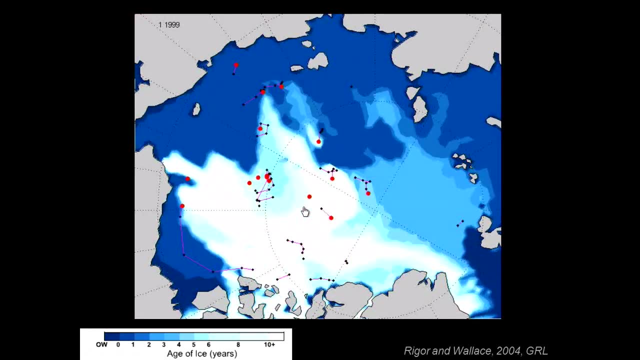 that the Arctic was covered by old ice, But changes in the wind have changed that. They've taken all this area of ice. They've managed to flush it out down here through to the Atlantic Ocean And over this time period we are losing the older ice from the Arctic and coming back. 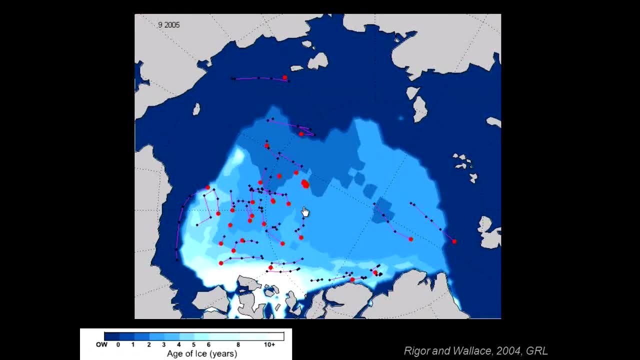 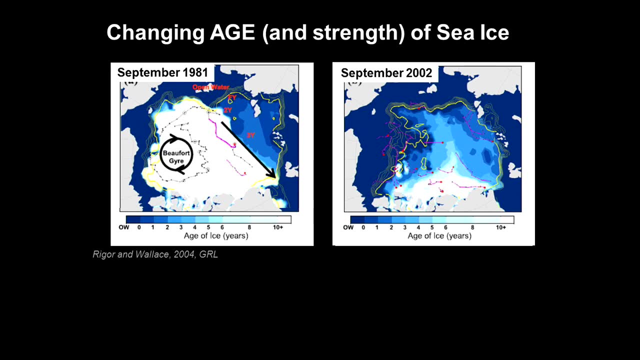 to just having a very much younger, newer ice in the Arctic Ocean. We've flushed the old stuff all away. To see the before and after, if you like, here is the before- lots of old ice, and here is the new, with very little ice left. In doing that, we can see 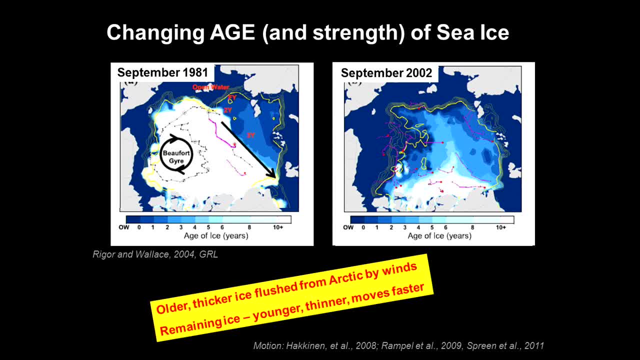 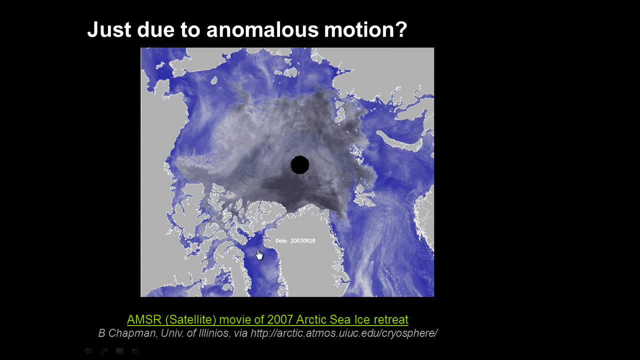 that we've flushed away the old, thick, resilient ice. It now moves faster and it's thinner. The other thing that goes with that is that it can also melt easier. If we look at how things have changed, is it just due to this motion? No, it's not. This is a movie of 2000,. 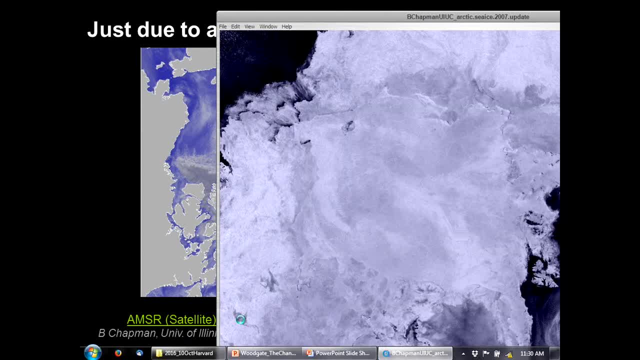 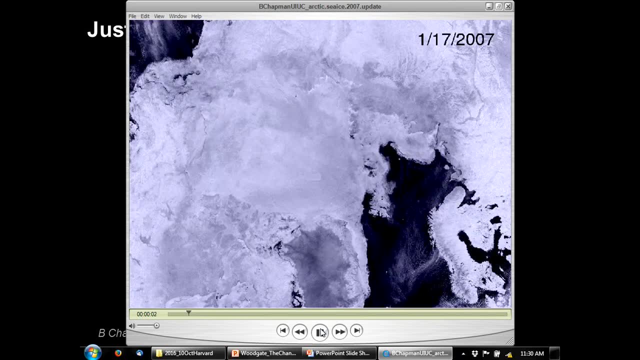 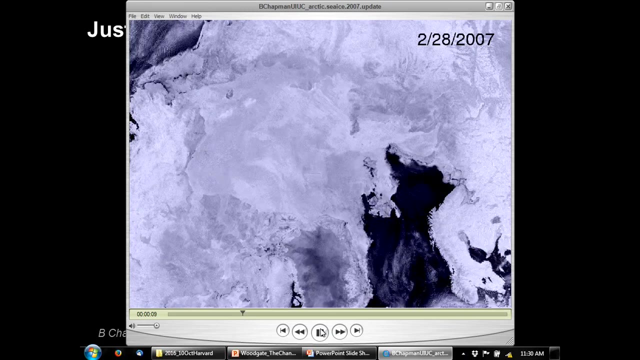 again looking at ice and clouds now. So here's Greenland again, And you'll see here the coast of Alaska, around these points, The big things that swirl past the clouds, but most of what you see underneath this is the ice moving, Sometimes as the wind blows. you'll 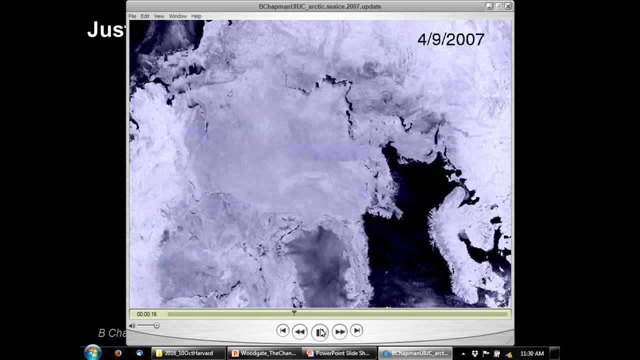 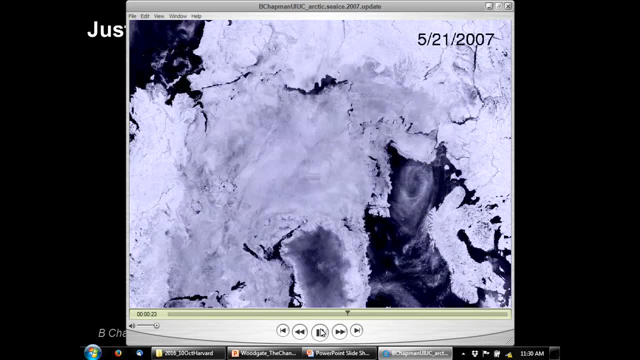 see black open up here. That's open water opening up along the coast. you see here. You see, if you watch this bit you can kind of sense a motion which is the same motion we saw before. You see these massive cracks coming across the whole of the Arctic, Those, 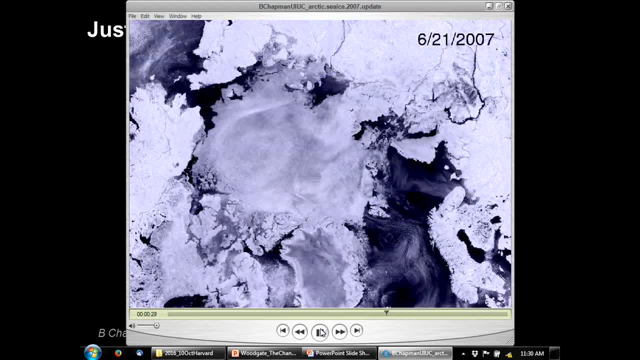 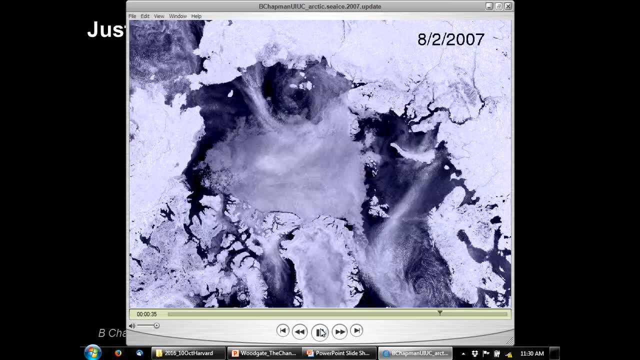 are the leads that we talked about. as the ice pulls apart, driven by winds and currents In summer. here the ice starts to pull back from the coast and you can see here the retreat of the edge, which is faster than the speed of the ice, Basically, as we watch this through, 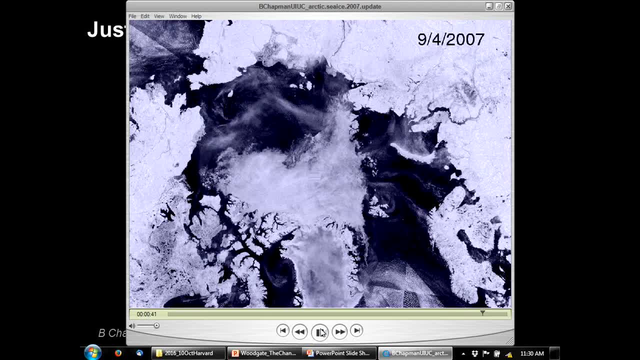 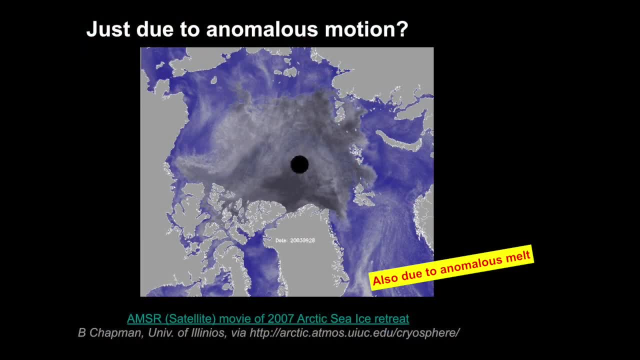 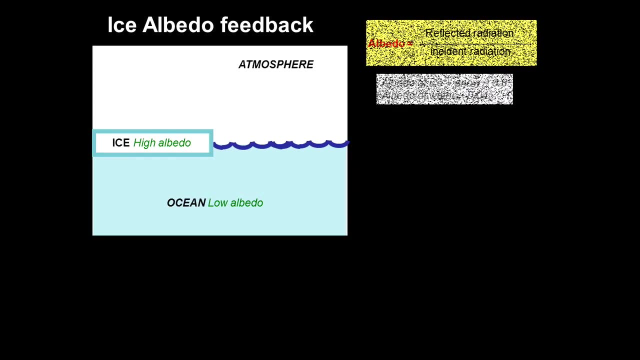 August and through September, that ice just entirely melts away. So what causes it to melt? The main thing is this idea of an ice albedo feedback. This is the reflectivity that was talked about a second ago. Quite simply, the ice is shiny. 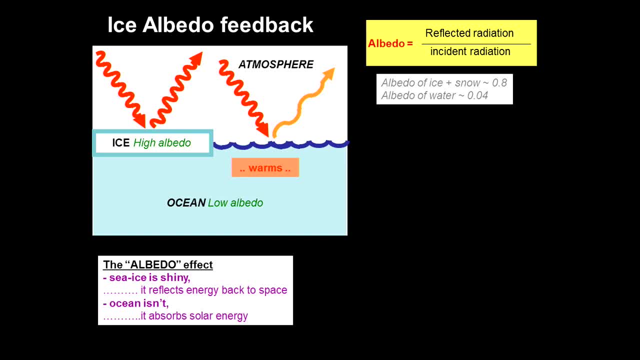 and the water is not. So if sunlight beats on the ice, it reflects that heat back to. If it beats in open water, that heat is absorbed and we get a feedback. Let's say we start with more ocean water, but water can absorb more heat. 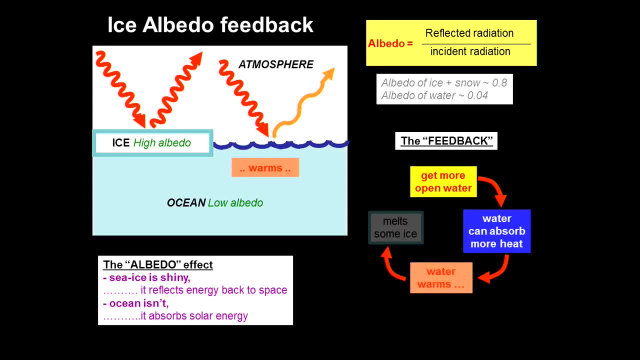 That means it will get warmer, which means it will melt some more ice, which means we have more open water, which means we go round and round this circle. It's a vicious circle, a vicious circle of demise of sea ice. The technical, physical term for that is a positive feedback. 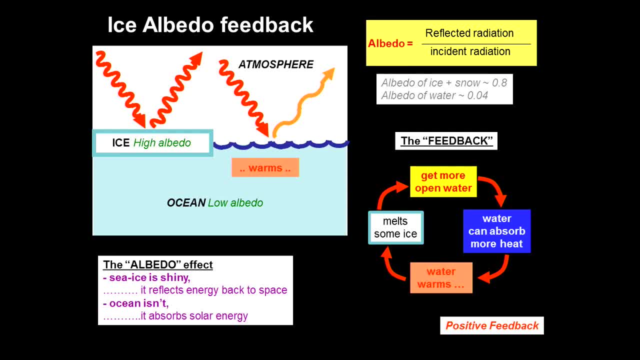 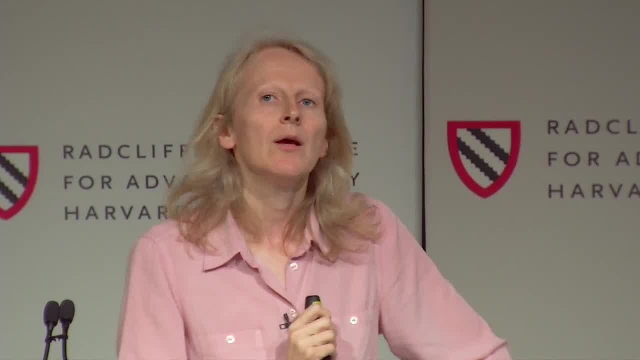 And so, once we can set this off, the only thing that's going to stop this is by turning off the light. Winter coming is the only thing that will stop this feedback. But we have to set this off. and to set this off, what can we do? 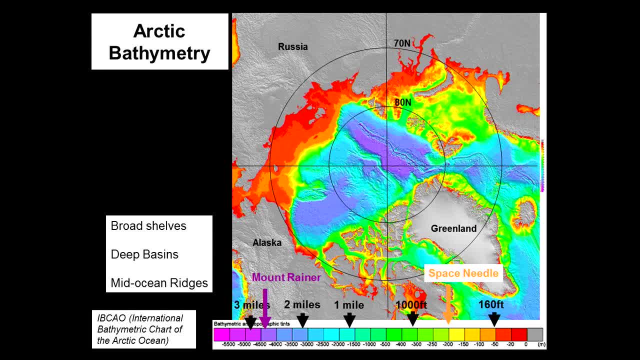 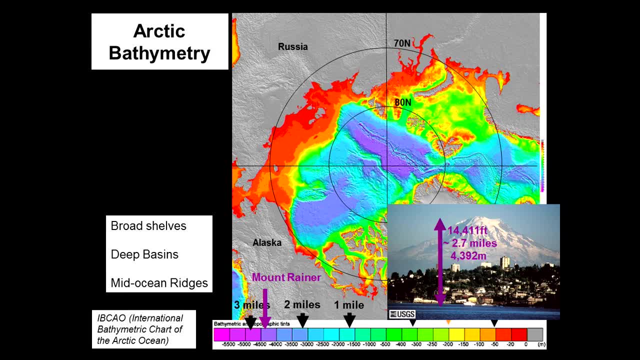 We can blow the wind off the coast, but there's a further role which is bringing heat into the Arctic, and that is the oceans. This is now a map of the bathymetry of the Arctic Ocean. Deep bits are blue. It's about the size of our local volcano in Seattle. 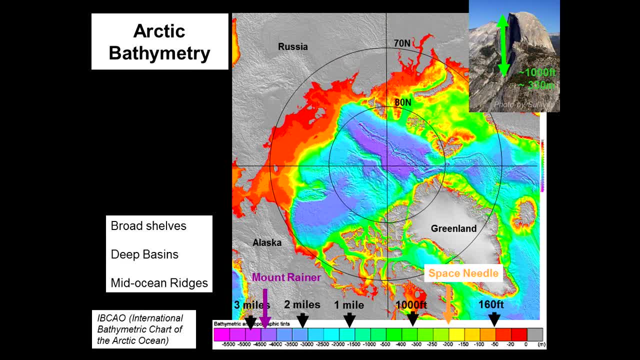 The red bits are all shallow and there's other bits, There's other things there that give you some idea of scales. We have an entrance here to the Atlantic Ocean, an entrance here to the Pacific, and waters flow from both of those oceans into the Arctic. 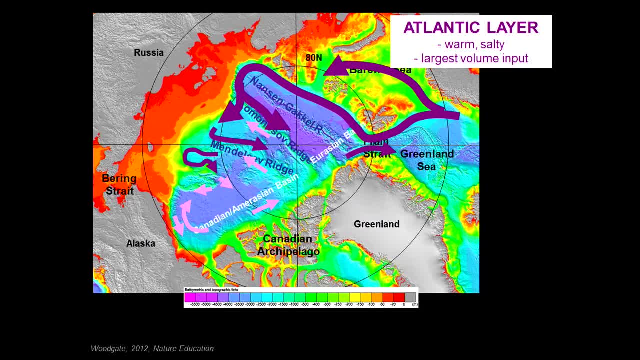 Here's the Atlantic water which comes in. It's a deep current and it likes to put its hand on the right-hand wall, like a good current should in the Northern Hemisphere, because the Earth is spinning And it goes round, following slopes and ridges. 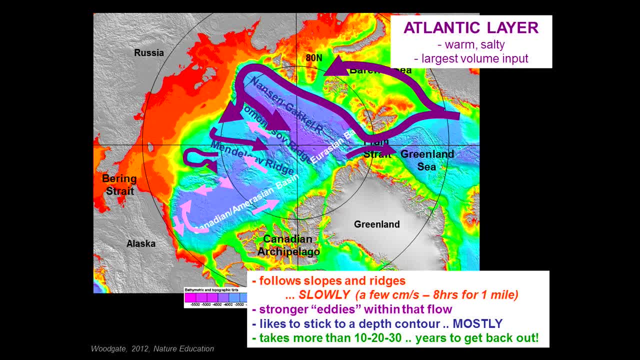 It goes round very slowly, a few centimetres per second. so it'd take eight hours to go one mile. So if we send some water in here, depending on whether it takes a few minutes or if it takes a short loop back through here. 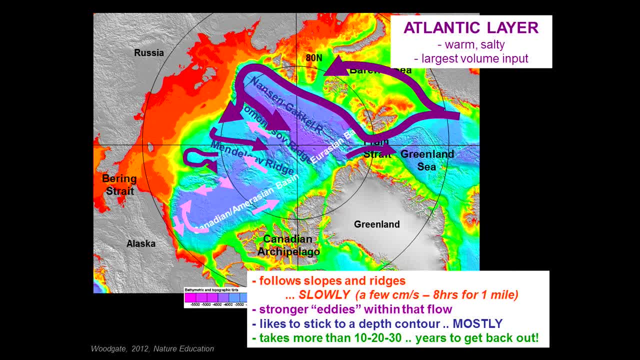 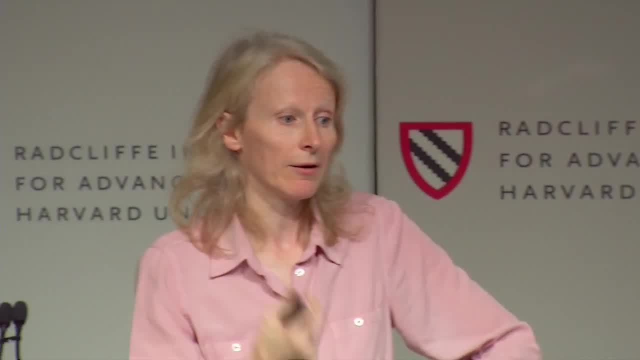 or the longer loops back through here. it can take 10,, 20, or 30 years to get back out again. So we send a heat signal into the Arctic. That's the time it's going to go round and then come back. 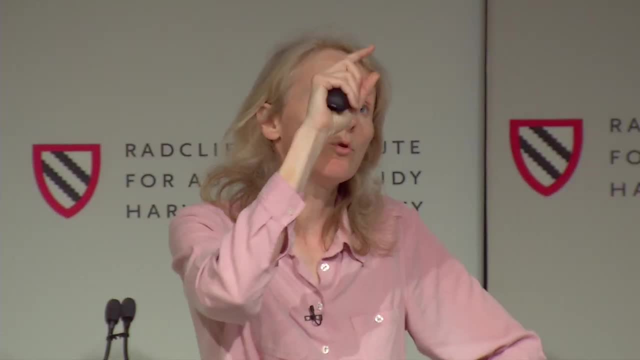 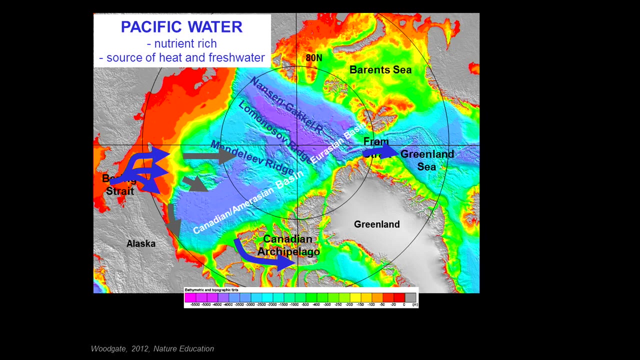 The other side, the water comes from the Pacific. That's higher up in the water column. It's also a lot fresher. It tends to stay on the top of the ocean and it's more driven by the ice and by the winds. 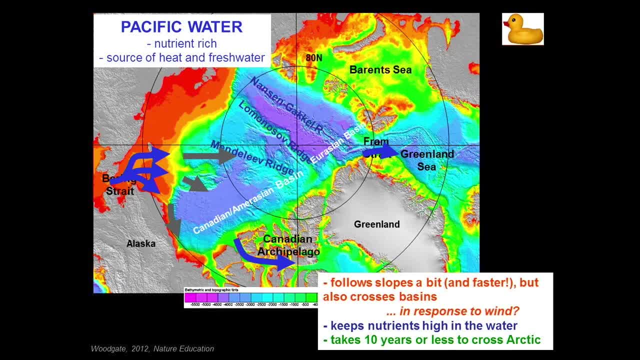 It moves a lot faster. It actually covers about half of the Arctic Ocean here and then comes out. It comes out through the Canadian archipelago, So it would only take about 10 years to cross the Arctic. What both these currents have in common? 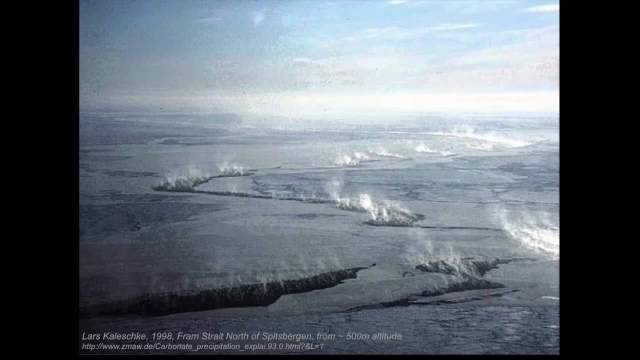 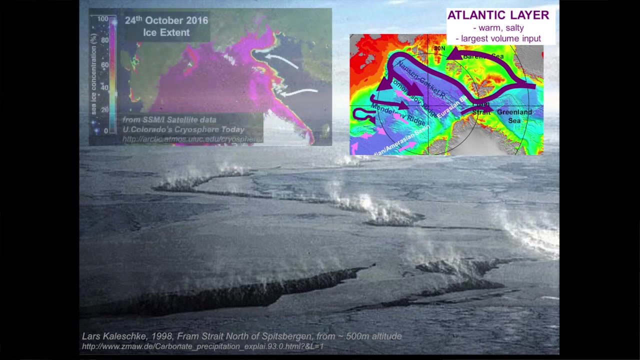 is they bring in heat to the Arctic Ocean. Here's some pictures of Fram Strait seeing the heat from the ocean coming up and melting the ice. If we look at that Atlantic layer, the arrows that we had for that, and we look at the ice edge. 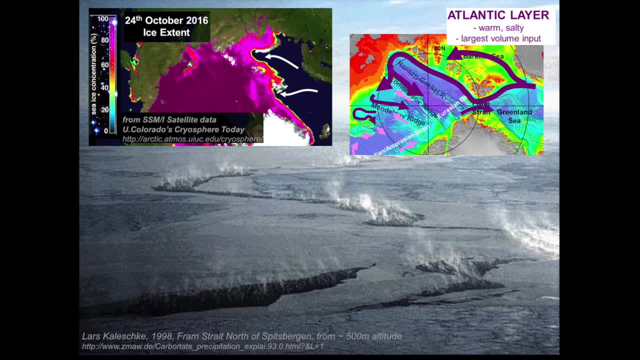 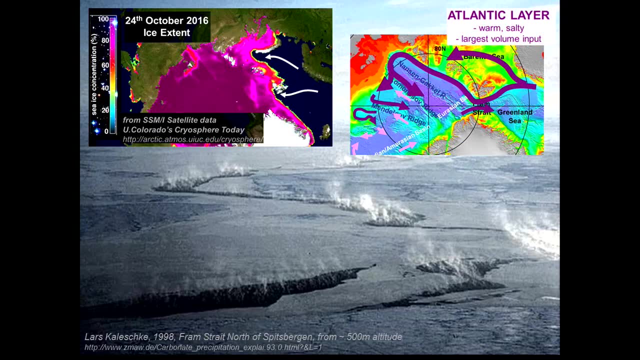 we can see here these tongues of hot water coming across the Greenland and the Barents Sea, here melting back the ice edge, Very suggestive of the patterns that the oceans are bringing in the heat which is melting off the ice And I show that as a pattern. but we can do the maths. 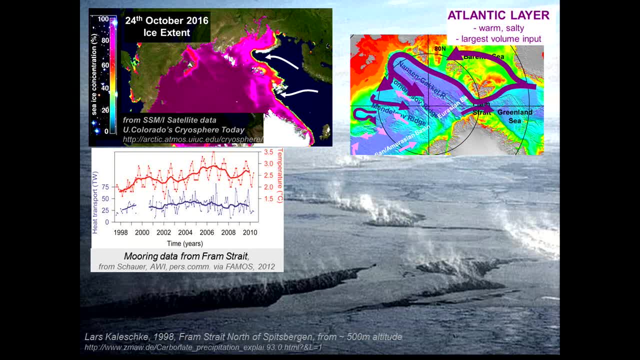 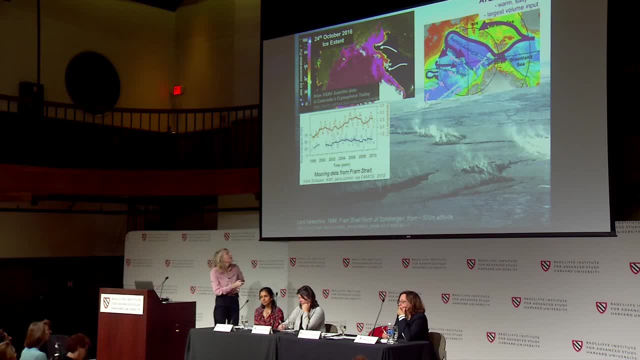 We've had measurements in these channels at great expense for many years. We can see that over these decades the temperatures of the waters have warmed as we go through the channel there, And you can do the maths and you can work it out. 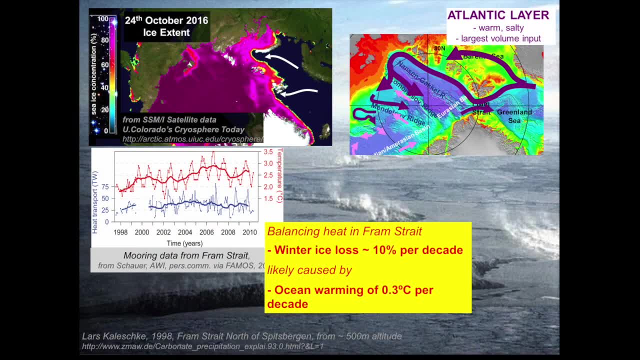 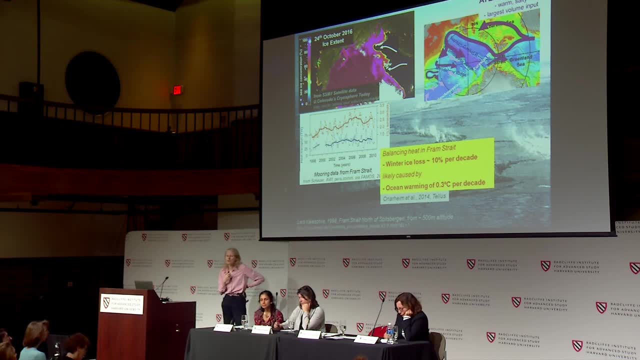 but we're just about right for the numbers. The amount of winter ice that we're losing in this area, which is 10% per decade in this particular area, is likely caused by an ocean warming of 0.3% per decade. 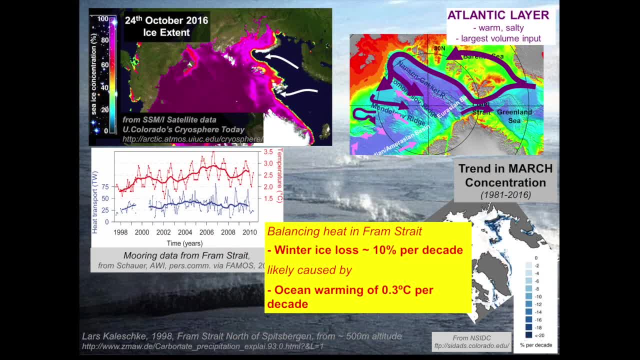 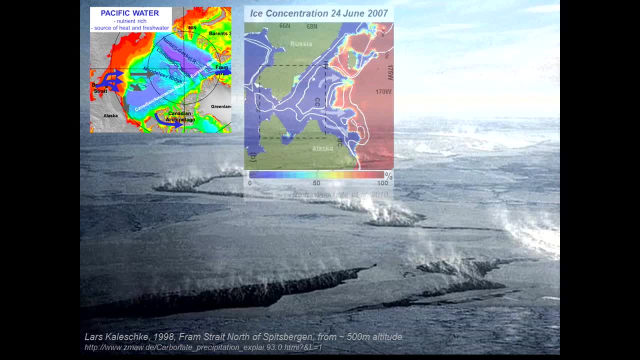 It corresponds to that map we had of where we saw the ice going away in winter. If we flip over to the other side of the Arctic, the Pacific, here the waters come in are only warm in summer, but we see the same pattern. 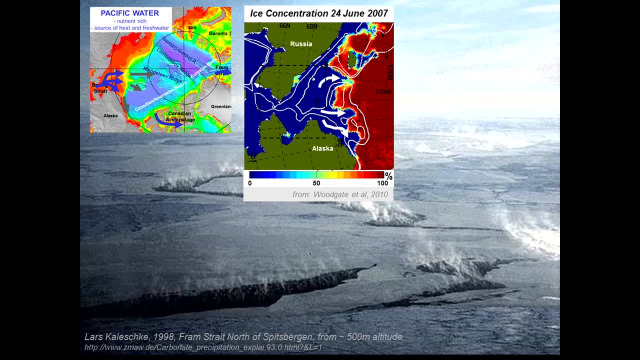 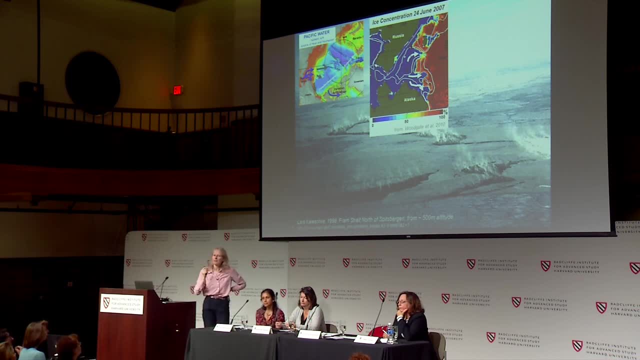 We have here the same: the tongues of water, again driven by the topography, melt back tongues in the ice. And this is now. we've got the sun up here. we set this off and now the ice albedo feedback. can take over and melt back the ice, The other thing that this water does: it ends up deeper in the Arctic Ocean and it can act as a gradual thinning to the ice. that is there: yet another nail in the coffin of the poor Arctic sea ice. 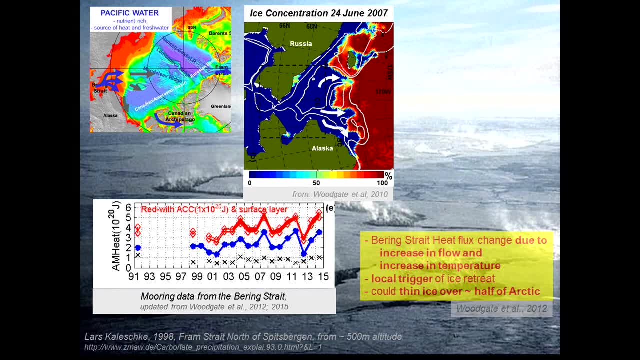 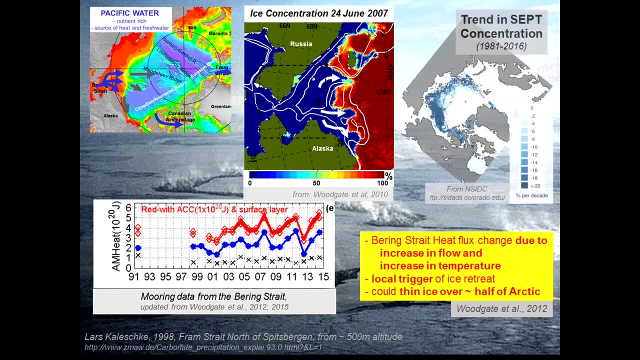 Again. we've had measurements here for many years. We can see this heat flow increasing and we can do the maths and we can say: this is the effect of these heat flows. We've got warmer waters coming in from both sides. 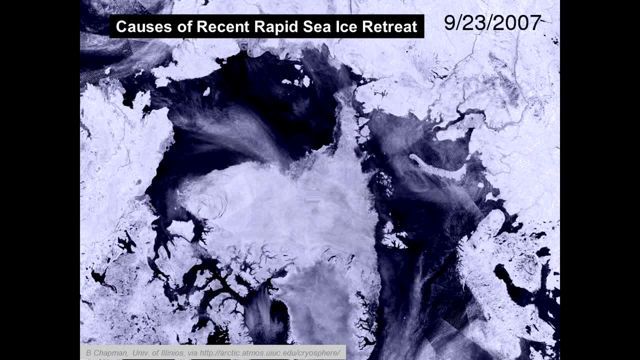 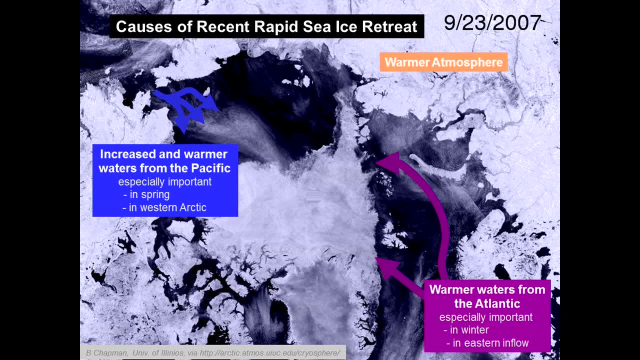 So what is our causes of recent sea ice retreat? The increased heat from the Pacific, increased heat from the Atlantic, warmer atmosphere and a lot of the water coming in from the Arctic. So we've got the Arctic ice melting. we've got the Arctic ice melting. 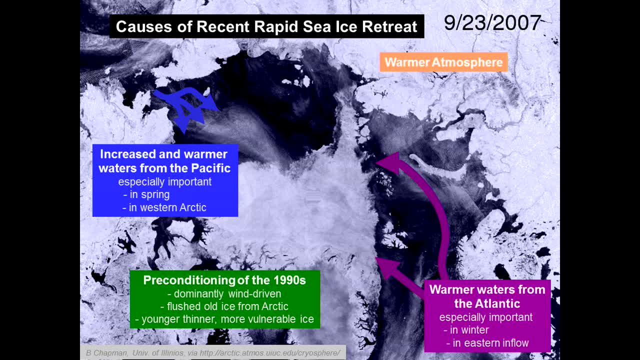 and we've got the Arctic ice melting. And what's really interesting is that these interplayers I haven't talked about, but that's coming into this too- added on to a preconditioning where we have flushed this older ice out of the Arctic. 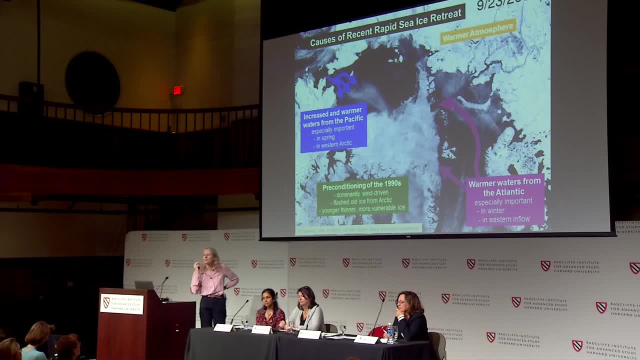 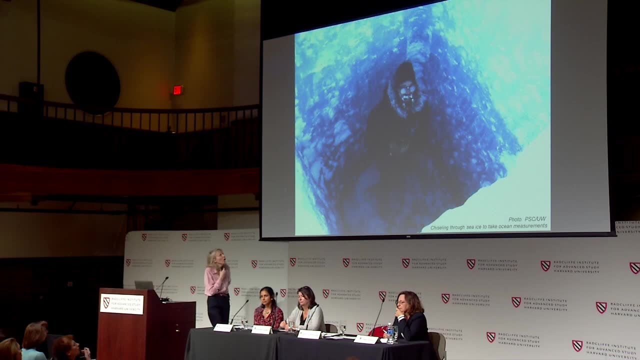 So all these things are conspiring to give the Arctic a really bad day, right, We've all had bad days like this. This is the Arctic's bad day. Quite how these interplayers, things that we still have to put together. 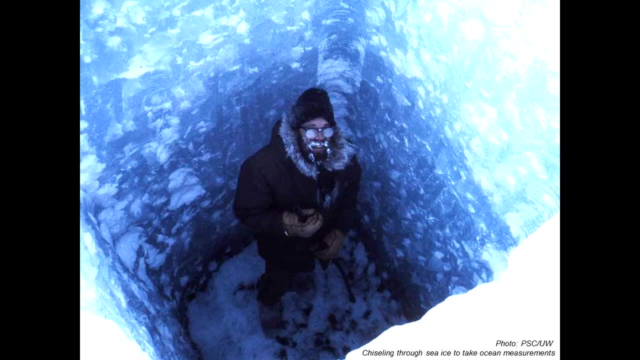 we have so far not managed is how we used to do Arctic oceanography. This is one of our technicians who has chiseled his way down through a bit of sea ice. This is a good bit of sea ice Chiseling down so he can get to the ocean below. 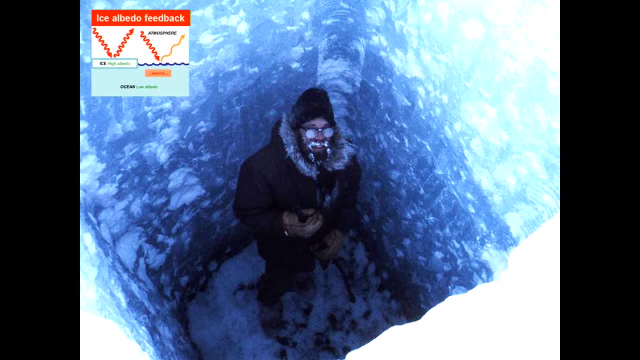 Digging himself a hole. The ice albedo feedback is kind of a killer in all of this. It comes with the idea of polar amplification. We saw that on an earlier video so you may not have been looking for it. The poles are going to warm first. 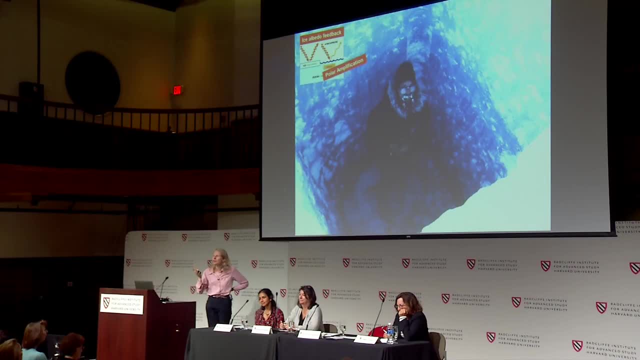 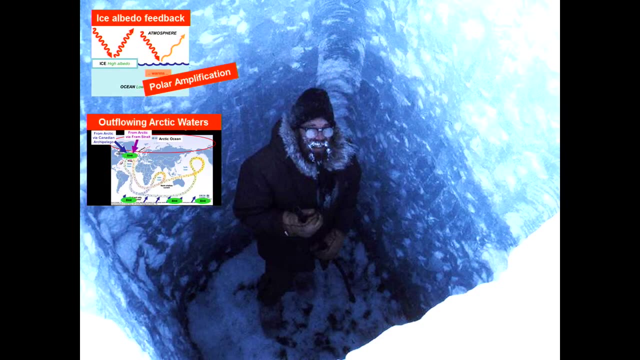 especially the Arctic, because we are losing the albedo, We're losing the shininess of the Earth and we're allowing all that energy to absorb into the ocean. Quite how that is going to play out as we push those Arctic waters into the rest of the 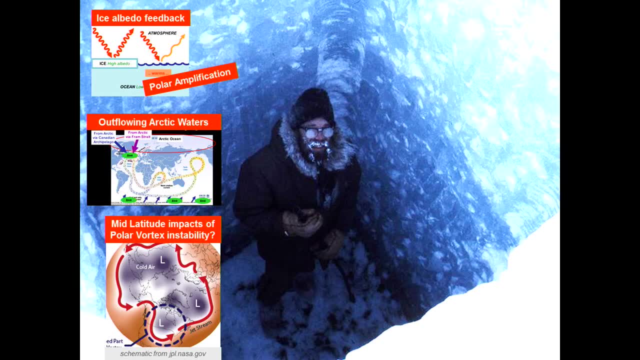 Those wobbles are thought to be driven by changes in the sea ice extent, and that gives us the cold air outbreaks and the dumping of snow onto the East Coast that we've seen in recent years. This is how the Arctic extends its fingers down. 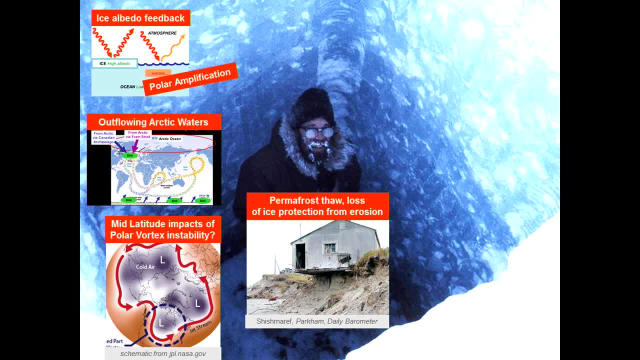 into mid-latitude weather. There is also the impact in the Arctic of the warming that we're having. We are permafrost, thawing, loss of ice, protection from erosion. If the ice pulls back earlier, the storms can affect things more and 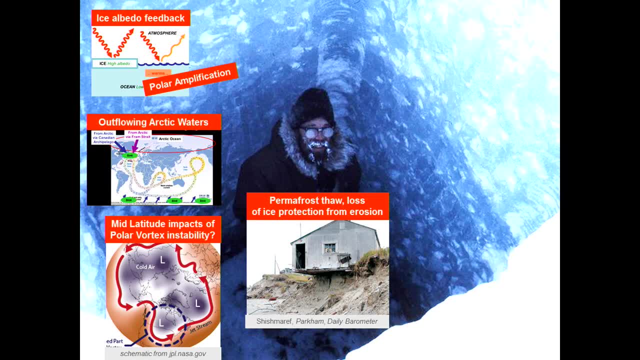 we have whole villages falling into the sea, Loss of infrastructure in terms of roads, buildings that are built on permafrost. Also within the permafrost we have a large store of methane hydrates. These are frozen methane under the sea, currently stable. 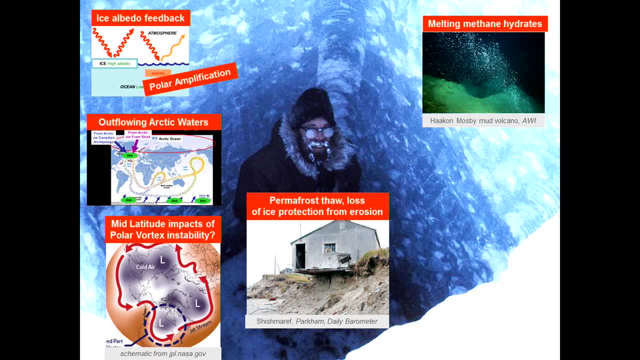 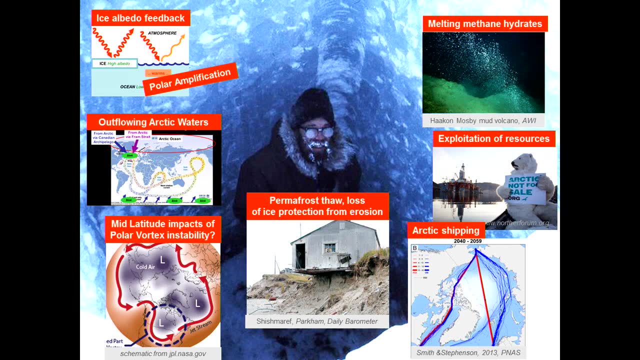 but as we warm, we could release that with potentially huge consequences. We don't quite know how that will play out either. We also have with this the opportunities which are coming from this exploitation of resources and Arctic shipping, which can now talk about going across the pole. 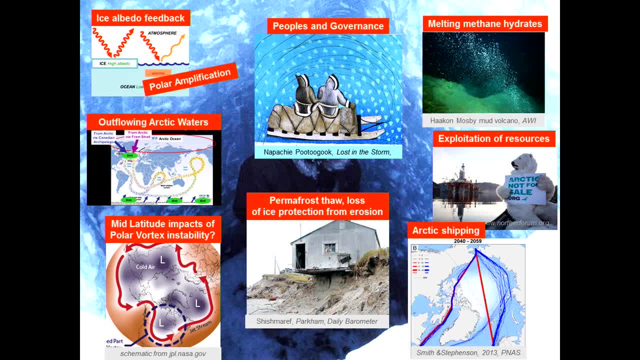 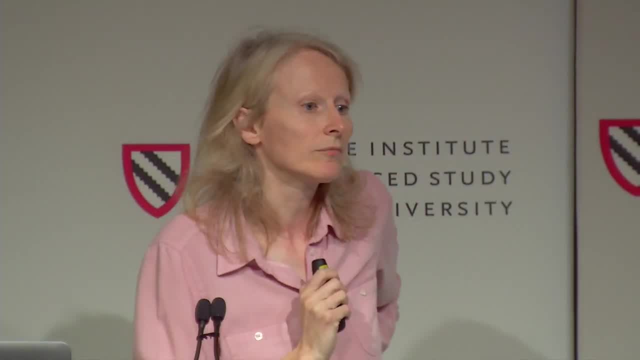 In all of this, too, we've got to think about the peoples and the governments. There are people who live up there. this is their way of life, and they're the governments of the world who are clamoring to own that piece of the ocean. 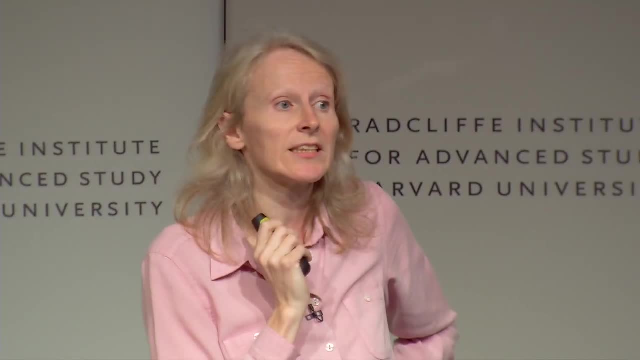 So what have we seen in our trip around the Arctic? We've changed the seasonal ice extent, how it changes, how we've thinned the ice. If you take just that one number, take away this, we are only left with 30%. 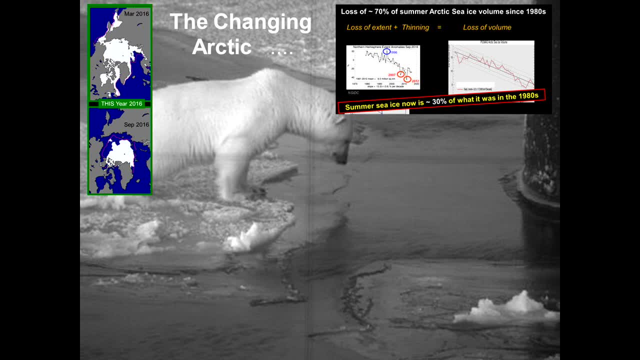 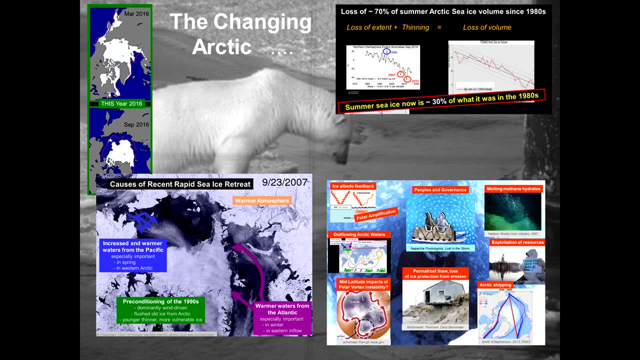 of the ice that we used to have in the summer just a few decades ago. We've looked at why things might be causing that and we've looked at the possible implications of all of this. It's a field which, because of the 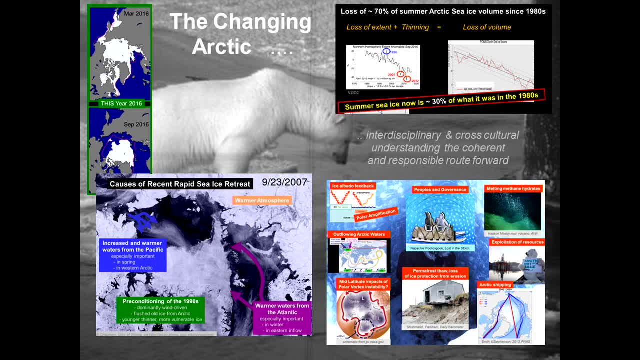 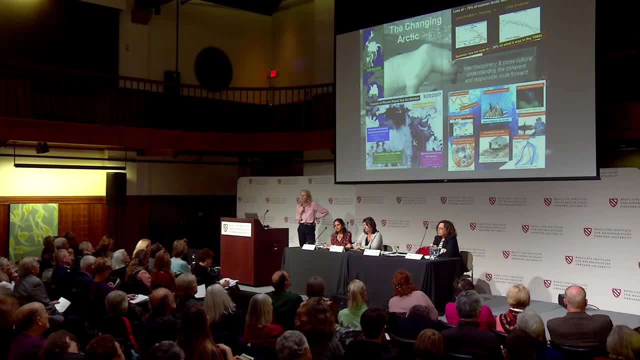 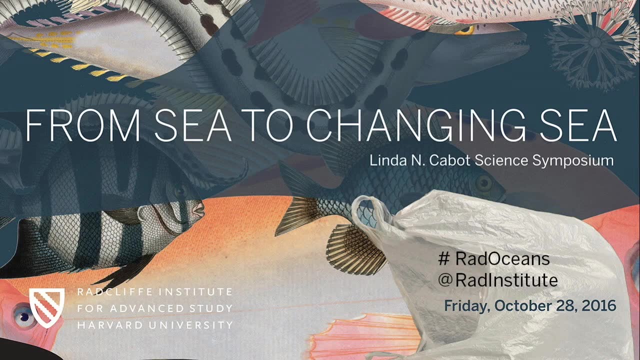 ramifications, these broad ramifications and the way the thing interacts. we really need not just an interdisciplinary but also a cross-cultural approach to have a responsible and coherent way of going forward into the future. Thank you. Okay, now for some more good news. 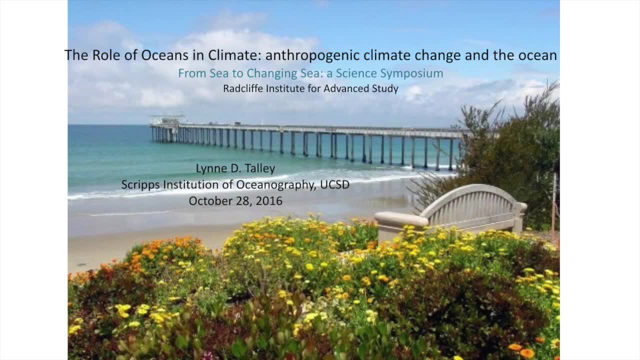 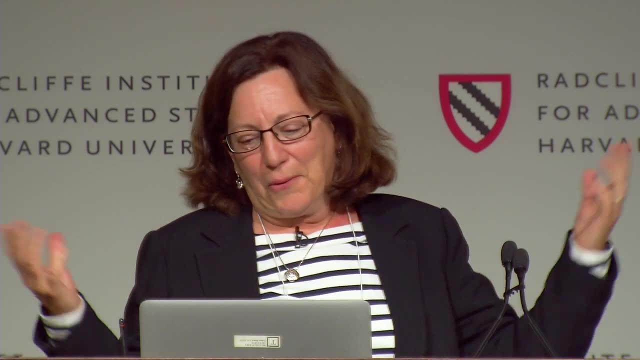 Here we go. Well, I live in a. I'm from Scripps, This is what it looks like every day: show up here and have to put on a jacket. I thought I would go ahead and put my cartoon, my favorite one, out in front. 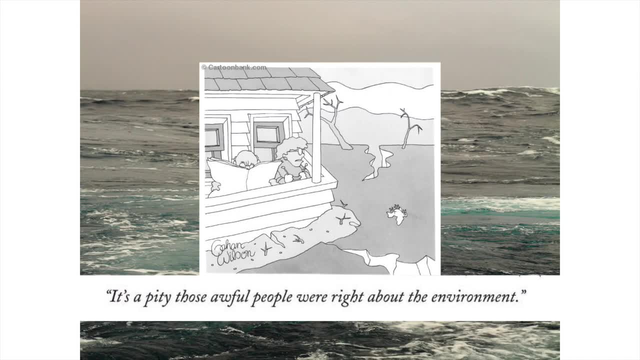 because we've lived in kind of a politicized environment the last few years as climate scientists and I think it's ameliorating a little bit. We're going back to some sanity, but this is one I've had in there a long time. 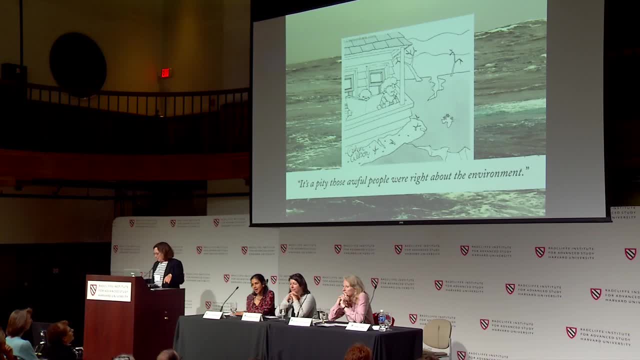 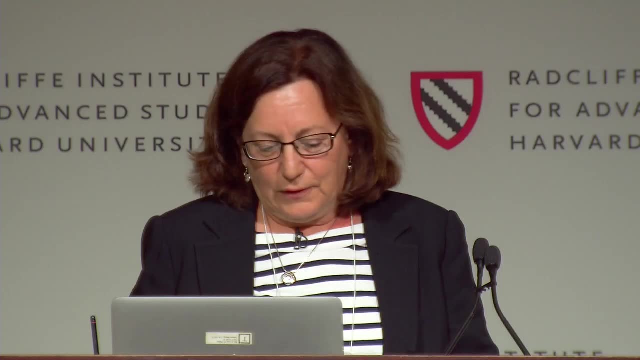 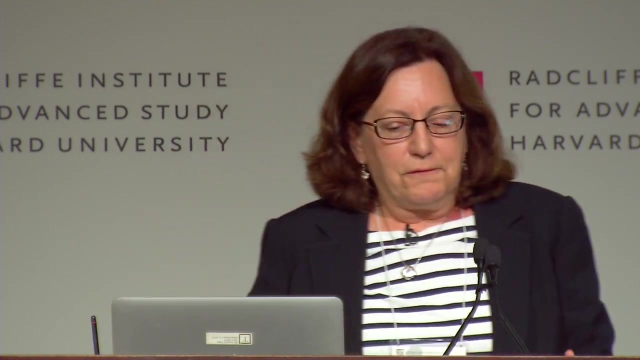 And I'm going to talk a bit about how we get from oceans to drought, Or what we can learn about the water cycle of the planet from what we measure in the ocean, And I actually have a very brief set of definitions, because we have actually, I'm speaking from 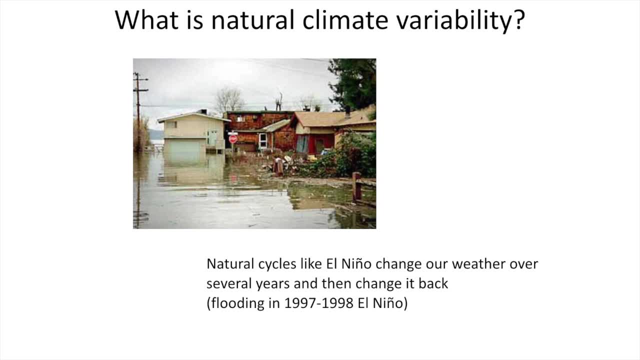 a place I'm going to show a lot of results from the Intergovernmental Panel on Climate Change, IPCC. I had the great privilege to be part of it- the last two reports We put together. the first time it had an oceans chapter two times ago. 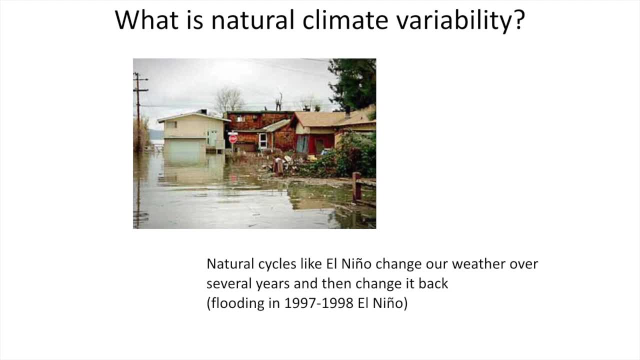 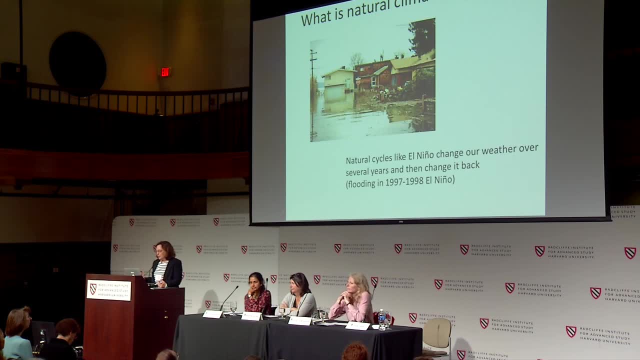 And we continued that with this one. So I'm going to show a lot of stuff from a particular slant in the IPCC of how the oceans are changing and how they contribute to climate change, But first you want to know what we're talking about. So there's. 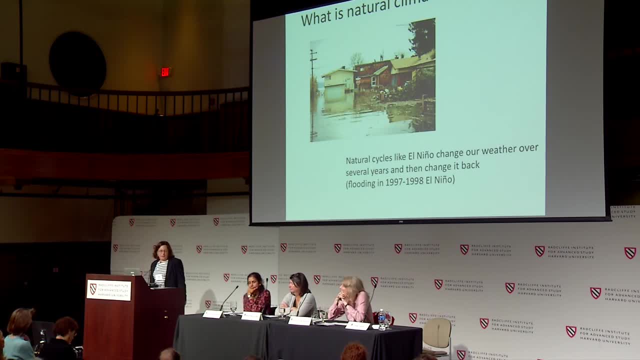 climate And there's climate variability. We have a lot of that, And there's El Nino. there's, you know, some years are stormy, some years are not, etc. That's natural And we have a major natural climate variability. 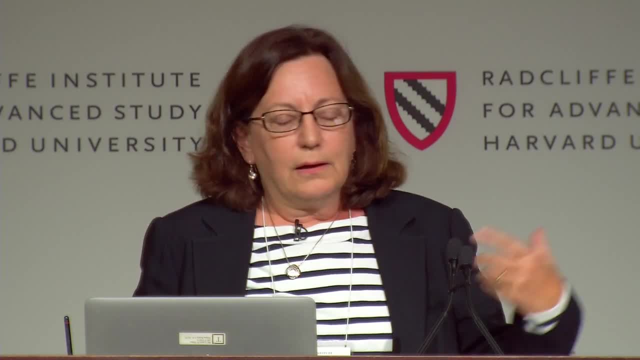 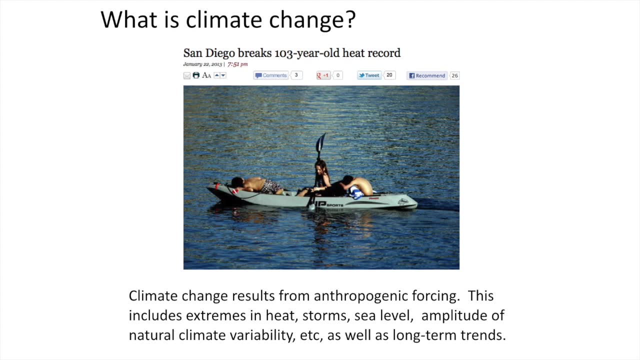 in the planet And that can be affected by climate change, which is what we drive through- anthropogenic forcing, And so we're seeing all kinds of records now. So I just want to get those two definitions in place. It's kind of. 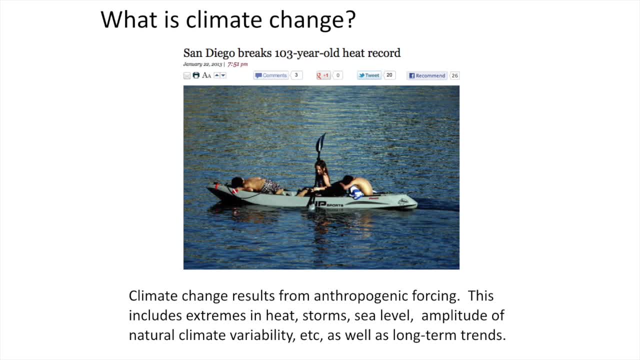 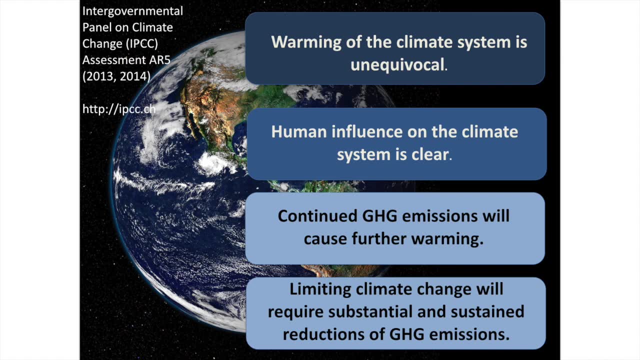 well, we have a framework there. These are four major overarching conclusions from the IPCC. This is not the oceans part. This is the whole thing. Number one which Susan Solomon put forward in the 2007 IPCC as the head of the working group one: warming. 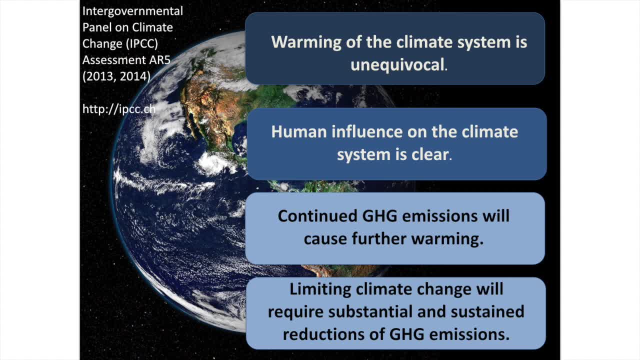 of the climate system is unequivocal. We came home from that with buttons to wear. Warming is unequivocal. Global warming does not cause ice ages. That was the second part of that Number two. human influence on the climate is clear. Number three continued. 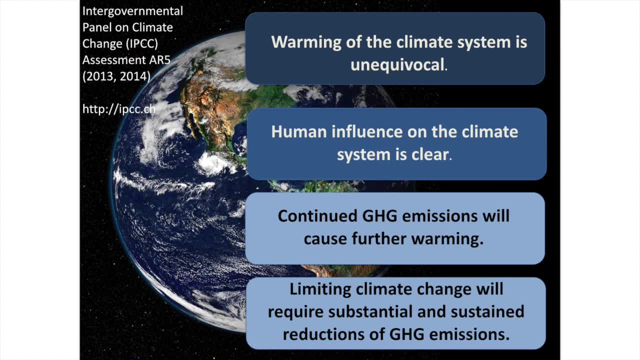 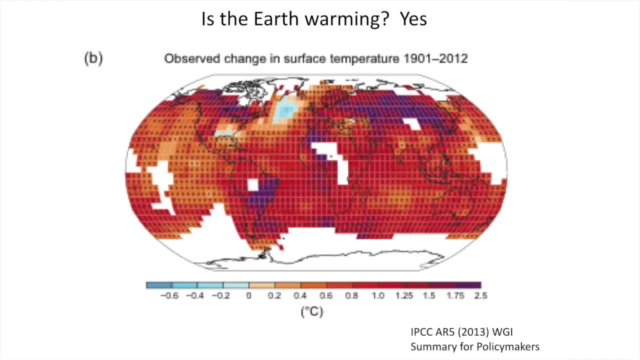 greenhouse gas emissions will cause further warming. And number four: limiting climate change requires substantial, sustained reductions of emissions. So let's look at the Earth. Is it warming? We've already seen this in video. This is the trend since 1901 up through 2012.. 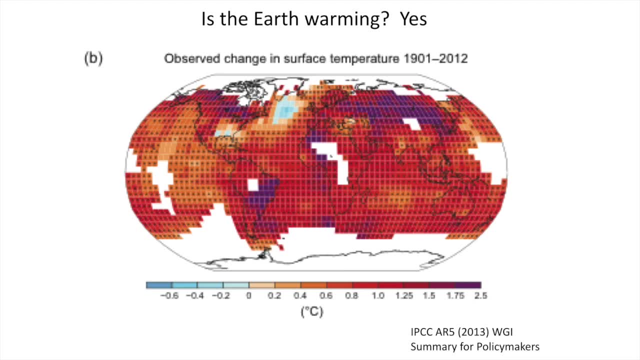 Where it's white is where there's not enough data. Mostly it's warming There it is, And it's mostly warming over land, but it's warming over the sea And that's important. This is from this wonderful NASA website, climatenasagov. Go on. 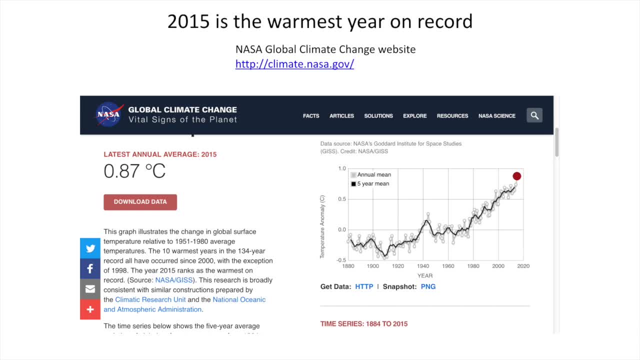 there If you want to put something on your Facebook page every day. from there. it's great. There's our graph And when you go online, that red dot at the end animates Boom, boom, boom. It's the hottest. 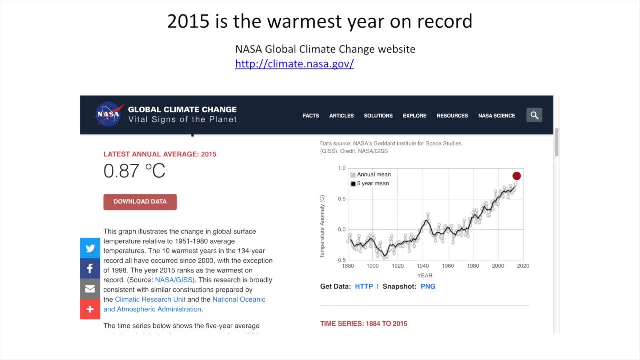 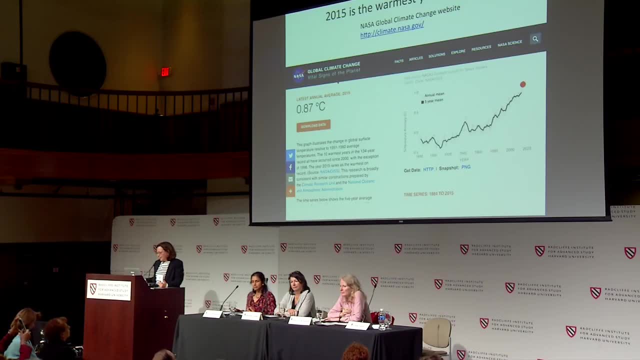 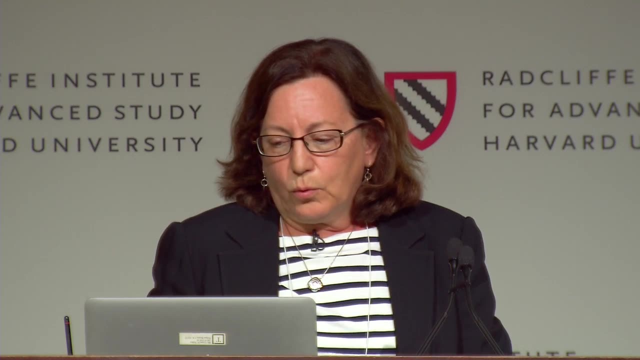 ever, measured with direct records, this past year And this year, 2016, was higher. So there we are: We're getting warmer, And they give you a nice number for how much warmer we are. It's almost one degree warmer. It's projected to get warmer. 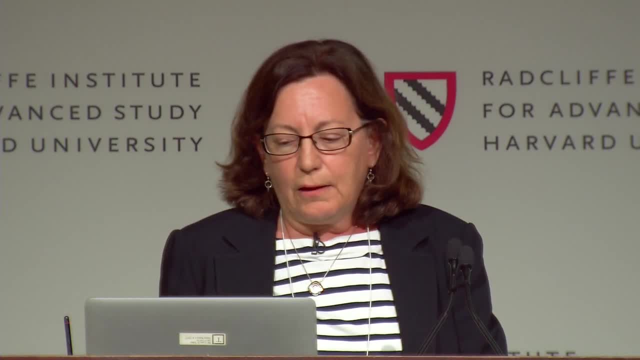 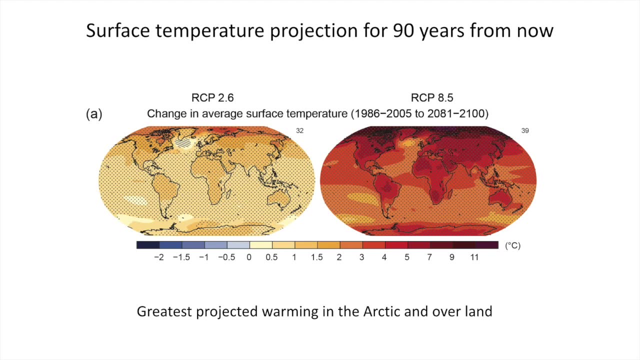 And there's the IPCC has different ways of going about that, with business as usual or some reductions or whatever. So you get from moderate to extreme. The one on the left is obviously more extreme, But that's where we're going if you just burn it all. 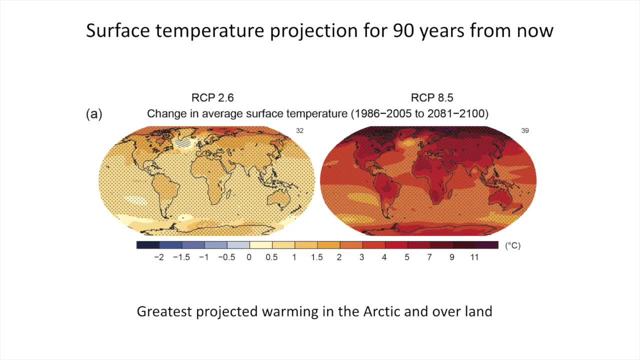 And you see the polar amplification that Maureen and Rebecca were talking about due to the ice changes in the north And you see, the ocean in the south is not doing a lot. There's a lot of ocean down there. Water has a lot of heat. 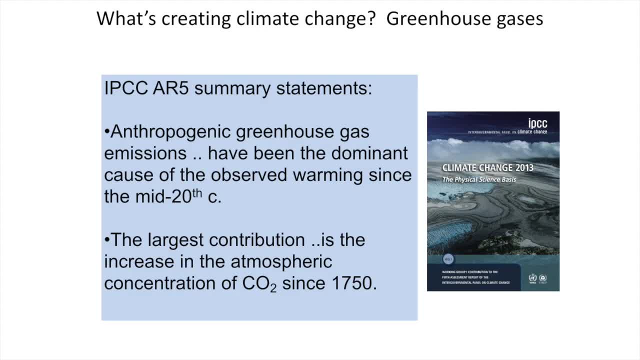 capacity. What's creating climate change? Greenhouse gases mainly. This is the big elephant in the room, And they are the dominant cause of observed warming. There's other ways. It's a very complicated subject, but this is the big part of it. 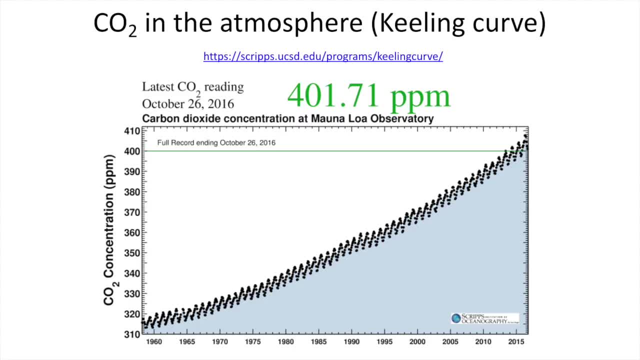 And the largest contribution is CO2.. And this is the Keeling curve last night: 401.. We're actually at the low for the year because we're at the end of the northern hemisphere summer. This is measured at the top of Mauna Loa. 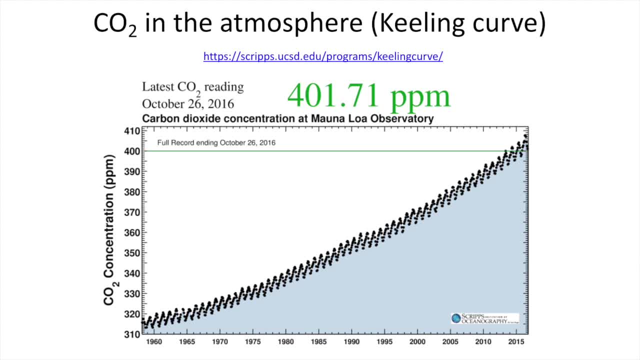 Dave Keeling set this up in the international geophysical year 1957. And with dogged persistence kept it going and now it's recognized as a really amazing record. You see the planet breathing and summertime and wintertime, summertime and wintertime, and 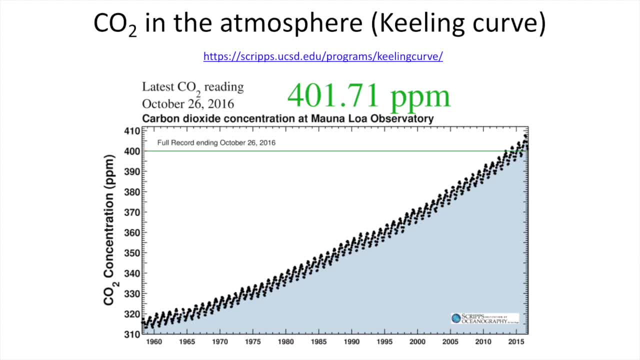 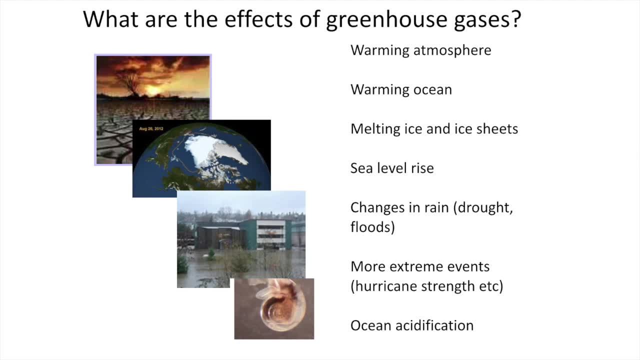 relentlessly going up, And that's the tail at the end of the curve that Maureen showed What happens with the greenhouse gases. We get lots of stuff happening, Bad stuff. Well, different stuff Depends on whether it's good or bad. 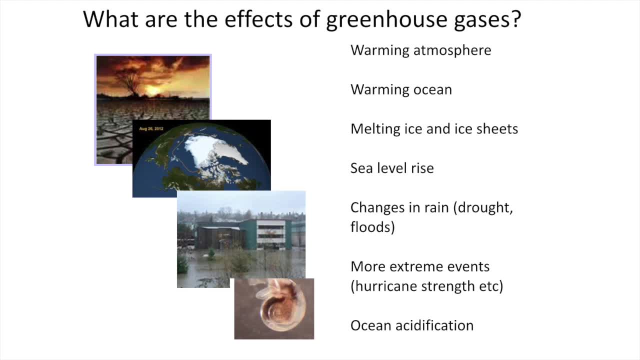 Warming Atmosphere and ocean. We melt the ice. We melt the ice sheets, We raise sea level. We do change the hydrological cycle. We're going to change the patterns of drought and floods- Not the patterns, but the strength of drought and floods. 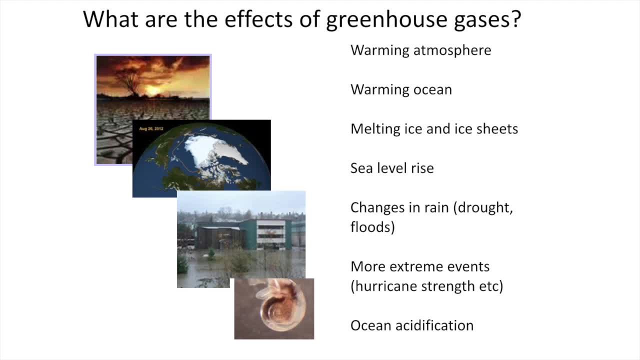 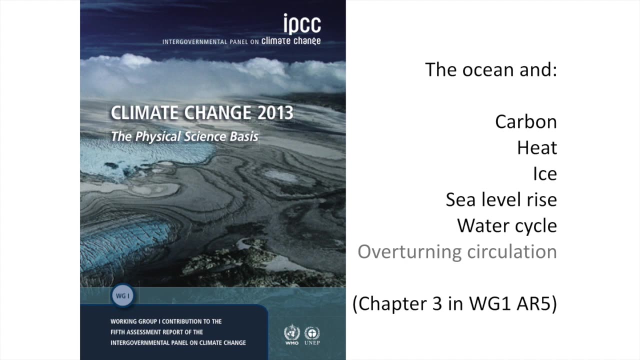 We have more extreme events. You can't attribute any given storm to global warming, but you can attribute years of changes in extreme events. Ocean acidification is another important one for the ocean. So, looking at the ocean, has the ocean participated in each? 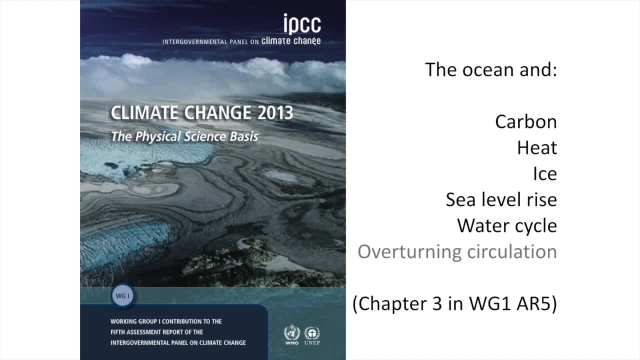 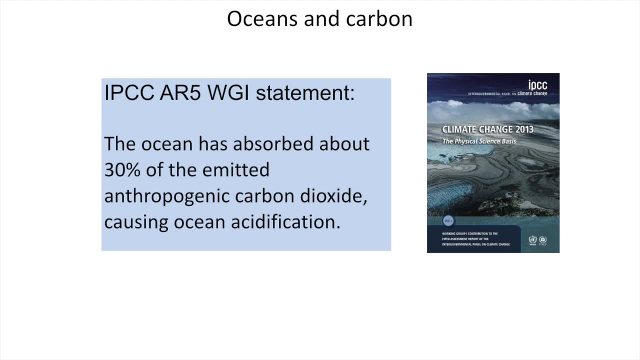 part of these parts of it In carbon, just one or two slides, Heat and ice, just a little bit Sea level rise and the water cycle. So a statement from the IPCC: The ocean has absorbed about 30% of the. 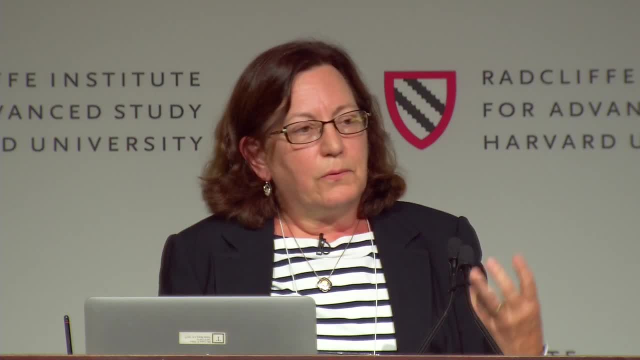 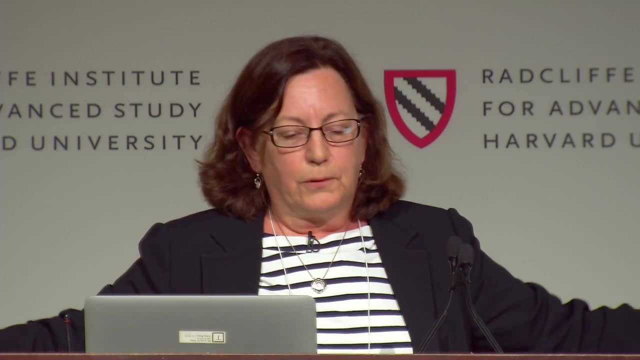 emitted anthropogenic carbon dioxide. Okay, that's an important number. You put a certain amount of carbon up in the ocean. You burn it. It's coming from fossil fuel burning: 8% land. 92% fossil fuel- Fossil fuel burning. into the atmosphere, A third stays up there, A third goes into fertilizing the land And a third goes into the ocean. And the ocean is not going to sit there and soak up the next 40,, 50,, 60%. This is an 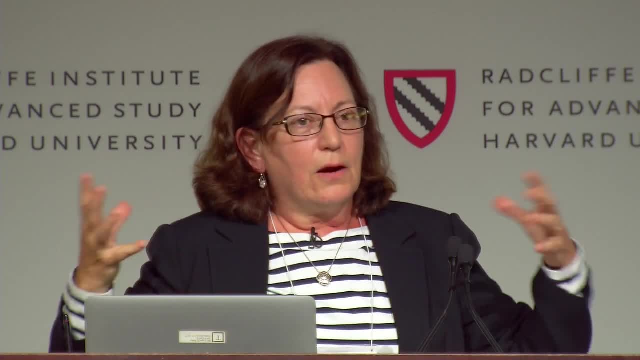 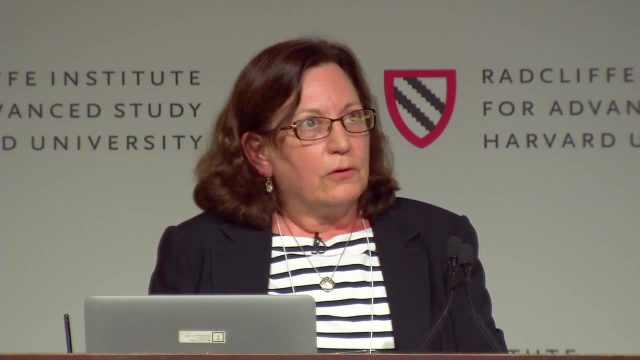 equilibrated sort of system. And once it's there, it's there. Maureen showed a nice graph showing that we're in a commitment phase. You put the CO2 in the atmosphere. it's not going anywhere. A third goes in the ocean of the part. 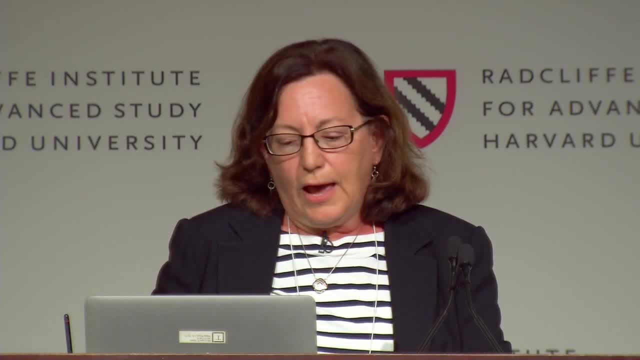 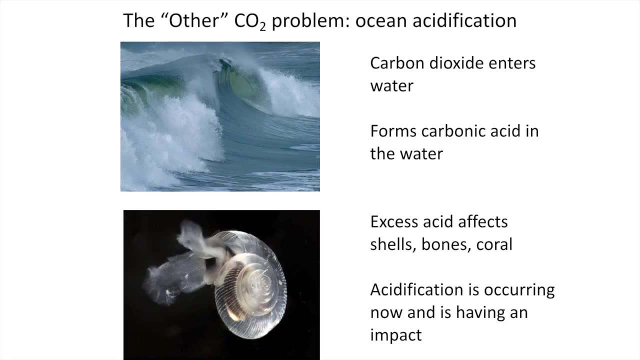 that goes up. How do you get it out? Well, you have to stop burning it to keep it flat, and then maybe you need to start removing it. Here's the other CO2 problem. The ocean is 70% of the Earth's surface. That. 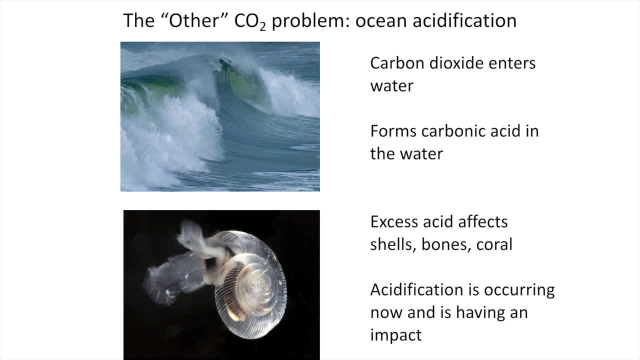 CO2, 30% that goes into the ocean. it's not a garbage dump that you just put in the backyard. It goes in and affects the marine life. So you get acidification. Carbonic acid is formed when you dissolve CO2 into water A little bit. 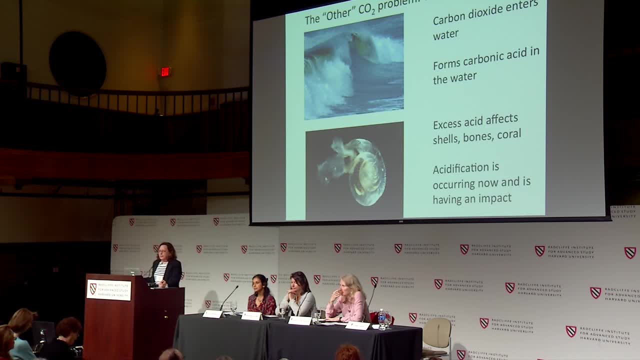 A little bit changes the pH And that excess acid has important impacts on organisms And there's a terrapod. They're kind of in danger. They have beautiful movies of them. I didn't bring any animations Flittering around The poor. 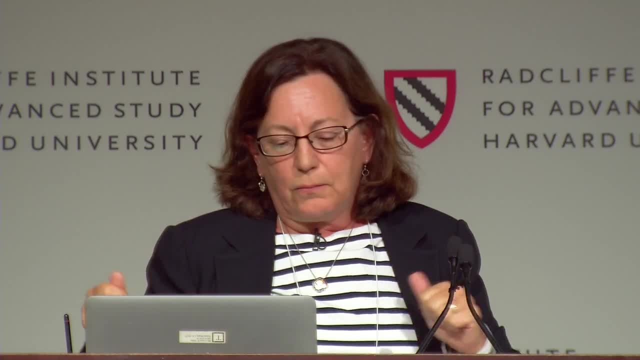 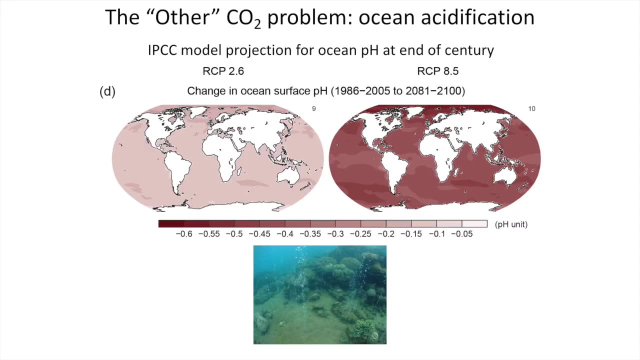 terrapods, Anyway, coral reefs, etc. You may read about all these things, And this is going on now, And so there are projections of how the surface pH will change in the ocean and also how the under-saturation, how. 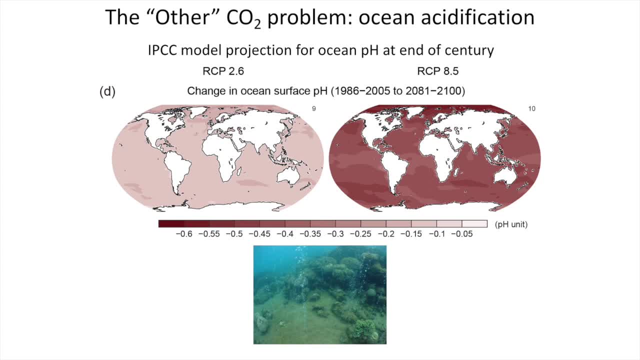 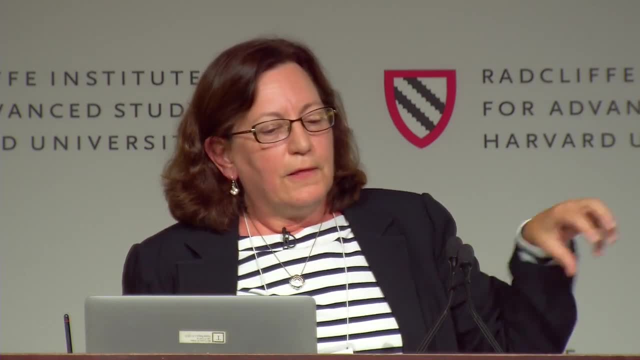 much acidification is impacting the organisms. That's it for carbon. That's an important second part of the carbon problem- if you haven't been kind of cued into it before, though, But the oceans are affected by the extra carbon as well. Now we go to heat. 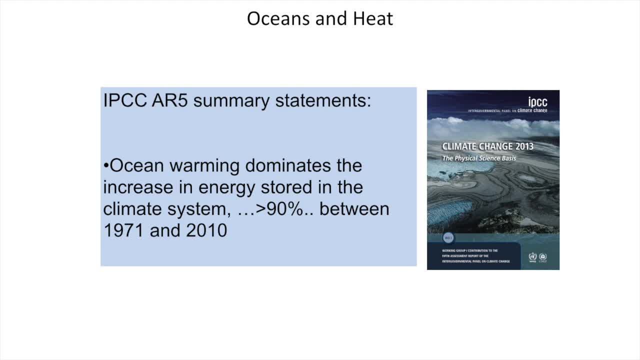 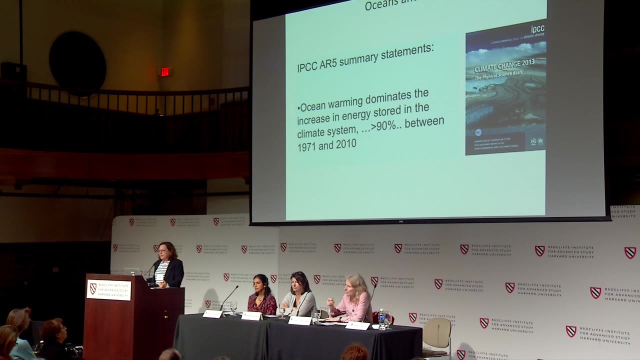 Okay, So you've heard this number already- That the excess energy in the system due to anthropogenic forcing. So this is the excess, not just the heat, but the excess is more than 90% of what's in there. So, yay, The ocean is. 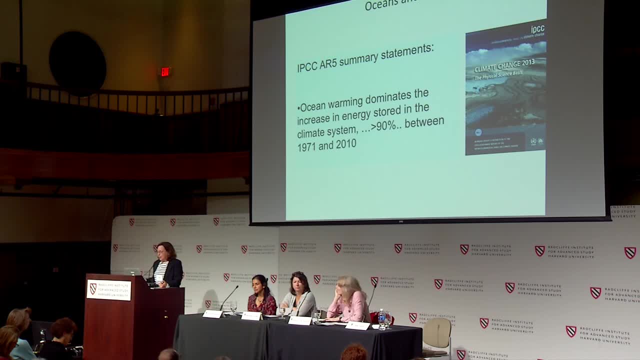 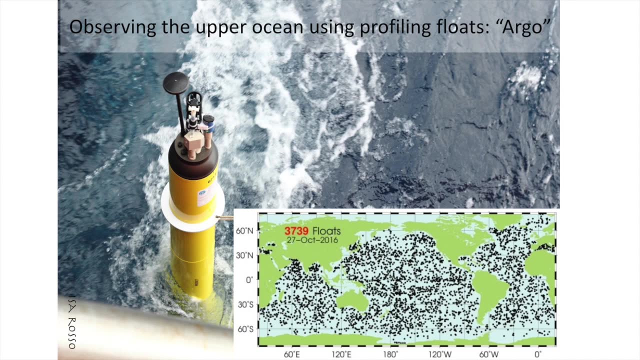 really helping us out. If that were in the atmosphere, think of how warm we would be, And I'll show a graph. How do we know these things? So this is where we get to what I do. We go out to sea and make measurements. 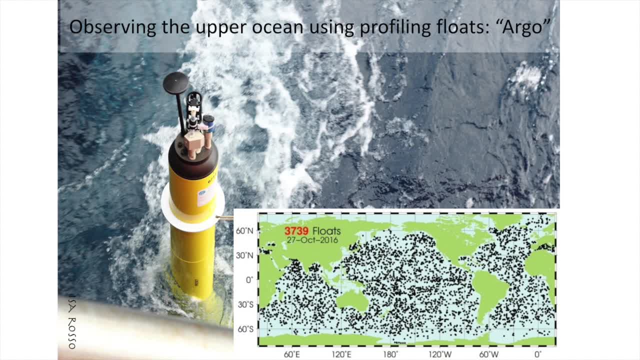 How do we know where the heat is? We measure it. This is the latest- yesterday's- maybe today yesterday- map of where we have had ocean temperature and salinity profiles over the last month. So we have a global network now. It's been a phenomenal. 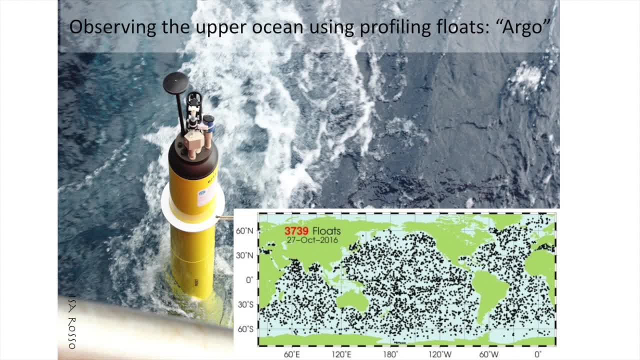 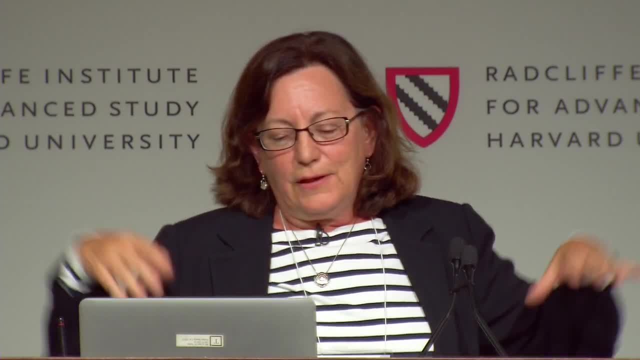 community international effort. Technology was invented at Scripps by Russ Davis. Dean Remick at Scripps been instrumental in taking this to the world, Taking the instruments to the world. These are: this is our network for the ocean. It's the upper 2,000. 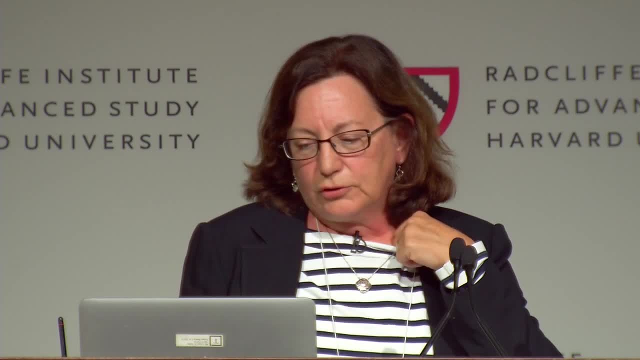 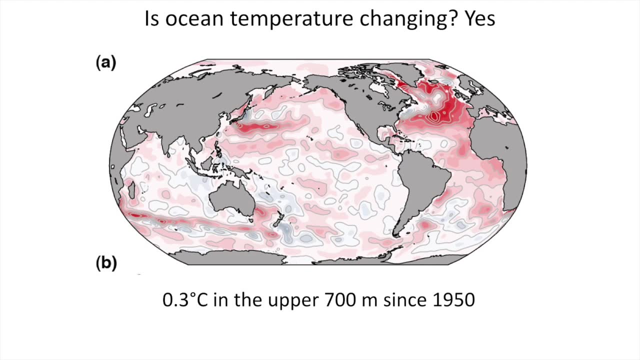 meters of the ocean. That's a picture of a float that we were putting out off of a ship in the Indian Ocean last year. Here's what you get from it. Is the ocean temperature changing? Yeah, it is. This is the change in heat. 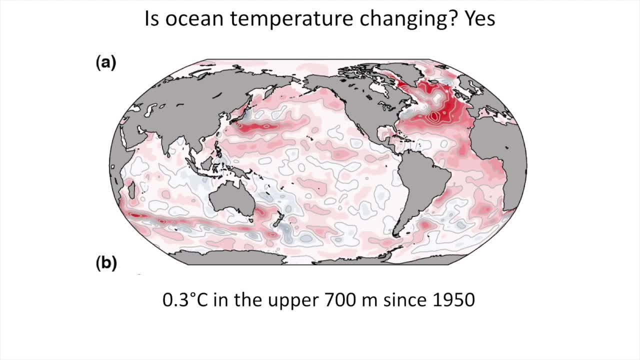 content of the upper part of the ocean: 700 meters times 3.. 2,000 feet Since 1950. Mostly red, Oh, okay, And then there's a lot of really interesting structure to it that we could spend days and months discussing. 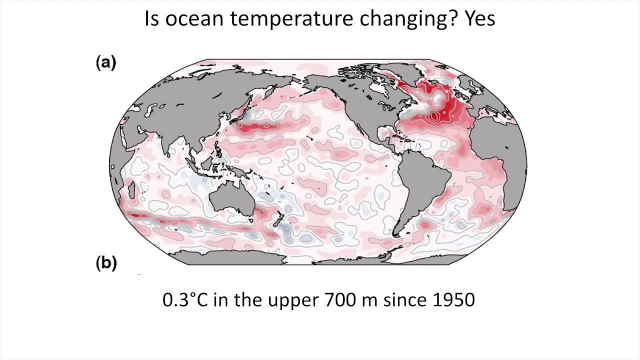 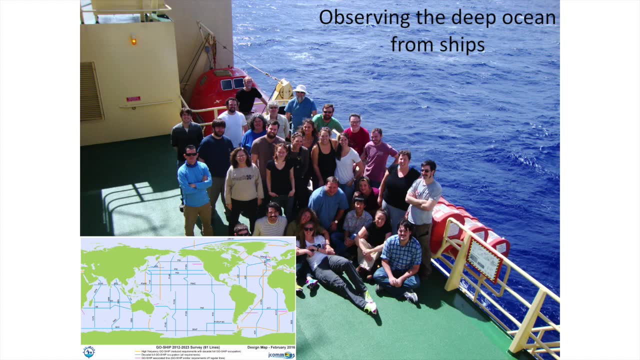 But it's mostly red. It's pretty patchy because we're using measurements since 1950.. So it's ship measurements in addition to these floats. And then I'm in the middle of that one. We go out to sea and we measure. 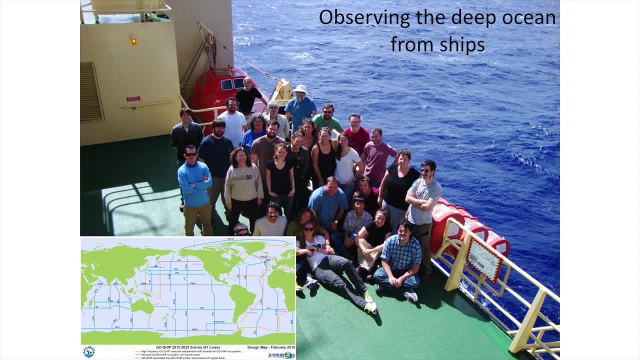 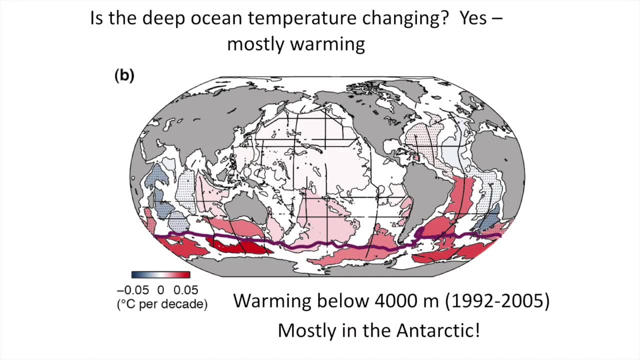 to get the rest of the ocean, to the bottom to see how it's changing over the decades, And we make extremely accurate measurements. And here's a map from Sarah Perkey and Greg Johnson: How to make your thesis become a classic. You get 10,000 citations. 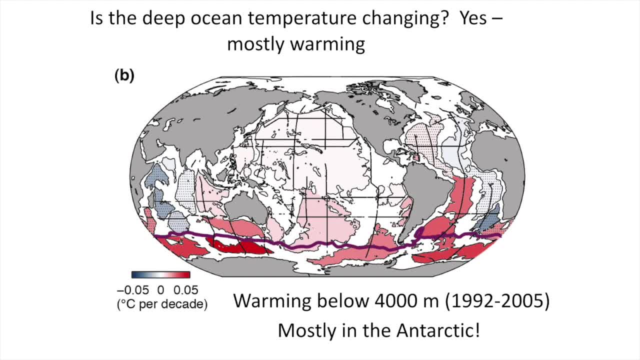 This is the map. This is using our very precise, very accurate- not precise, but very accurate- deep measurements to look at where the warming's happening below 4,000 meters And you see it's a very different pattern. This is a big eye opener. It's very much in the 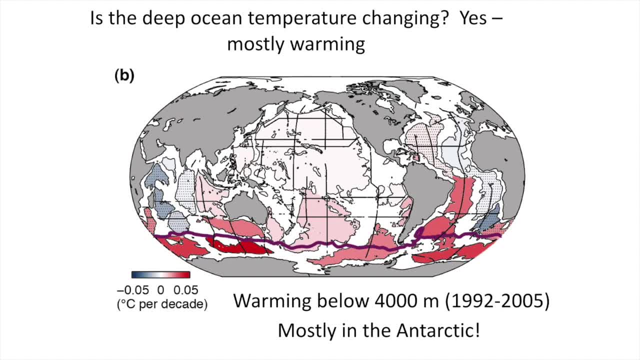 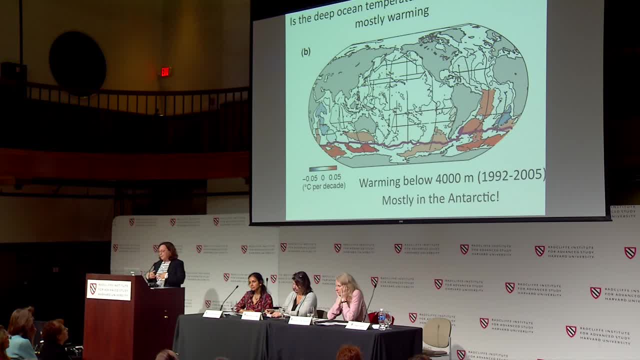 south, And this is where deep water forms around Antarctica and goes to the bottom And the balance is changing And essentially, the deep water is changing in properties. There's less of it And that makes the deep ocean warm, So we have a lot of interesting. 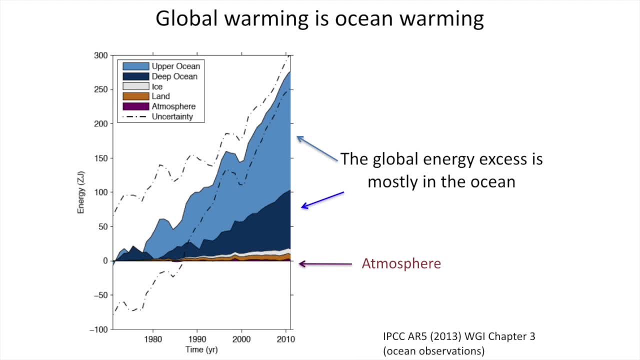 observations. a lot of interesting things to think about. This is our take home graph on warming. There's the title Global warming is ocean warming And there's our let's see. is there a pointer here? Yes, there's a pointer. I'm going to show this. 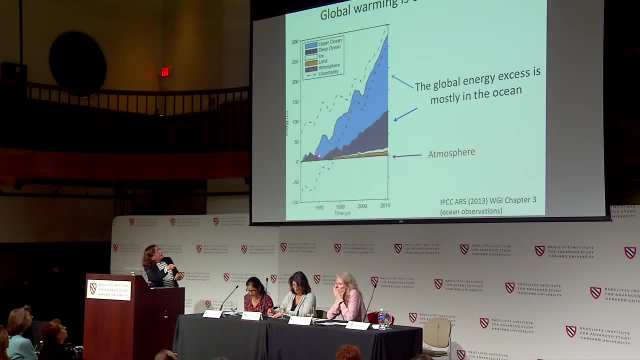 Here we go. Okay, This is the total heat in the whole system, Everything. So this is not called just anthropogenic, This is it. There's some funny units over here, Zeta Joules. This is years since we've had enough measurements to do this. 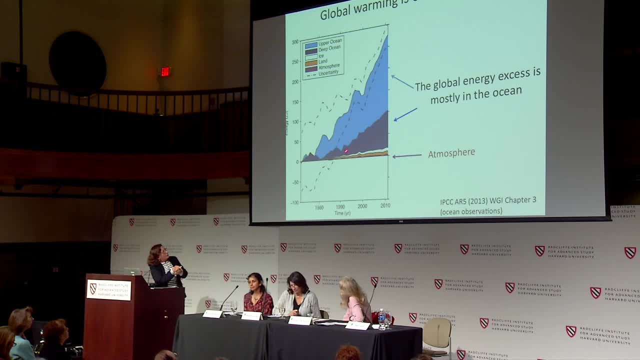 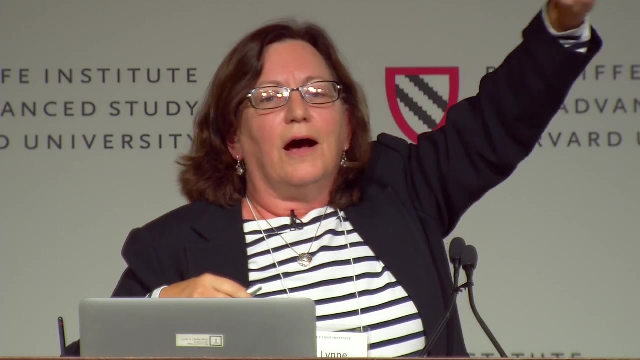 There's the total And, okay, down here there's a little tiny purple line. That's the atmosphere, That's how much the atmosphere is warm. So there was huge press about the hiatus. I bet you've heard of the hiatus out there. There's. 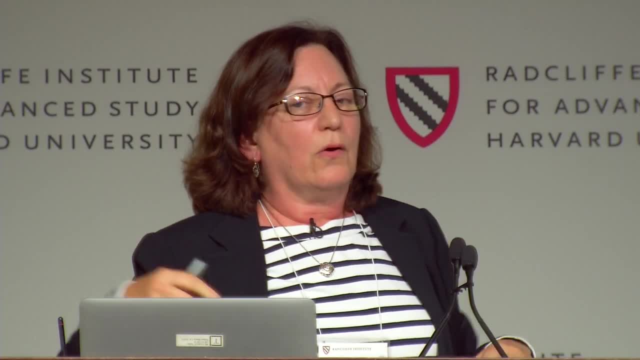 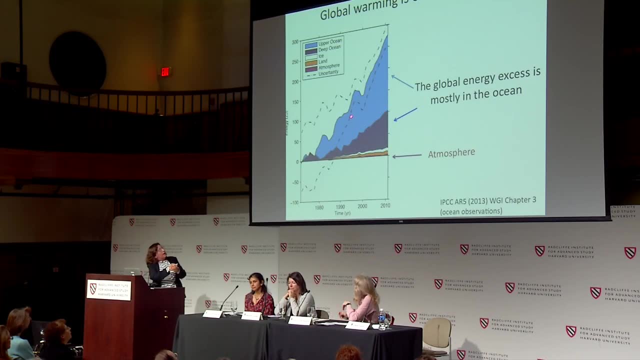 a lot of skepticism. Well, the skeptics could say, oh there's, you know, the climate is not changing Because look, it's flat for the last 10 years. Well, that was flat in this curve down here. Is it flat in that one? 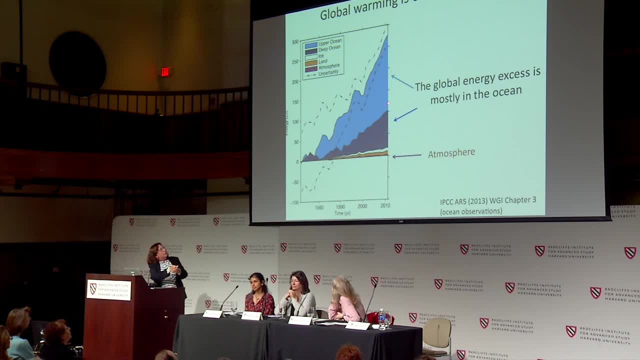 Oh no, What is this? This is the upper ocean, The upper 700 meters of the ocean. This is the deep ocean below 700 meters. You see, this is the 93% we're talking about. There's bumps and wiggles. Yes, there's climate. 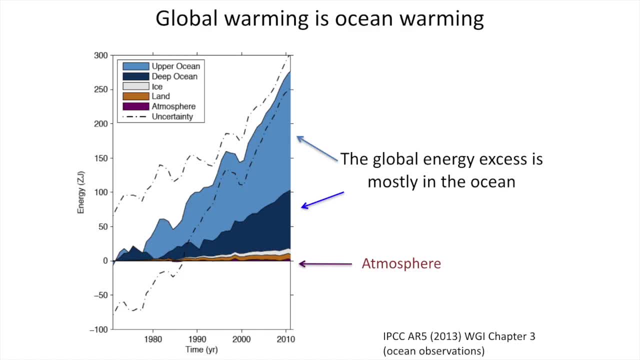 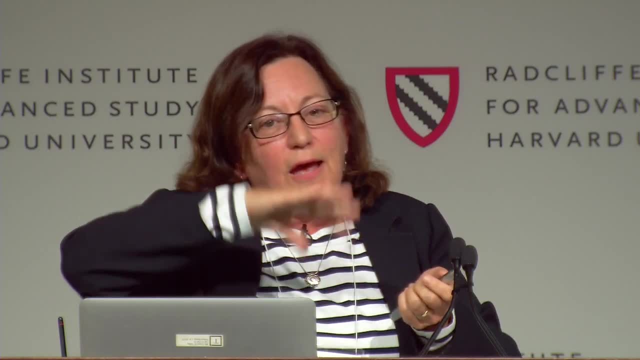 variability, But there's a relentless upward swing there And most of the heat's in the ocean, Thank goodness. But it also means that's what's happening when we have these bumps and wiggles in our surface, temperature hiatus etc. And what's happening. 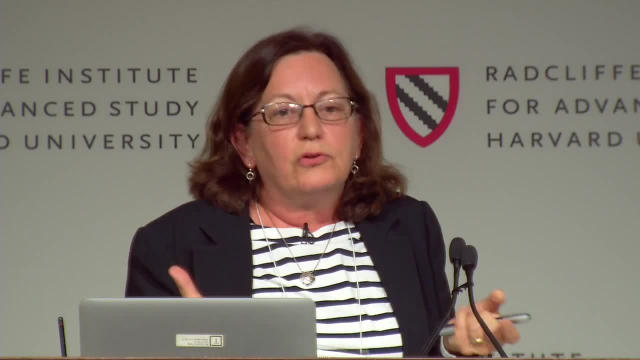 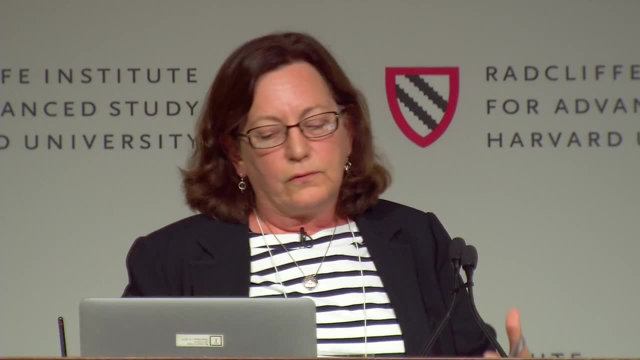 is there's an exchange between the ocean and the atmosphere. The ocean is sitting there, going, yeah, okay, let's have a mode And let's take up some heat and change the temperature at the surface, But the heat in the whole system is going up. 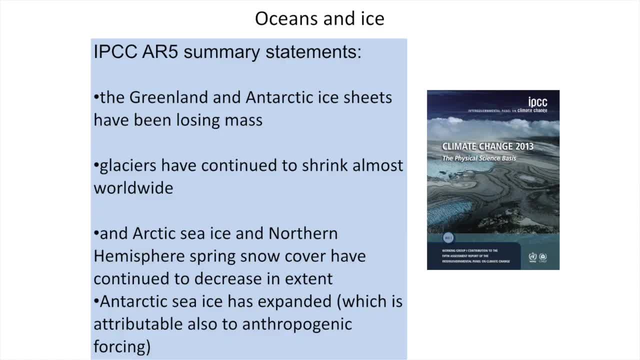 What's this doing? Overall, the heating of the whole system is the ice. The Greenland and Antarctic ice sheets are losing mass, Glaciers are continuing to shrink worldwide. That's not the ocean, so I'm not showing it- Arctic sea ice, etc. 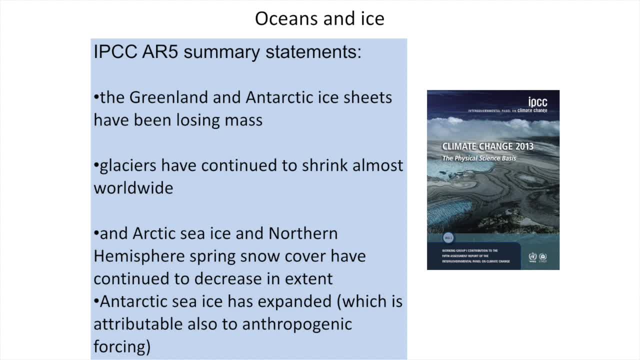 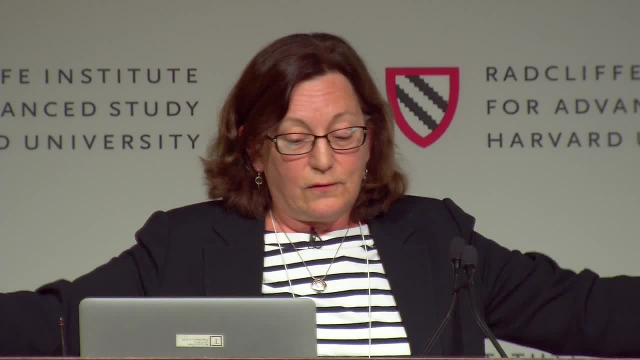 And the Antarctic sea ice has expanded, which is a very interesting topic, And there's workshops going on about that. That's attributable to the largest extent is in the winter, when there's no ice albedo feedback. It's dark down there And the wind is blowing. 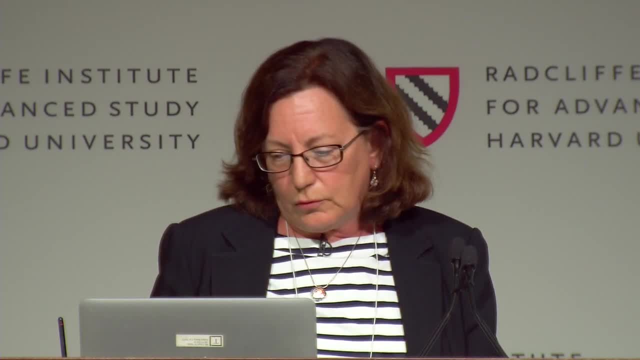 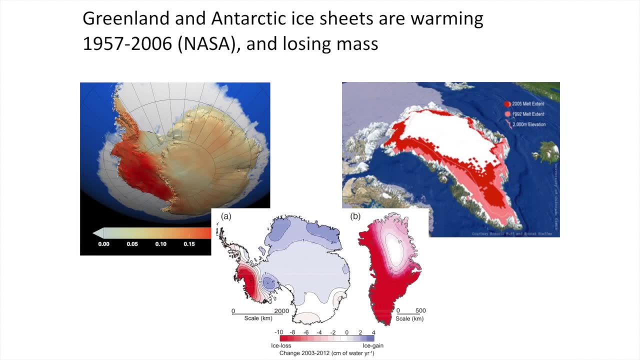 stronger because of global warming, And the wind pushes the ice out, So the cover is going up. We've already seen these great pictures of the Arctic ice. Here's the ice sheet warming. This is Greenland, where it's warming and losing mass. 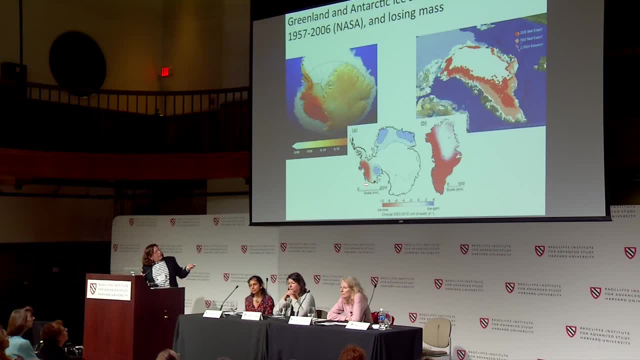 There's the mass loss. This is Antarctica, where it's warming. Here's the mass loss. You know it's not the whole thing. so, yeah, we're going to be kind of happy with only how many meters was that? 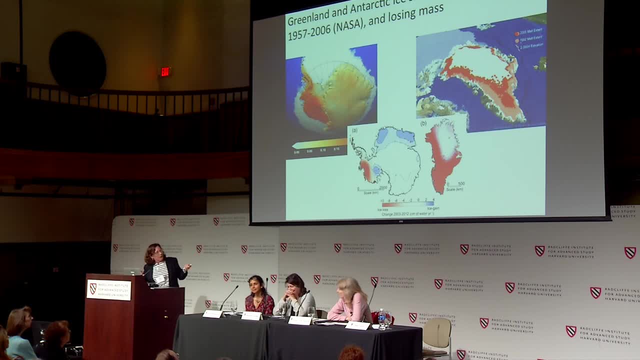 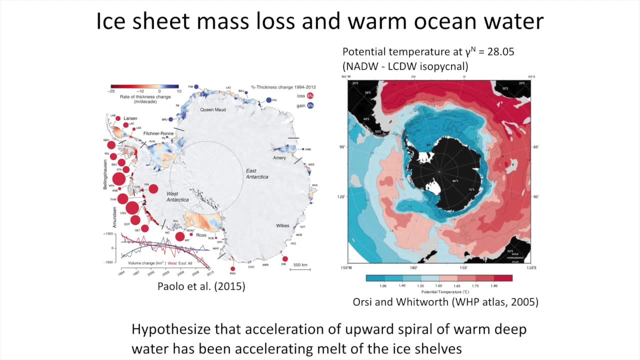 Six meters as opposed to 180.. Six meters of ice loss. As an oceanographer, we're interested in this. You've already seen from Rebecca and from Maureen how the ocean affects the ice balance. This is in the Antarctic. This is the Antarctic ice sheet. This is 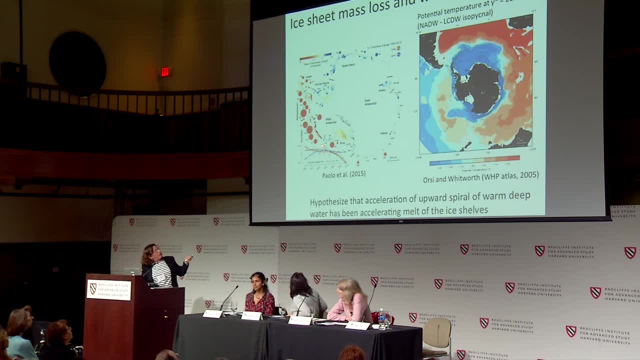 the ice, increased ice loss from the Antarctic ice shelves, And the ocean is a part of the culprit. It's not just the atmospheric temperature. The ocean is wrapping warm water coming out of the North Atlantic spiraling upwards towards Antarctica- Guess where it hits. 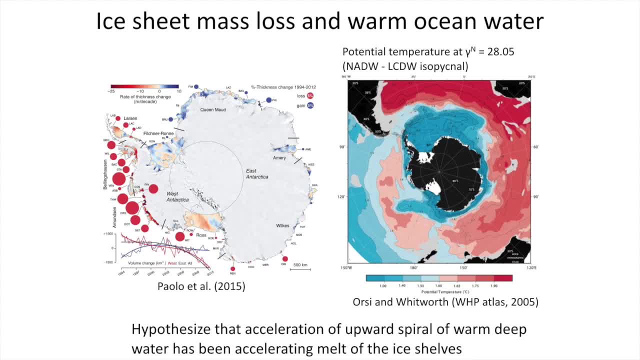 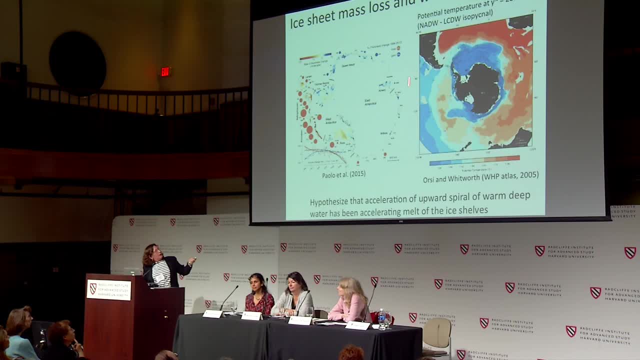 X marks a spot Over here, So this is where it spirals in very close to Antarctica, And we're working hard on quantifying that in models. How much of this ice loss is due to accelerations of this pathway of warm water to the surface? 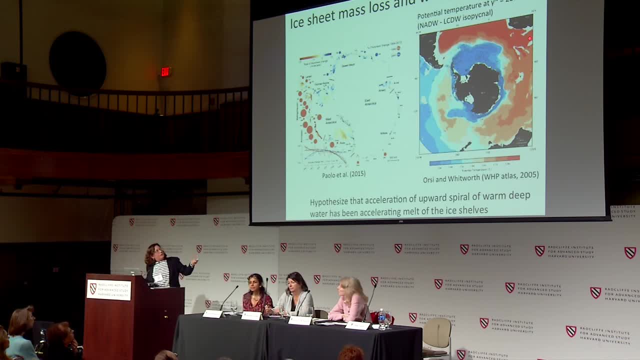 So you don't see the third dimension here. It's going from 3,000 meters deep up to 200 meters. This is the mean state. This is the way the ocean is set up. So this is the incursion of warm water. 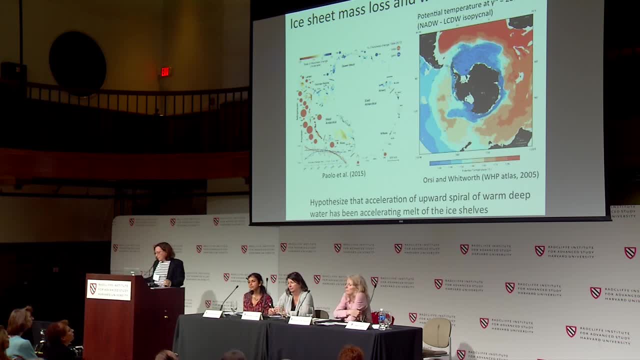 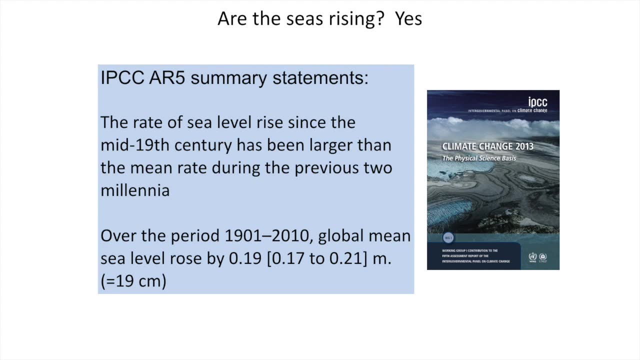 And changes in that, probably due to winds, may increase this mass loss over here. Are the seas rising? Yes, you've already seen that they are. Here's the IPC summary Rate of sea level rise has been larger than the mean rate during the previous. 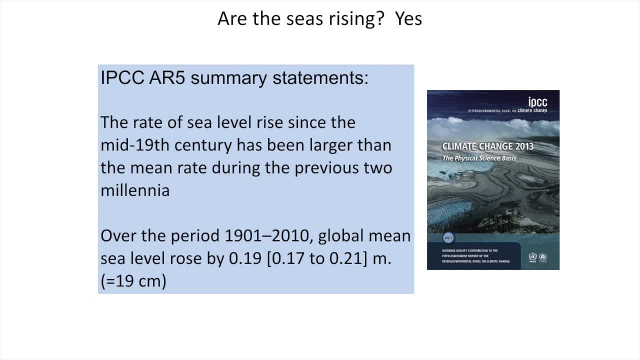 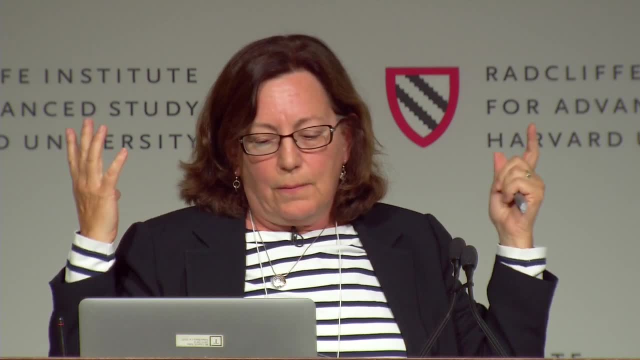 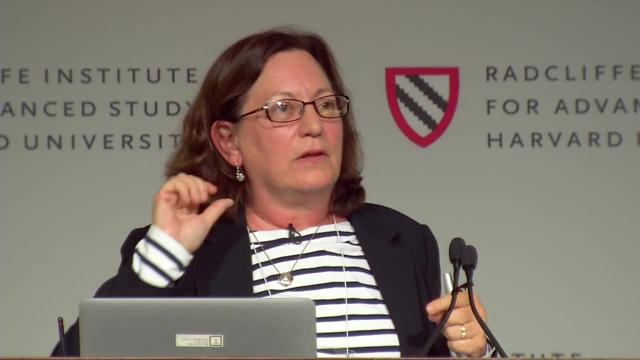 two millennia It's gone up 20 centimeters. Well, 20 centimeters, that's not very much. Go home, sleep well. Who cares? Oh well, with that 20 centimeters also comes an increase in the and the more storminess. Storm surges go up. There's a change in. there's actually different rates for different parts of the tide. That aside, well, let's say: well, the most important thing about that 20 centimeters is that it's relentless. So I'll show you a graph in two. 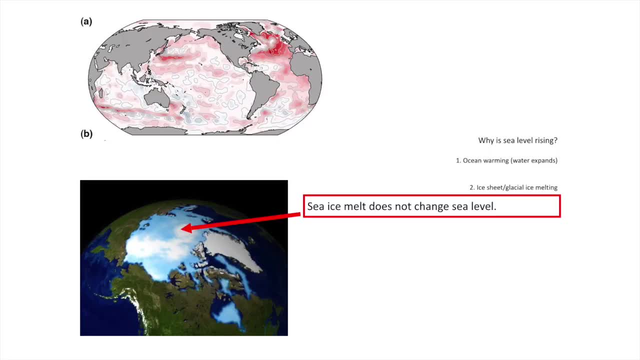 First, I want to just give you a little pedagogy here on why sea level goes up. It goes up for three reasons: The ocean warms, so it expands. Okay, that's all that heat there. Number two: ice sheets, land-based. 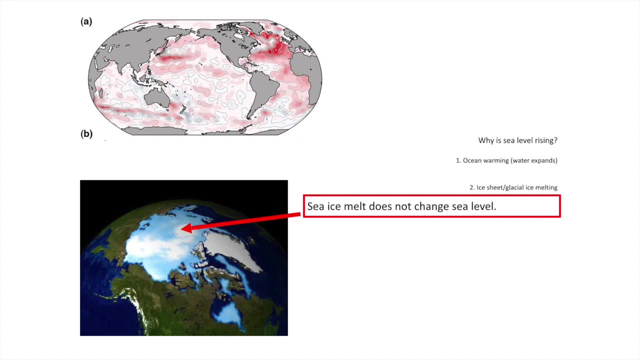 ice melt, Not sea ice. Sea ice is like ice cubes in your iced tea. When it melts, your iced tea doesn't overflow, But when the ice sheet melts, it does fill up. So you're adding water to the ocean from glaciers. 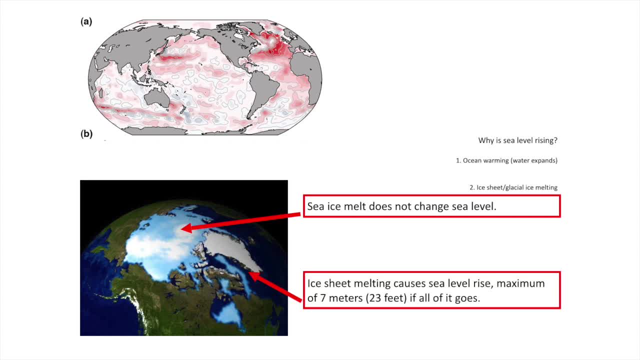 and ice sheets. So the sea ice melt doesn't change it, but the ice sheet melt, the shelf melting, the ice sheet melting does. Those are two big factors. The third big factor in the change in sea level is rebound over thousands of years. You can go on this. 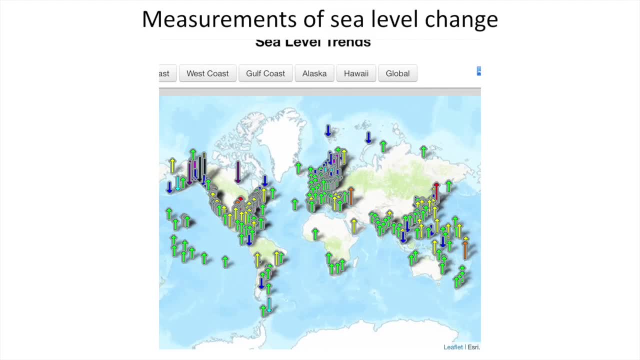 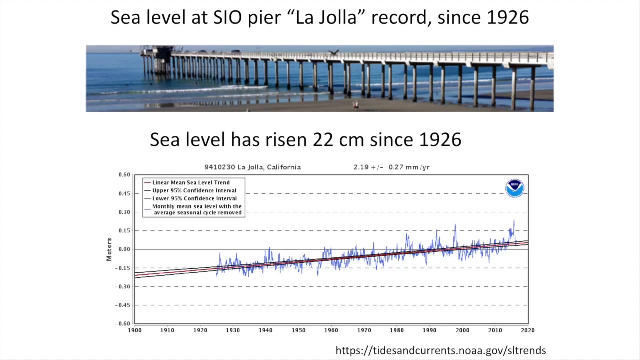 wonderful NOAA website and find information from all the long tide gauges around the coastlines and you see a pattern, mostly up arrows. and these are from the tide gauges, some of our favorite ones. The down ones may be the rebound. Here's La Jolla. 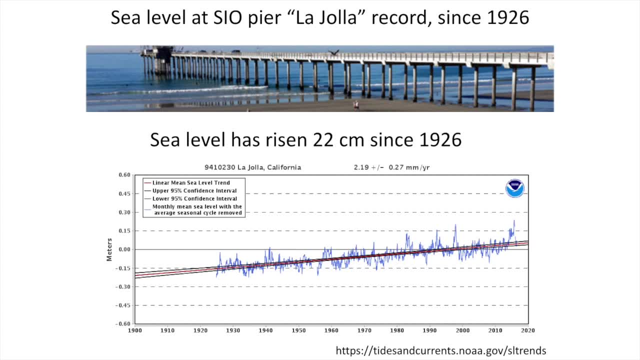 We just celebrated 100 years of La Jolla records. It's out at the end of the world. People are out there every single day making manual measurements of temperature and salinity. There's an automated tide gauge out there. 100 years is 100 years. 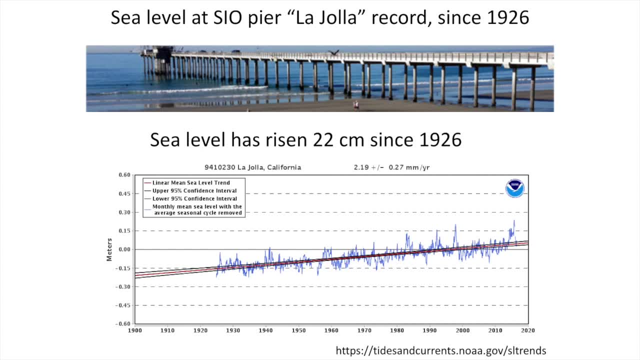 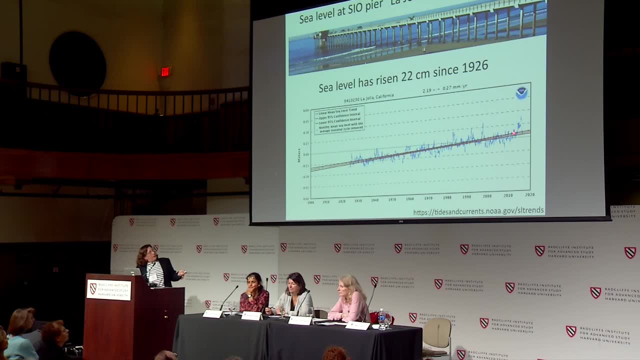 enough was the question that was posed. Well, should we stop? No, Don't stop, Because here's the record: Relentlessly fit a line through it, relentlessly going up lots of bumps and wiggles. And if you only have 20, 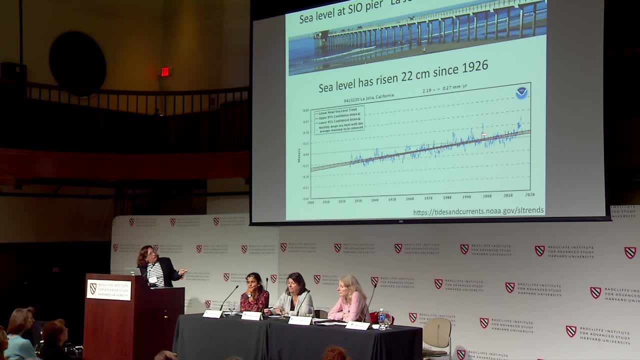 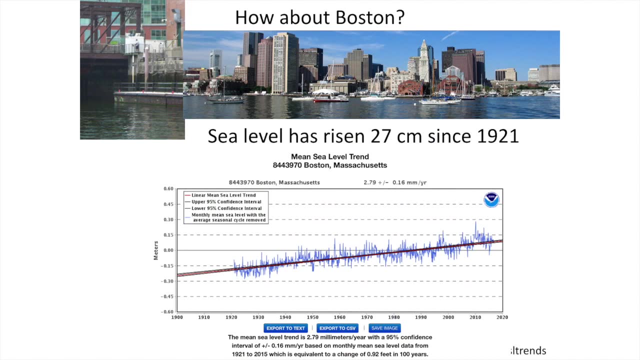 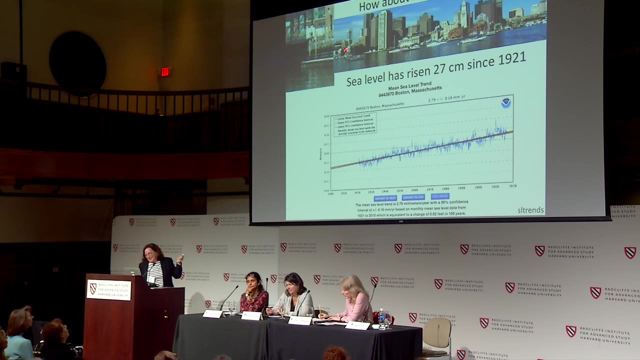 years, or you stop. what do you know? You've got to keep measuring it. So this tide gauge goes up relentlessly. Let's move over to Boston. What's going on here? Ooh, same answer: 1921.. Out there in the Boston harbor. 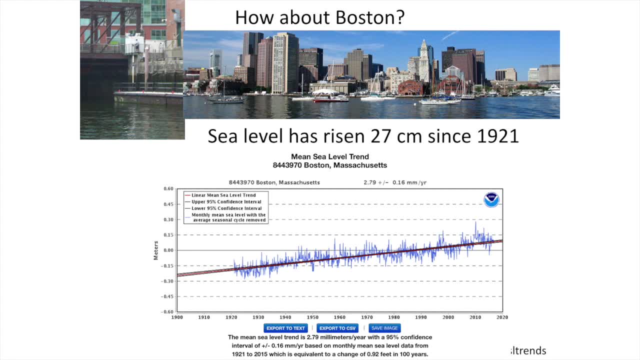 in this kind of very picturesque corner is the Boston tide gauge that's been there since 1921, maintained by the Coast Guard, And the same kind of picture- Bumps and wiggles and a line fit through it, going up relentlessly. You can make a map. 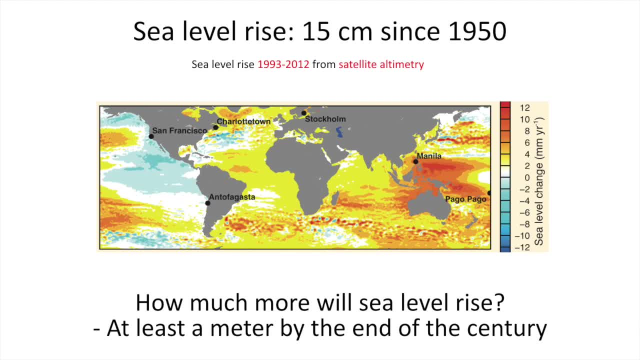 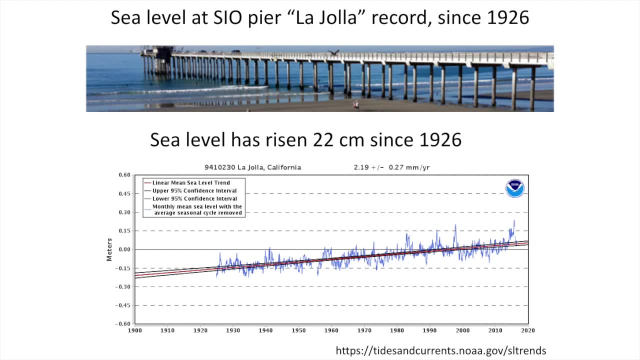 This map doesn't look like it's going up relentlessly, It's going down. This is only since 1993.. If you went back to these things and started in 1993, you might see sea level going down. So you're seeing natural modes of variability. 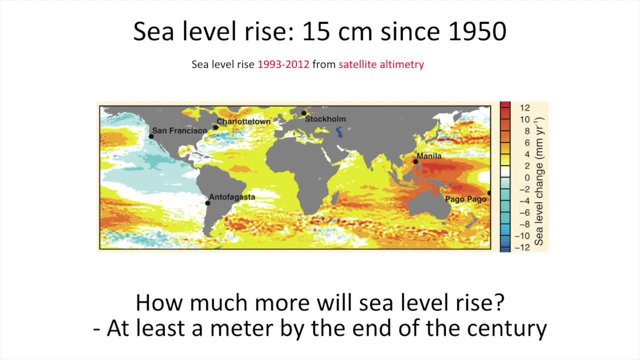 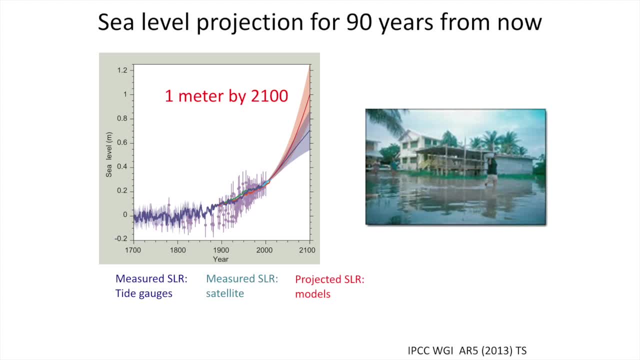 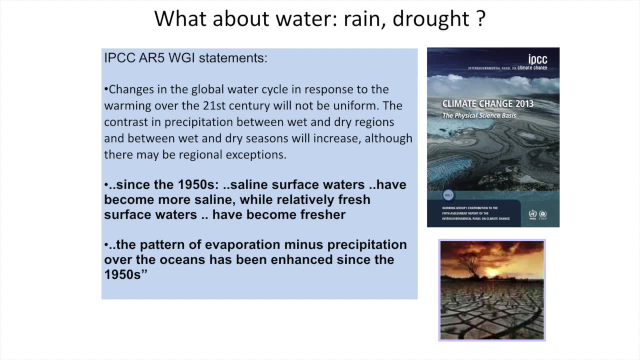 superimposed on relentless sea level rise, So the idea is that it keeps going up. Here's the projections: It should be up by at least a meter by the end of the century. Okay, so, last but not least, that's sea level. 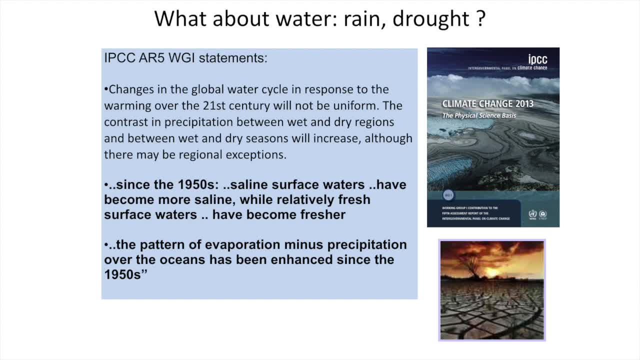 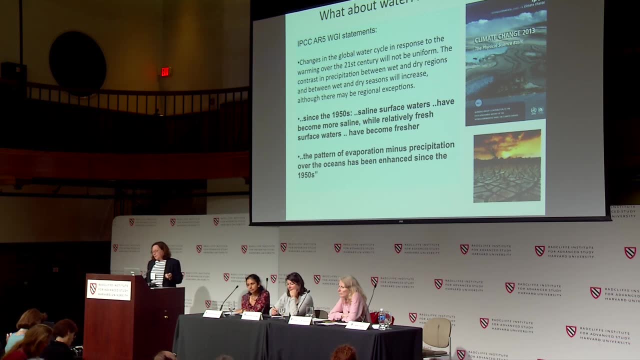 Just going to come up. What about our rain? What about our drought? What about the things that matter to agriculture? What about the things that matter to populations in arid areas? Okay, so what we're going to be able to see here? 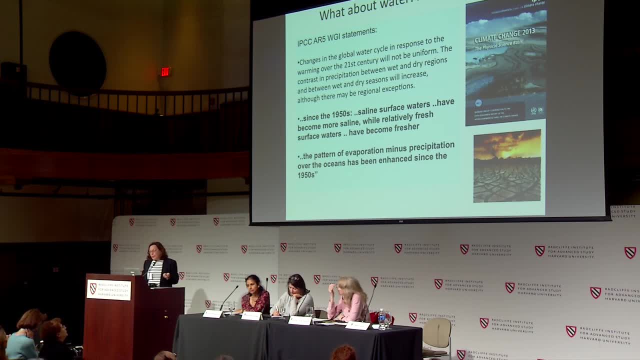 is that the ocean salinity is acting as a global rain gauge, which is great. We can actually learn a lot from ocean measurements that we can't from just rain gauges on land. What we found to summarize and then go through: why is that? since the 50s? 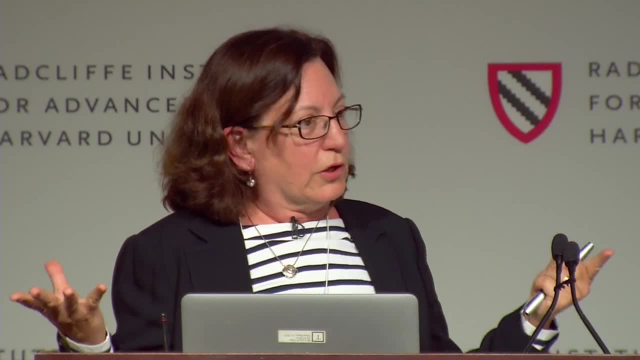 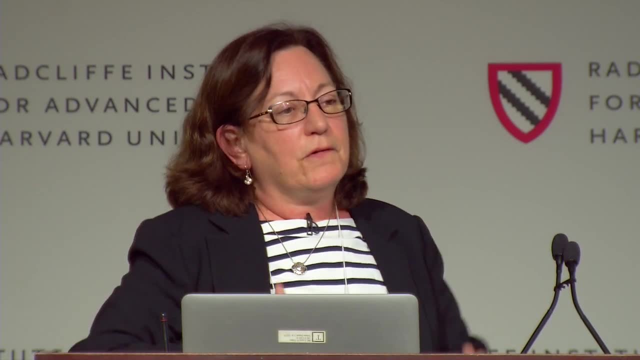 where the surface waters are salty- saltiest, they've gotten saltier. Where they're fresher, they've gotten fresher. That means we've changed the amount of evaporation and precipitation. It's doing more of both. So places that are evaporating. 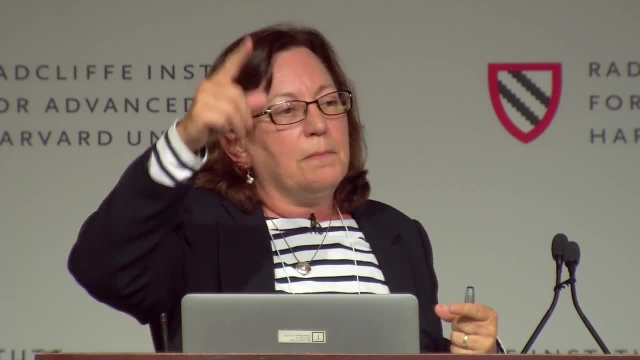 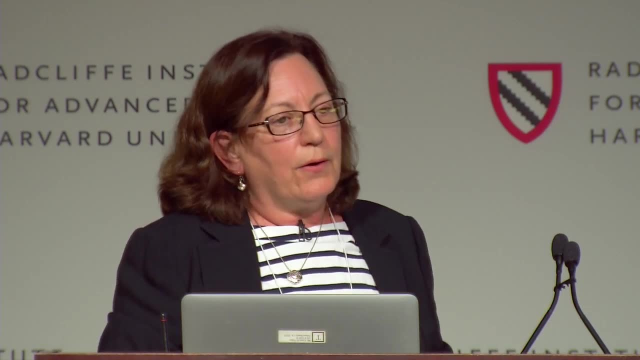 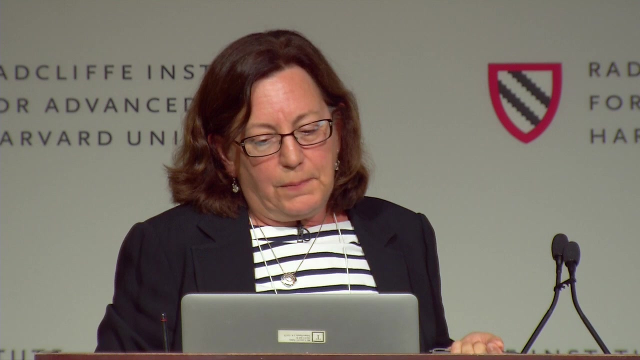 are evaporating more, Places that are raining are raining more And that means that if you extrapolate that over to land where you have arid regions, they become more arid. Where you have wet regions, they become wetter. So we have seen over the ocean. 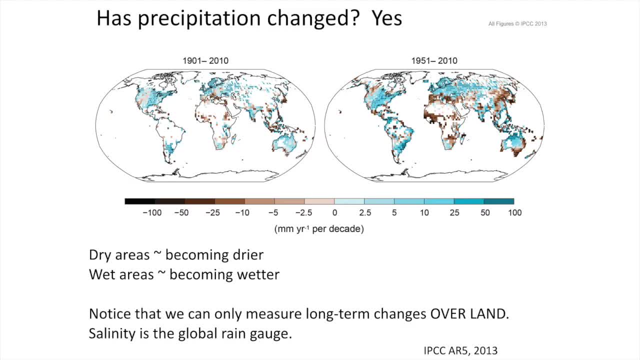 enhancement of the pattern of evaporation minus precipitation. This is some graphs from land which are showing this pattern, but will show it big time with the ocean that the dry areas are getting drier, the wet areas are getting wetter. This is rich, get richer. poor, get poorer. 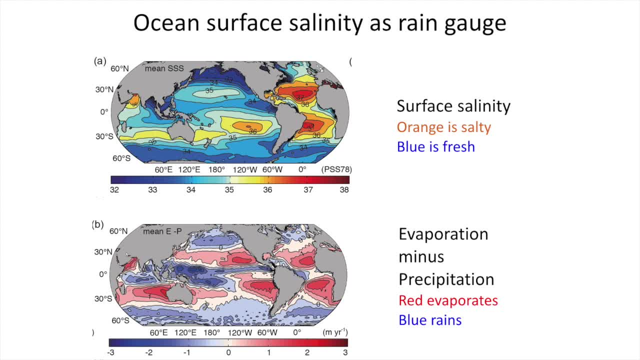 they can only measure that over the land. What we do with the ocean. these are the mean state of the ocean. the top plot is the surface salinity, maybe something you've never looked or thought about before. Where it's orange, it's high. where it's blue, it's low. 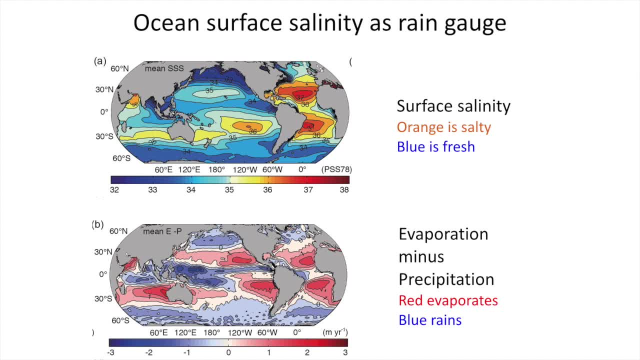 You can see the patterns in this. bottom plot is showing evaporation minus precipitation. where it's red is where there's more evaporation, where it's blue is where there's more rain And that matches up pretty well with the surface salinity pattern. These are related to each other. 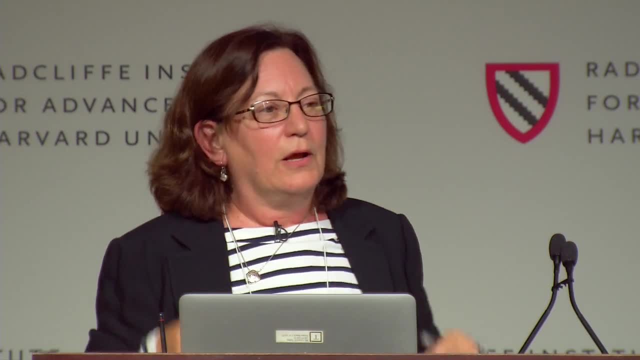 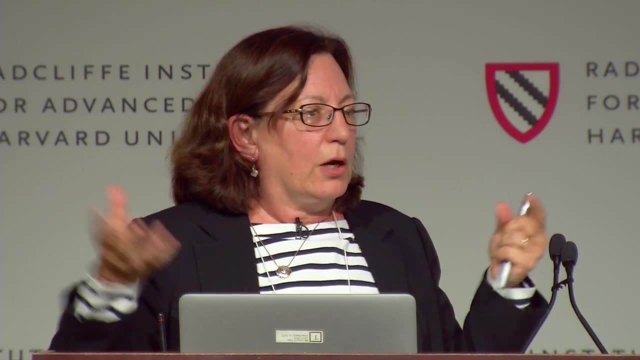 So the way you change salinity is: you add water or you subtract water, because the salt is out there. So it's the dilution. You put in more water, it'll get fresher. you take out the water, it gets saltier. So we can stack some plots. 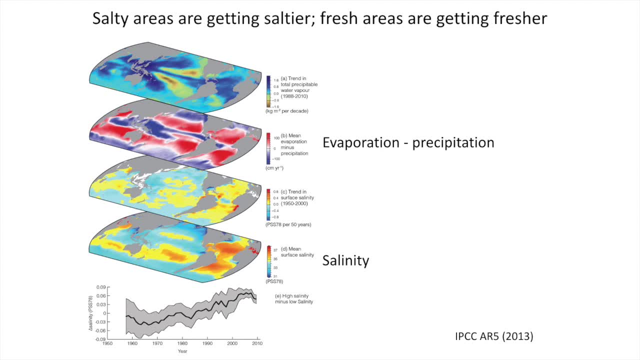 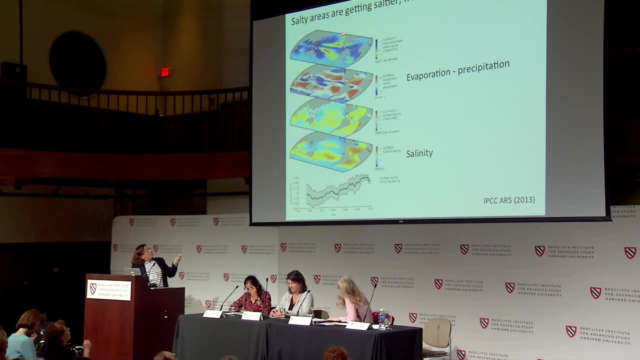 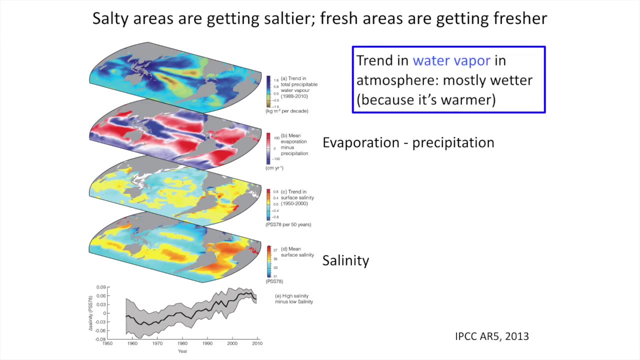 that plot of the evaporation, precipitation is here. this is a world map in the middle. this is a world map of the salinity at the sea surface and above them. I'll do the one at the top first. The one at the top is showing you the trend. 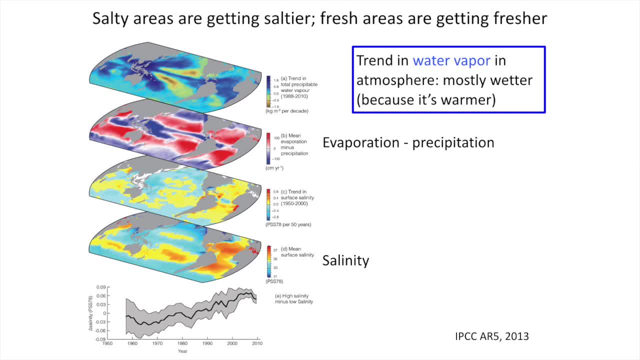 in the water vapor in the atmosphere. The whole thing that drives all this is: the atmosphere is warmer, so it can get wetter, so it's holding more moisture, so it's cranking more through because it doesn't hold a lot of water. most of the water is in the ocean. 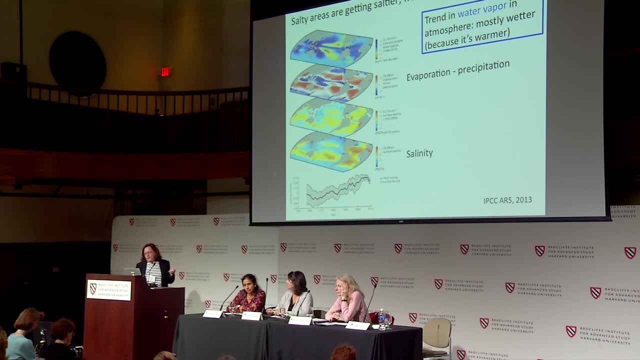 That means it's just picking it up and dumping it out. picking it up and dumping it out. So the trend in water vapor globally is to be more. There's some places that are drier. This map that's noisy, because our data is kind of noisy. 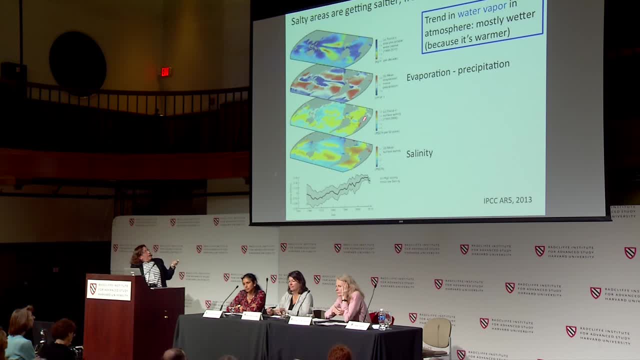 is the trend in surface salinity and it maps pretty nicely onto the actual map of surface salinity. so that's when we're saying that the salty areas are getting saltier, the fresh areas are getting fresher. in this sort of noise we have uncertainty measurements on that. 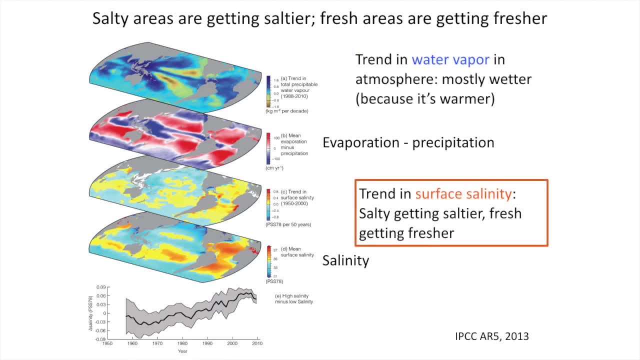 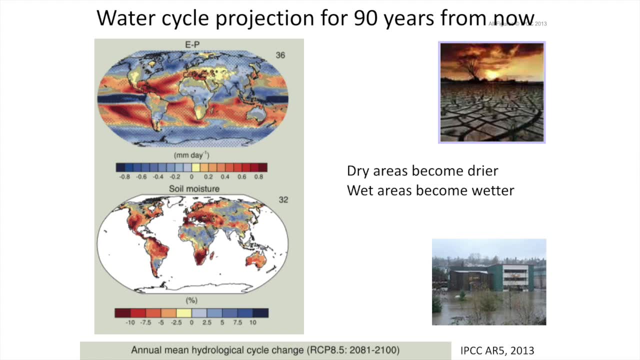 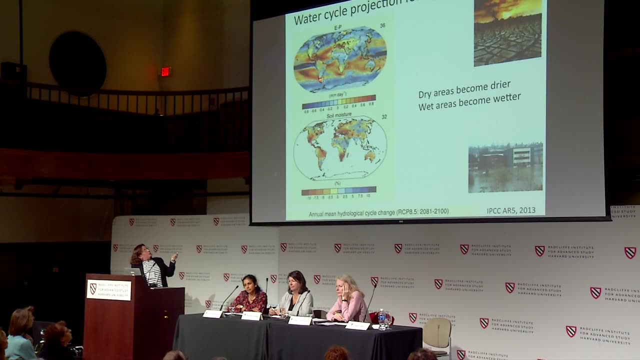 this noisy sense. So surface salinity is suggesting that globally we're having this change in the pattern. and then you can make projections up to the end of the century using all these climate models which show this pattern of change in evaporation, precipitation. so the trends look a lot like. 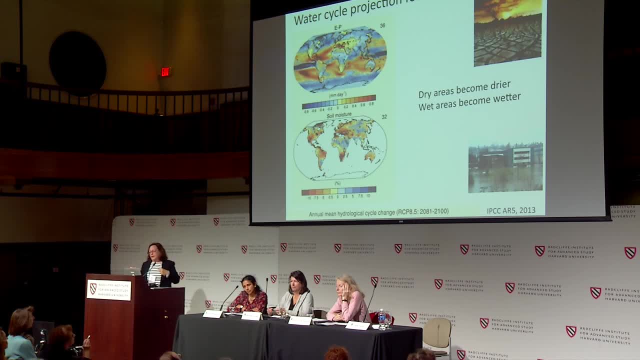 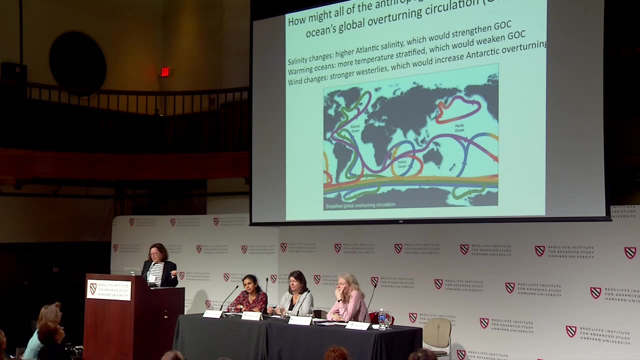 the actual situation, the actual mean state. so where it is evaporative, it becomes more evaporative, and where it's so, you get dry, and where it's wet, you get more floods. Okay, so I am behind. I'm going to skip that. just to summarize, um, climate change in the ocean. 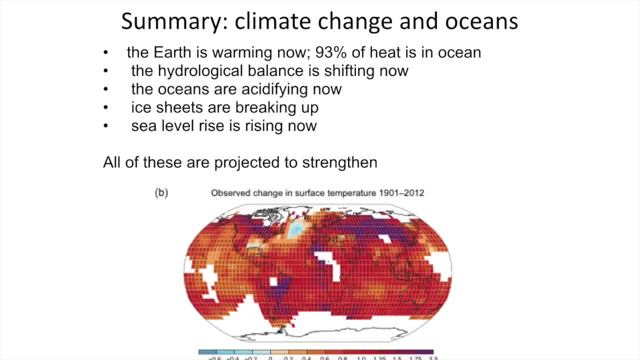 earth is warming. now 93% of the heat's gone into the ocean. hydrological balance is shifting. now it's strengthening. now oceans are acidifying, now ice sheets are breaking up and sea level rise is going on. all of these are projected to strengthen, so there is 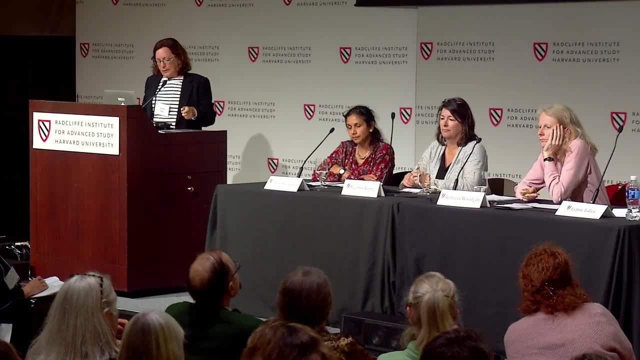 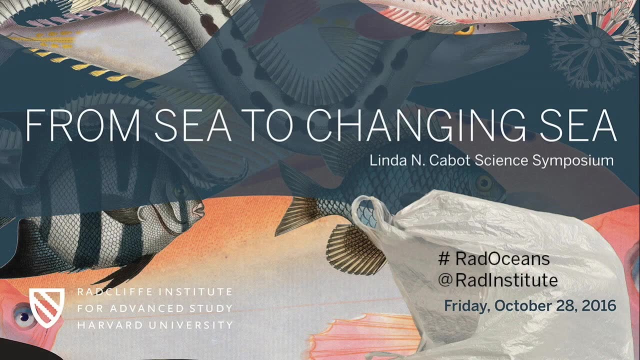 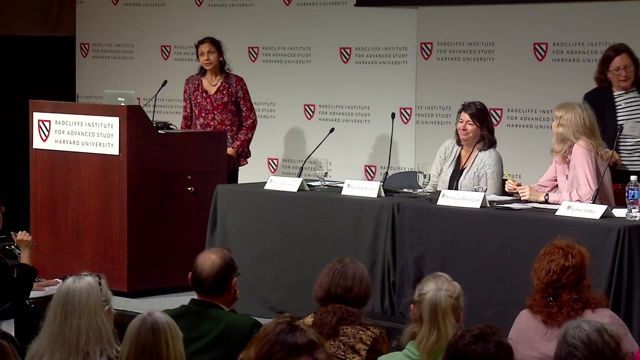 strong evidence for climate change, and I think that's all stop there. applause, applause, applause, applause. I'd like to thank the speakers and I'll start off with a few questions to the panel, and in the meantime we'll have a mic set up, so if you want to ask questions, 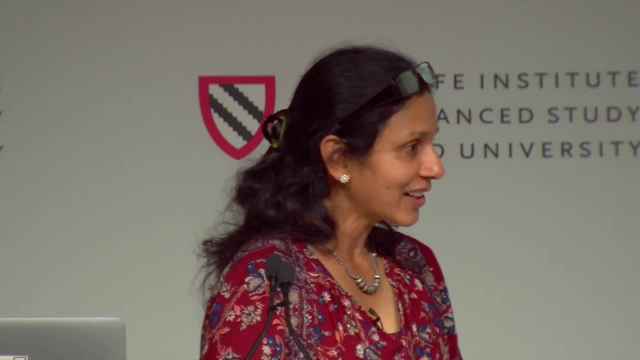 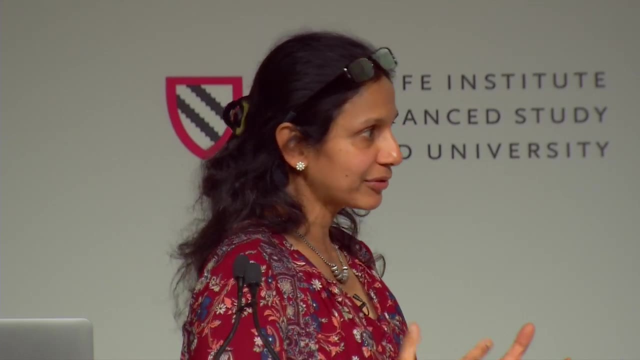 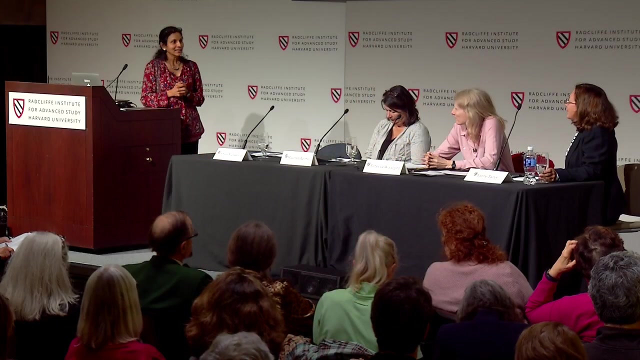 we'll go until 12.15. so let me start off by asking. maybe, Lynn and Rebecca, you know there are big differences between the two poles and how they work in making the earth's climate what it is, and one big difference is the arctic is in the ocean. 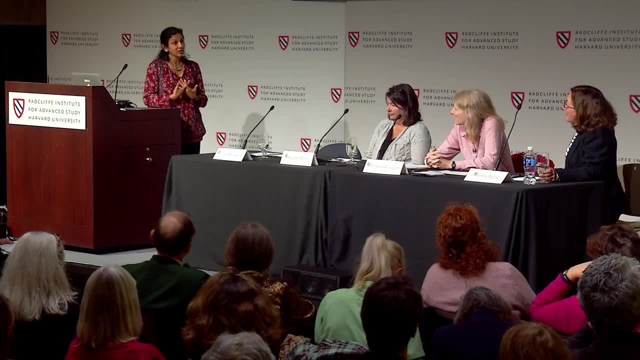 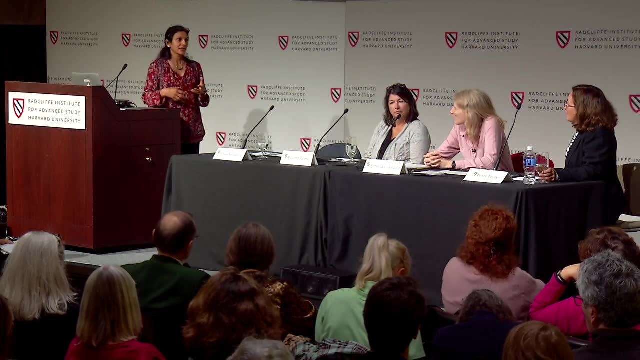 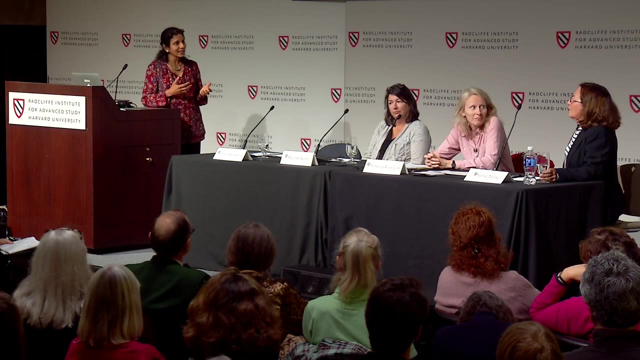 and Antarctica is land mass, but there is a circulation around Antarctica. maybe you could throw some light for us as to why the Antarctic ice sheet is not melting at the rate that sea ice is melting. and you know, during the glacial, interglacial fluctuations there was a huge change. in ice volume in the northern hemisphere, I believe, not as much in the southern hemisphere. so what are the big differences there? I think you already said it: it's inside out. so one is ocean surrounded by land and the other is land surrounded by ocean, and that just completely changes. the way they respond to the winds. both of them have wind patterns. the Antarctic ice sea ice area is out in the westerly- that's like where you live right here up through Greenland- whereas the arctic is the other direction. there's a lot of pieces to this. so one of the. there's a lot of ocean in the southern hemisphere. there's a lot of land in the northern hemisphere. that makes it a different response. there are easterly winds ringing around the arctic and the easterly winds in the Antarctic are right along the coast. 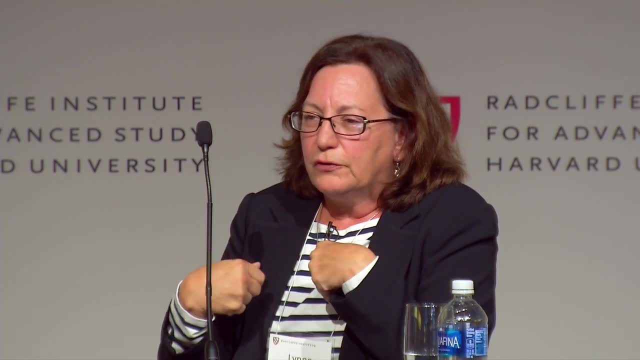 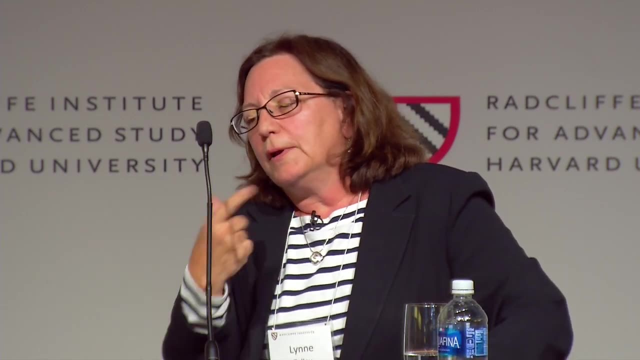 and they're really important for pushing water into the coast. but the main wind pushes the ice out from Antarctica towards where it melts. so you have this. what we're doing with global warming is spinning up those winds. they're getting stronger because the contrast and temperature are bigger. 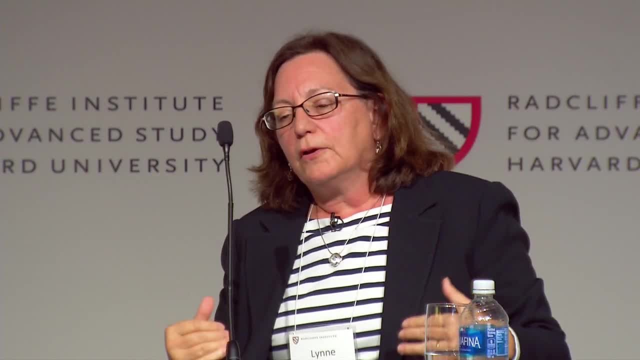 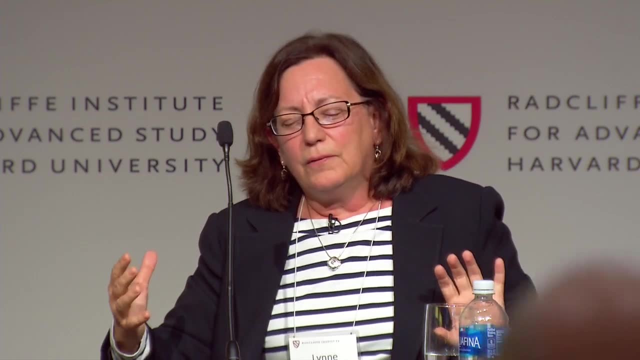 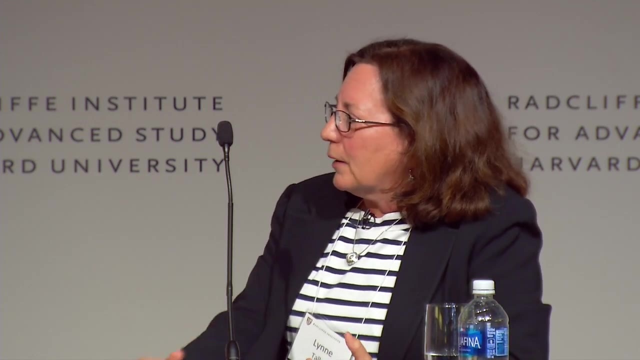 there's bigger winds and that's pushing ice out farther. so, even if the volume and so forth is a little different, the extent is getting bigger. there's more- I think that's the biggest one- in the sea- ice and the arctic is just warming. the Antarctic is only warming. 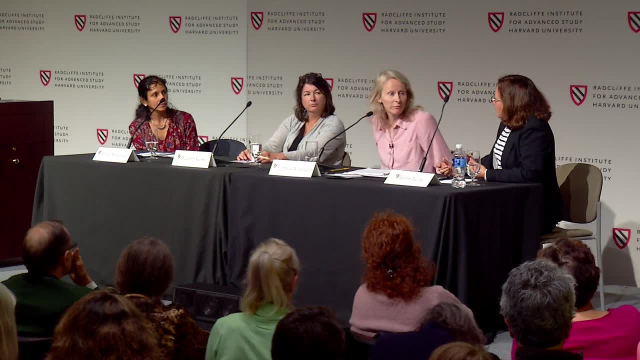 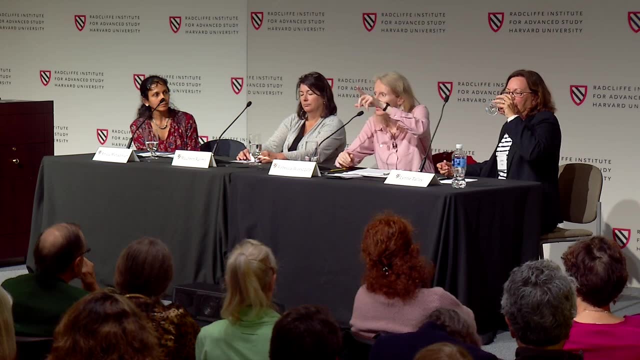 in the west Antarctic area. yeah, so I'd agree with that. basically, you've got just a very different geography which allows different things to happen. so around Antarctica we have the strongest current in the world, the Antarctic circumpolar current, which manages to isolate things down into Antarctica. in the arctic we don't have that. we have an ocean we can flow waters into from either side. the ice in the arctic is generally it's sea ice. it's thin ice. it's some meters thick. in the Antarctic it's a dirty, great big chunk of land ice. which is kilometers thick. so you have a different whole climate associated with those things. it's nice to have two poles. during the glacial was the Antarctic ice sheet much thicker, so in North America the ice that was over Boston was flowing from central Canada down to here. in Antarctica. the ice expanded, but it was only able to expand out to the end of the arctic ice shelf, which was more exposed because of the sea level drop, because of the northern hemisphere ice sheet, but then it just falls off the continent and flows away. so it really is: there's no land for it to move. 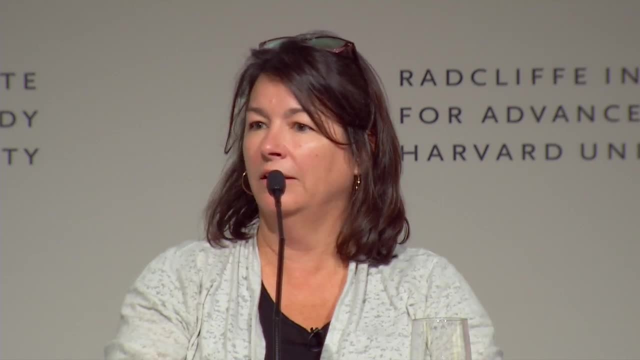 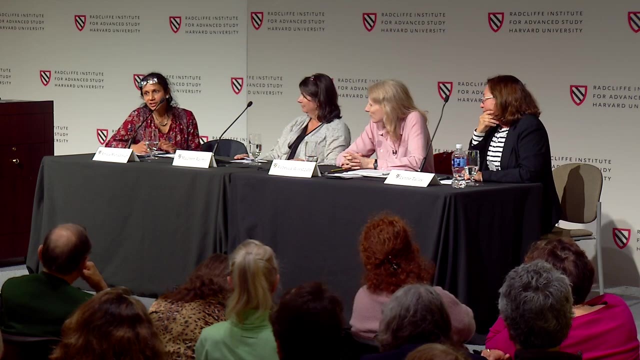 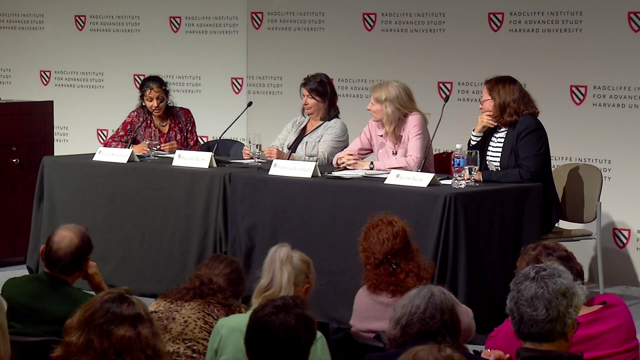 northward onto, it's limited by the size of the Antarctic continent. so I have another question about what oceanographers call the meridional overturning circulation. so the oceans transport heat from the tropics to the poles, and there's been some, a lot of papers that came out. 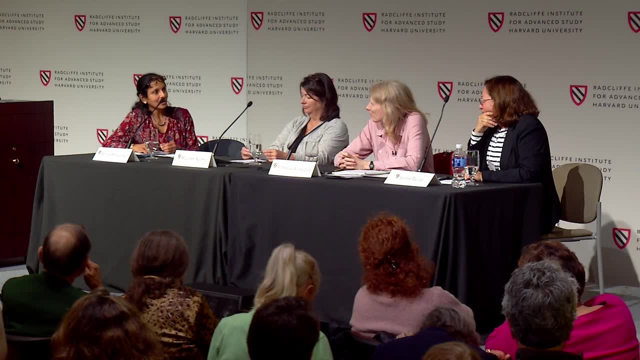 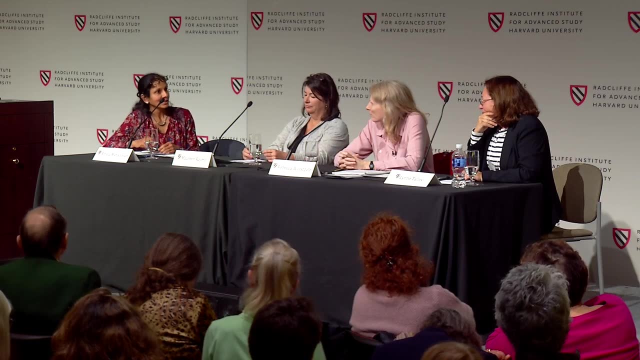 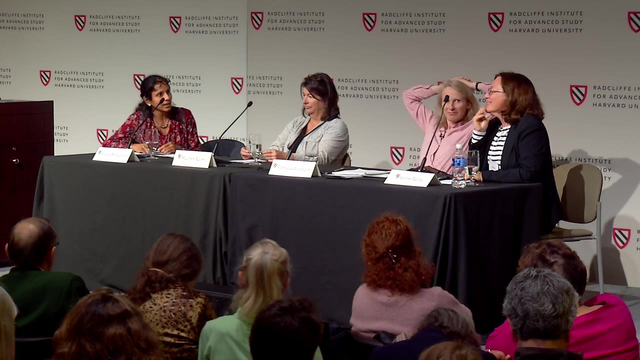 about the strength of this overturning circulation from the paleo literature. we know that in the past the strength of the circulation has changed, and so what is our current thinking? if we melt sea ice and we put all this fresh water up there at the poles, do we think that's going to change the rate of deep water formation? 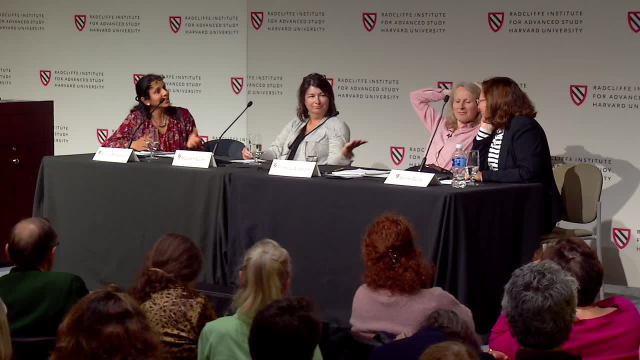 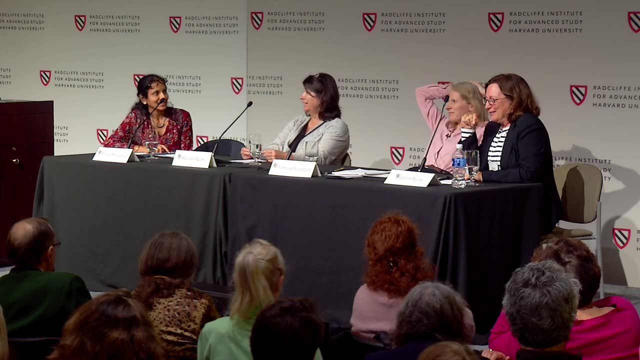 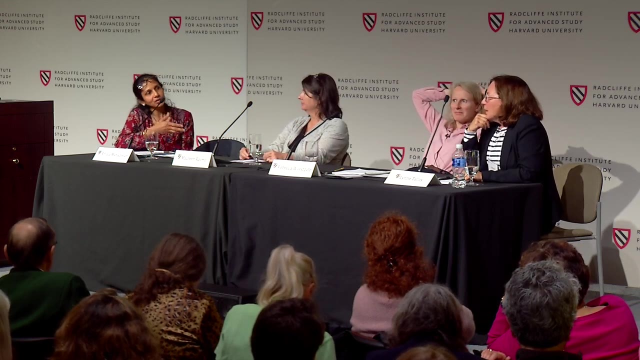 and the overturning rate. do we have any clues in the past? well, you could better speak to the future. it's certainly happened in the past that it shut down- yeah, major reorganization of ocean currents. so maybe you can tell us what you think is happening, might happen in the future. 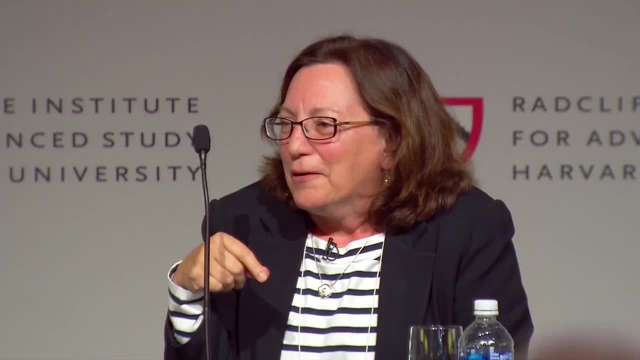 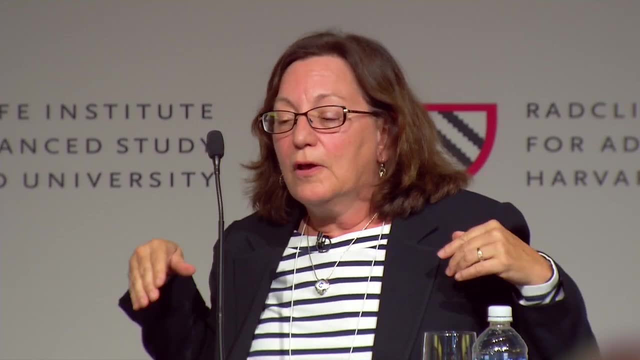 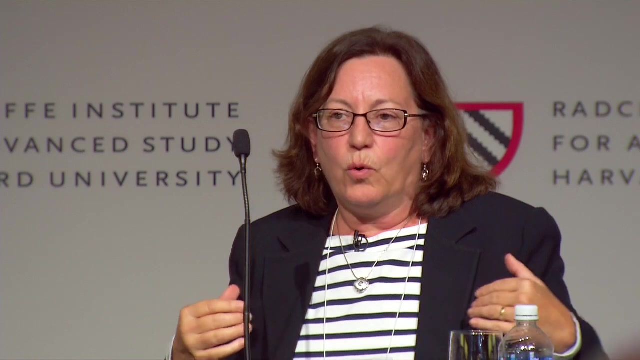 and then Maureen can tell us and then somebody else out there. this is pure speculation in a sense. three slides there. what we're talking about here is the overturning circulation on Rebecca's slides going all the way up into the arctic. that is part of the overturning circulation. 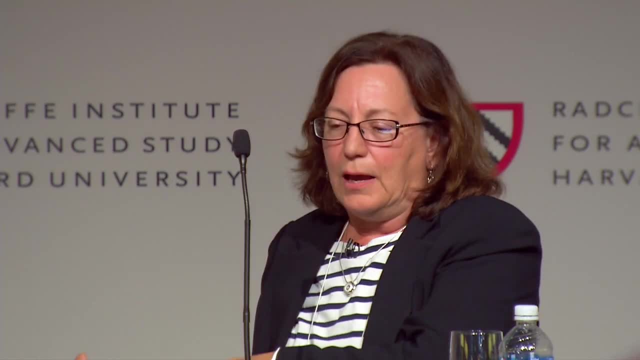 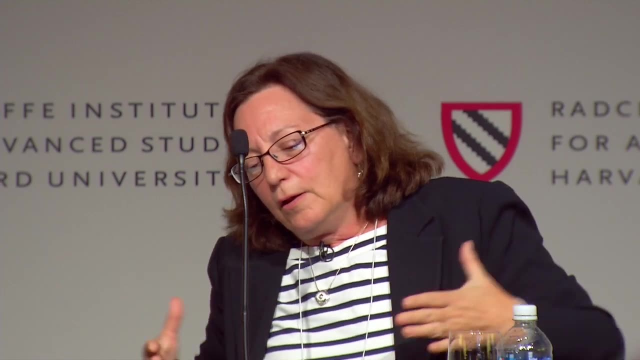 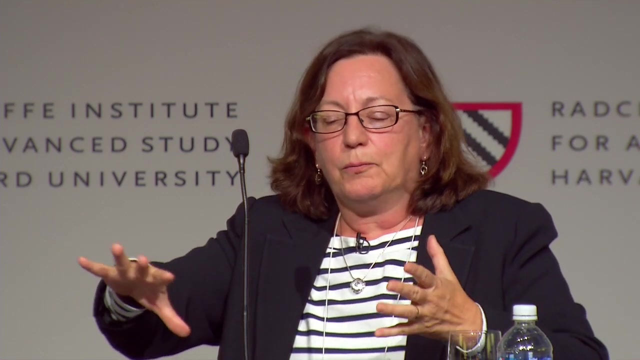 that water is going all the way up there and it's getting cold and sinking and coming out. so that's the north atlantic part of the overturn that that progression of warm water up there is important in keeping passages open. it's part of the western european warming. 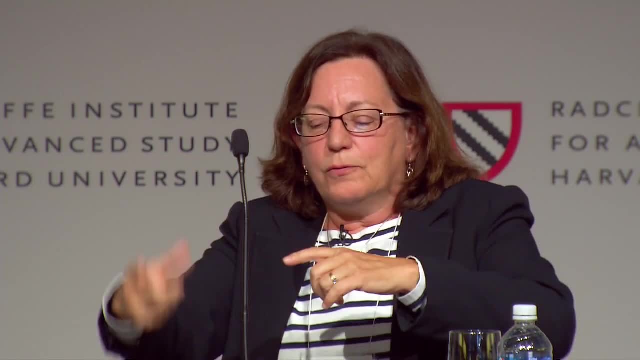 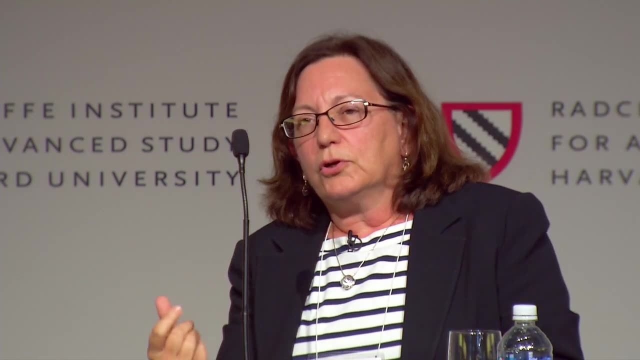 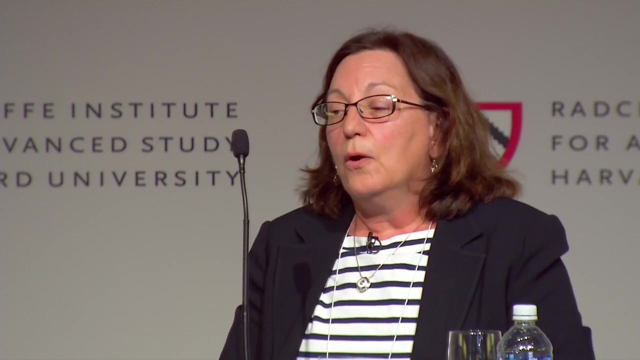 that part. okay, that's the southern part, and the southern ocean is the other. cold part of the world is isolated by the circumpolar current and we have a lot of ice formation right around Antarctica. it makes very dense water that goes to the bottom. so we have these two sources. 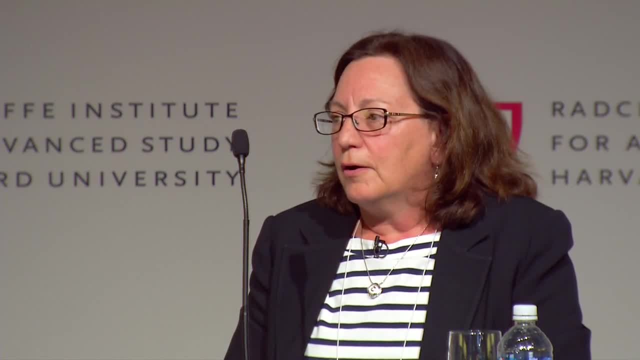 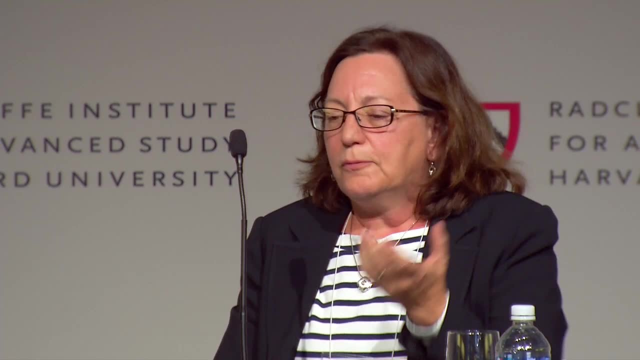 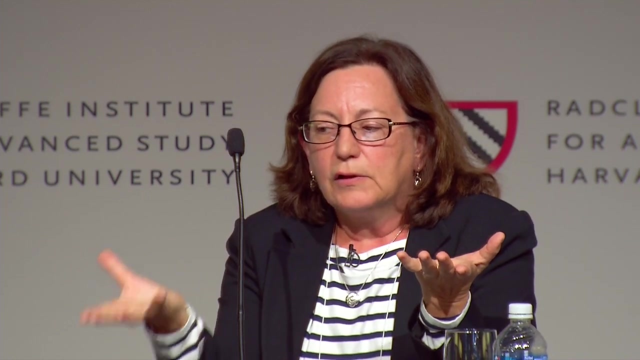 we have one northern hemisphere high latitude source that does not make deep water, which is the pacific ocean, and it's our current experiment in how salt or lack of salt works in the Atlantic is the pacific has a lot of rain and it's very fresh. and the Atlantic has a lot of evaporation, so it's salty. so you put these two things at both ends of your table and you say which one wins. if you cool them both, the freezing, oh, the salty water will get dense and the fresh water will just float. 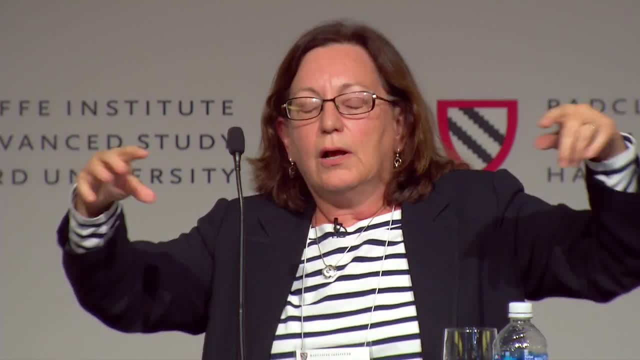 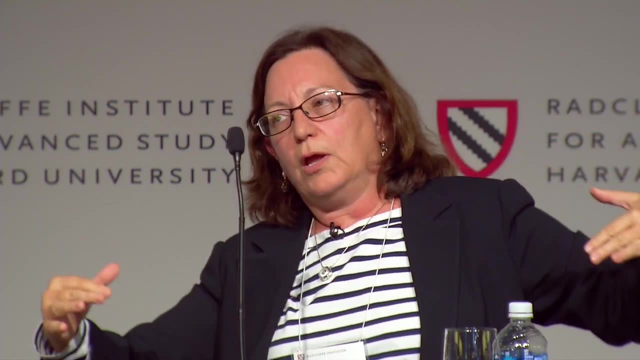 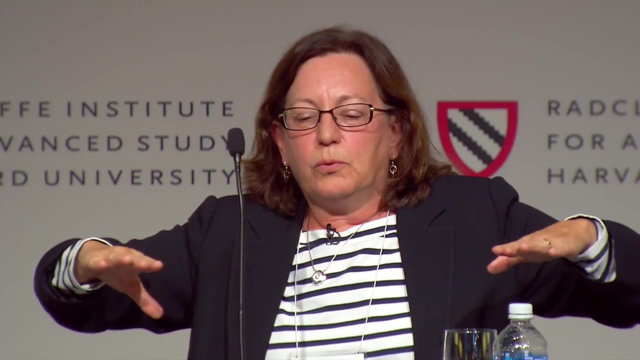 on that salty, dense water. so that's the simple picture set up by Stommel and earlier, a long time ago. we have these two ends and they fall when you move the continents. I think that's tectonics. so then the question is: what's the vigor of those two overturns? the pacific one is weak, it's shallow. the Atlantic one is ten times stronger and goes to the ocean bottom. the question is: if you add a lot of fresh water from all this melting ice on top of the North Atlantic, does it shut that circulation down and then change the amount of warm water moving north? 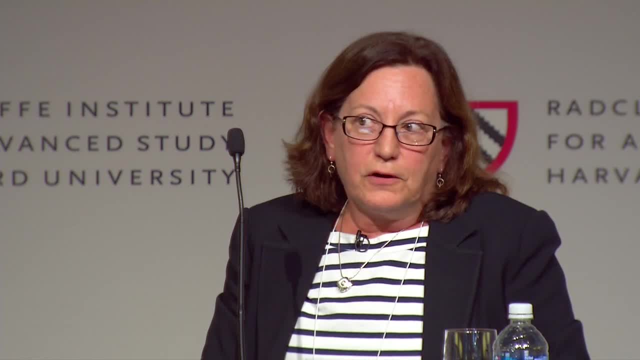 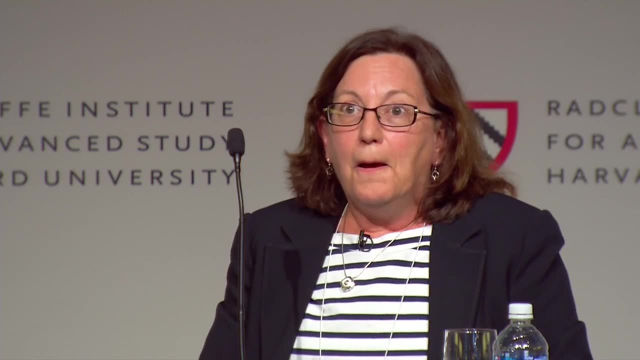 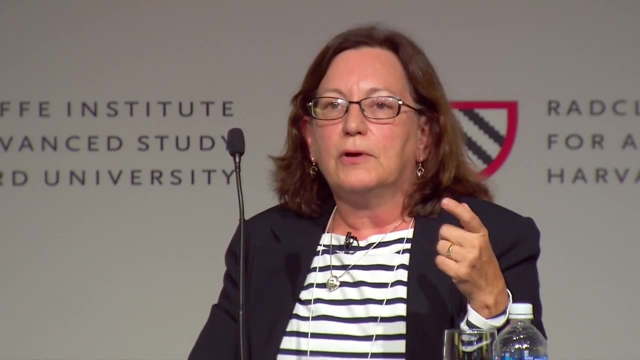 and so we had hints that all this fresh water was starting to weaken things. a decade or two ago, the northern North Atlantic was relentlessly freshening, but it turned around and some of us went. ha ha, the circulation finally caught up all that extra evaporation down off of here. off of the gulf stream over to Europe and Africa. the extra evaporation makes salty water. that got pulled north and it helped keep that cranking. so my speculation is that, yeah, the whole thing warms up, it becomes more stratified. you're dumping more fresh water. 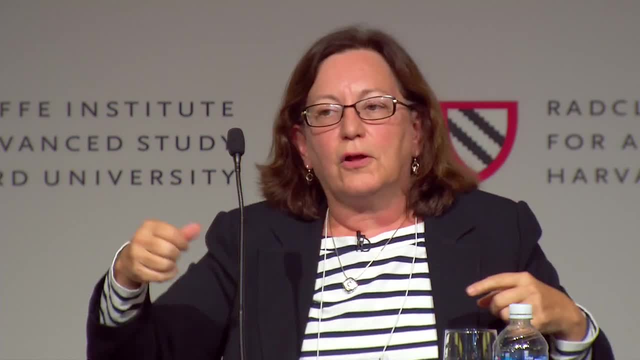 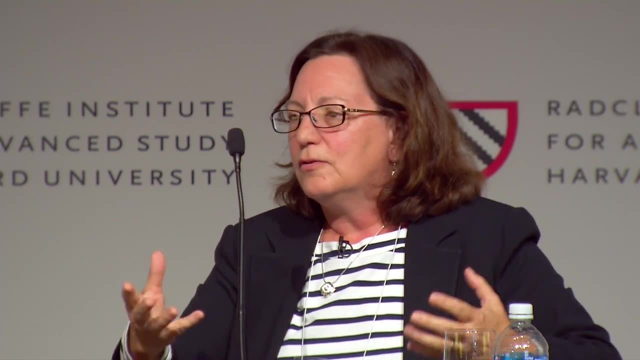 in the north, but you're also pushing all this salty water in. so you've got to have a balance, and I don't know which way the balance will go in the next hundred years. you need to run a lot of models to do that. maybe some of you have done that already. 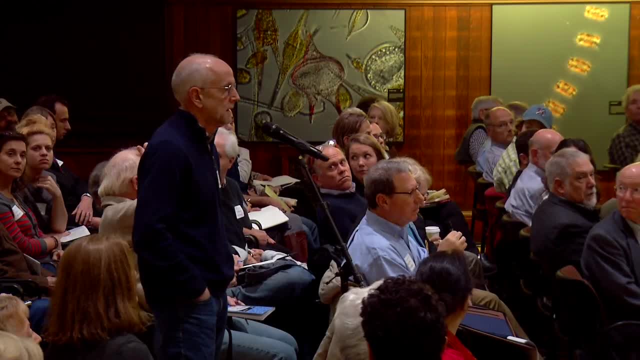 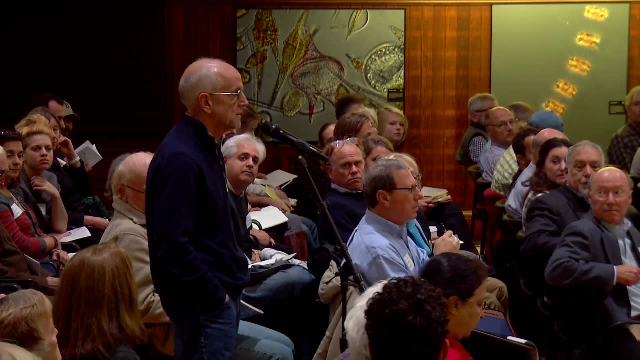 ok, thank you. I'm going to pass it to the audience, because we have quite some questions. my name is John Wigglesworth and I'm a secondary school earth science teacher, and I spent a semester teaching about oceans and climate and I wondered if you had any thoughts. 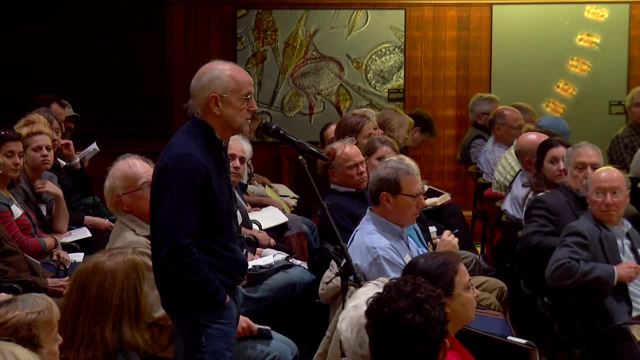 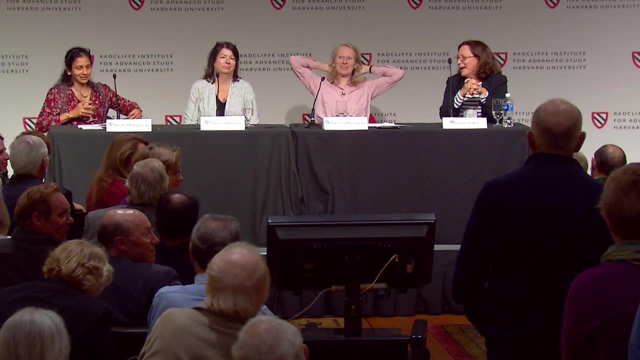 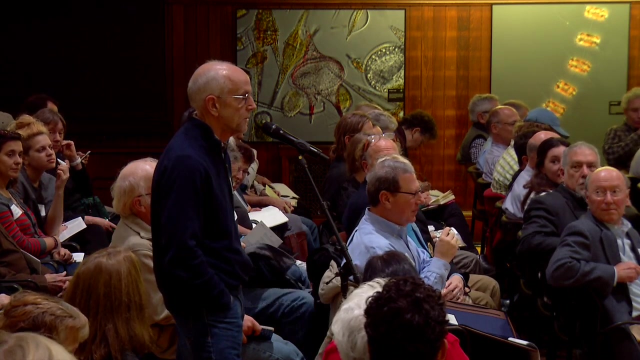 on how to give your message in a way that gives young kids some hope. oh dear, something that I deal with all the time working with 8th graders and juniors in high school, and it's a pretty sobering message. and how do you do it? 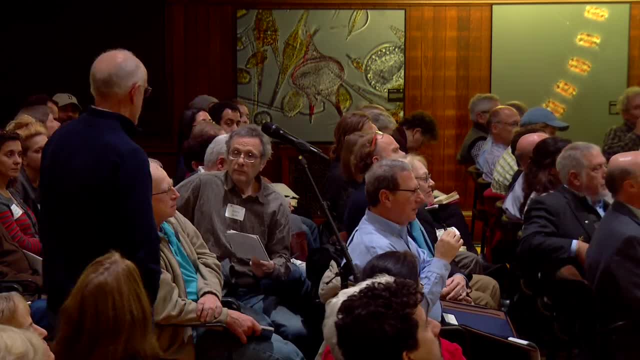 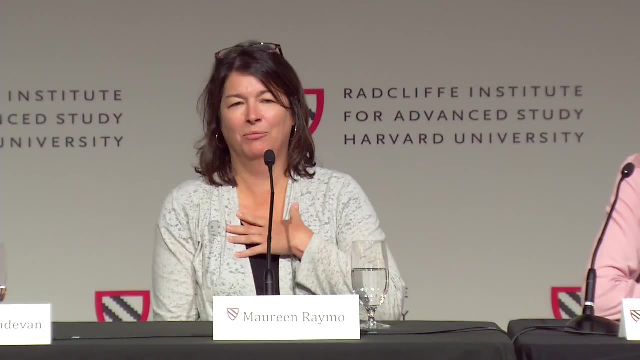 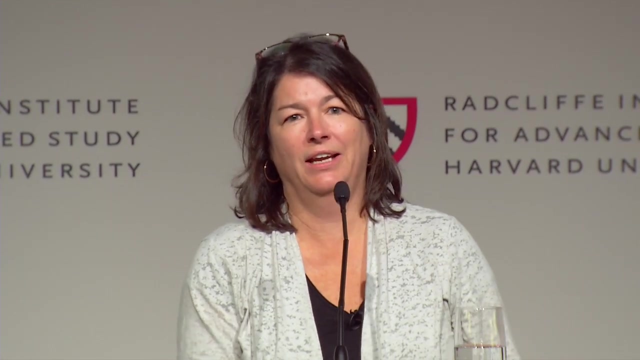 that gives people a sense of hope. I'm happy to try to answer that. so I'm actually extremely optimistic, even though it's a very pessimistic message, just because I firmly believe there is no limit to human creativity and our ability to engineer and our way out of this. 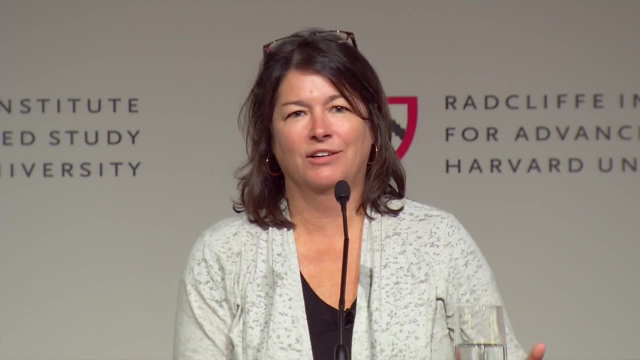 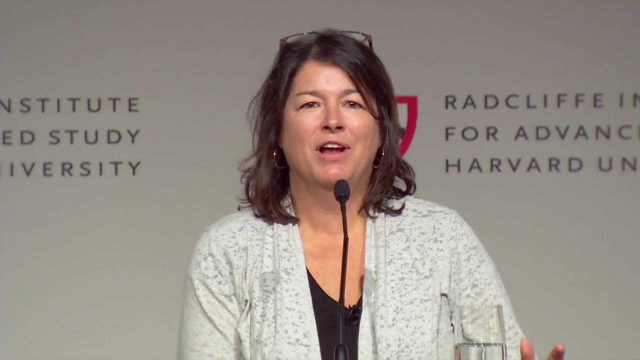 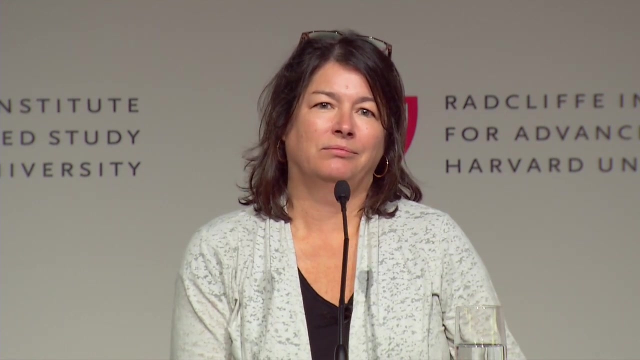 but it has to start with an acknowledgement of the problem and an effort to reduce CO2 emissions. so I'm not sure, but I think people have to be empowered by a knowledge of the problem and want to solve it. so I would add to that: I struggle with this too. 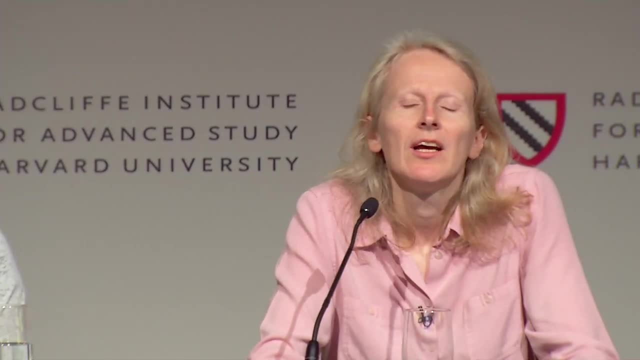 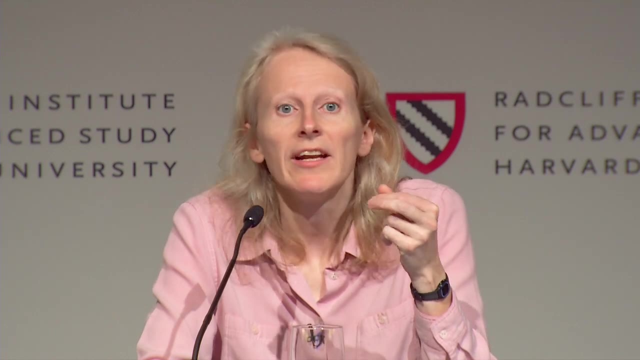 I teach a class on the Arctic and you come to the end and you think: how can I end on some positive note? and I think it's to remember in that that we do have the ability to change this. if we go out there and say we're going to throw all the money. 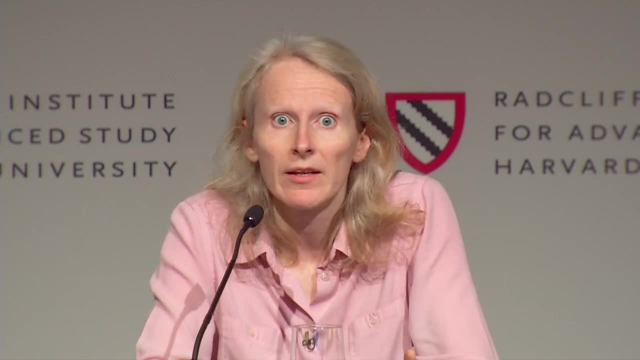 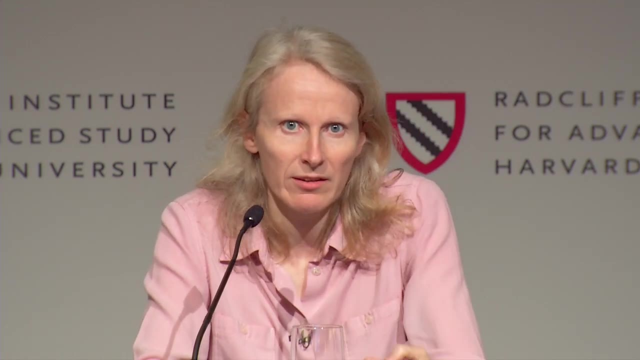 that we're putting into making ourselves rich by solving this problem. we can do it. perhaps the most positive thing I saw on this was somebody said: right, I know seven technologies that could chip away at a seventh of this problem, of the CO2 problem, but we have to teach the people. 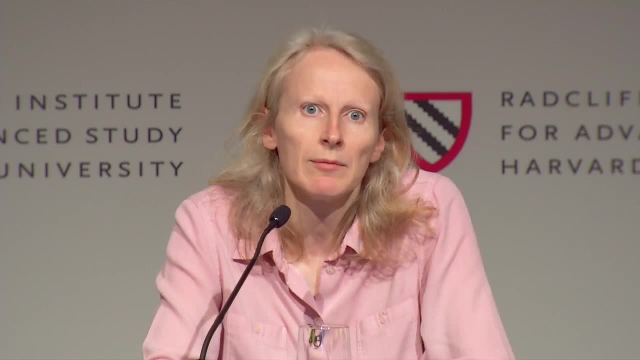 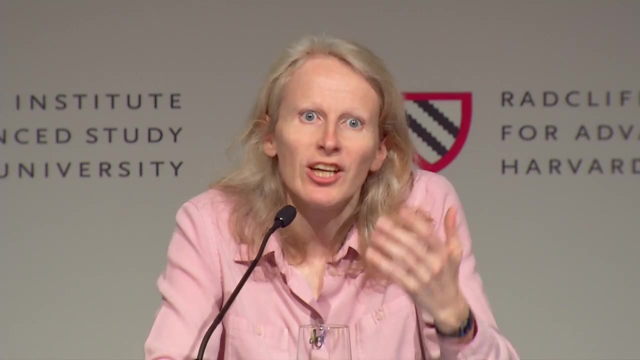 that this is happening, that we have to face up to it, like we teach people to face up to problems in life and go in and do it and find on the way, some way of predicting and mitigating it. so it's their future and I hope we can get them to grasp it. 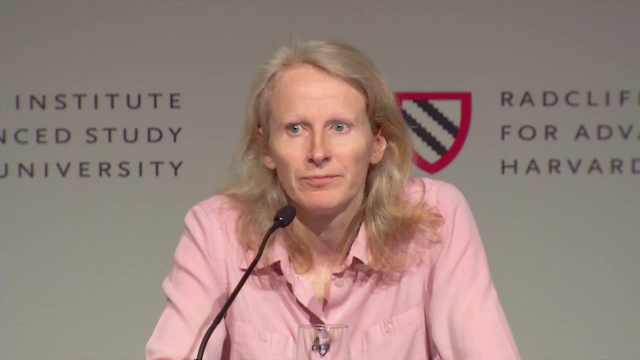 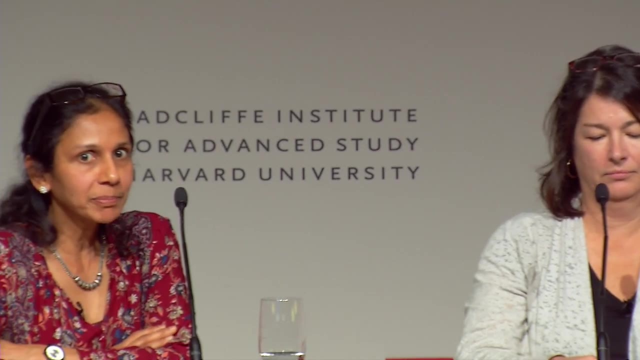 and do something about it and burn it all on our watch. and I think something we can add is that there have been other problems for which there was no political will in the past, but when public opinion changed, political will came about, so I think there's hope for that too. 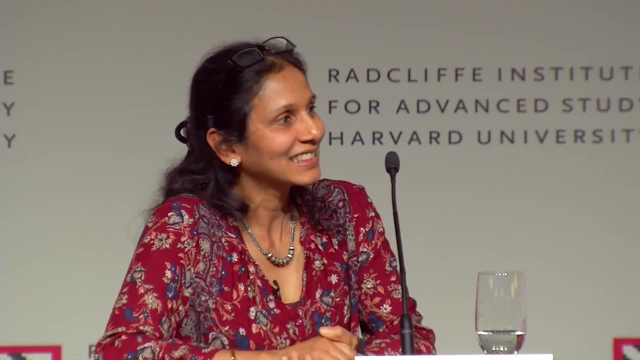 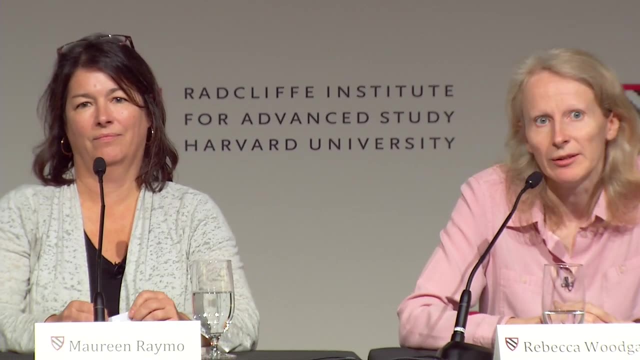 so take the CFC ban. we managed to ban CFCs because that was a science problem. so we can do it. we just have to team together and actually do it, okay. so the next question. we're going to have to be a little quick because we have five minutes. 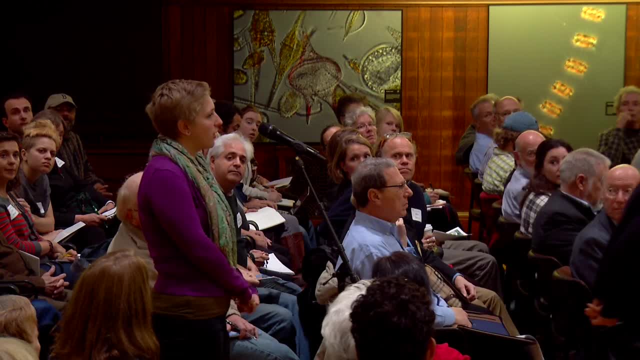 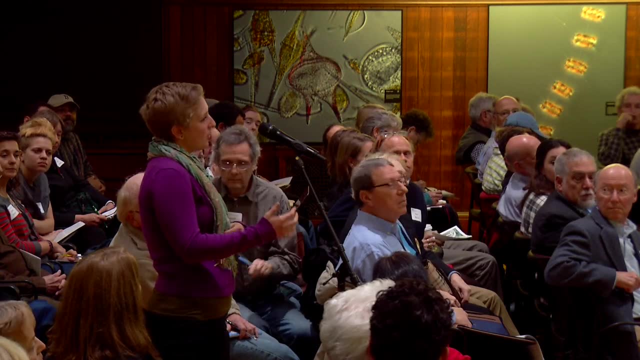 I'm Tina Hernandez. I'm a graduate student in the MIT Hui joint program in oceanography and I had a question for Rebecca about sort of ice edge blooms and the effect of melt ponds on under ice blooms, and so I was wondering if ocean color changes. 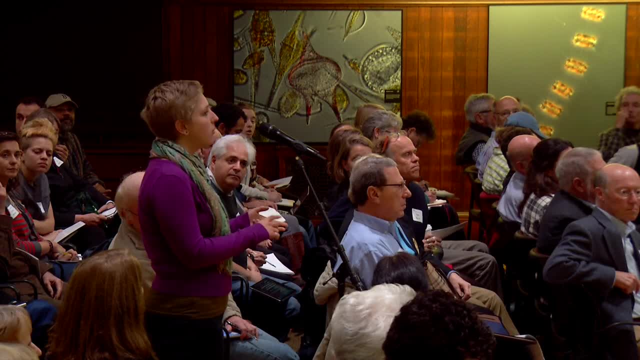 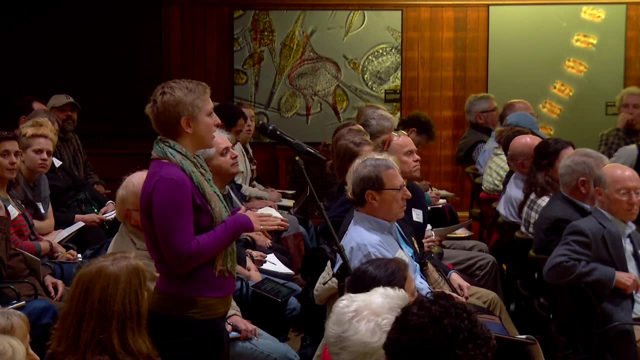 whether those blooms happen under the ice during melt ponds or at the edges, if that contributes at all to these positive feedbacks that melt the ice like: do you know anything about ocean color? okay, so this is really cool if you have a phytoplankton bloom in the ocean. you need to have nutrients, stratification and light. if we get melt ponds in the ice, we get like windows in the ocean which are allowing light to come into under the ice regions which we always thought were devoid of life until the ice had melted. we are finding there are those blooms in some places. 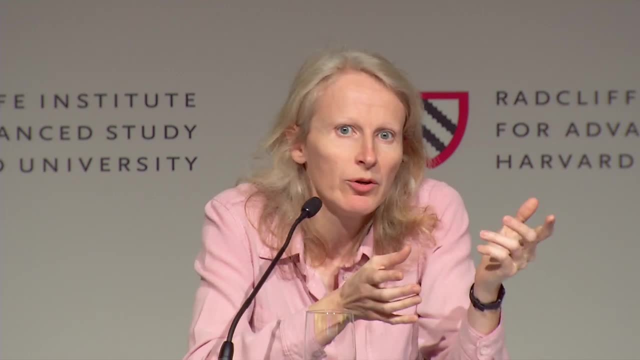 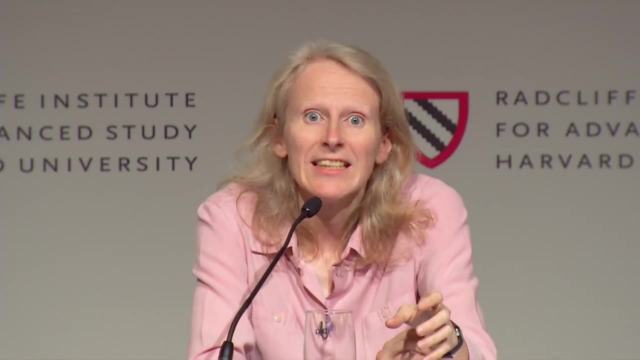 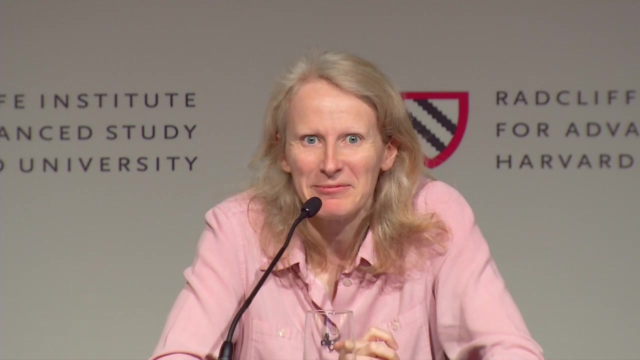 quite why, we don't know. we think because of the melt ponds. have they always been there? we don't know. what is the feedback then from that phytoplankton? some don't quite know. we are kind of working on that. Marla and I are working on that at the minute. 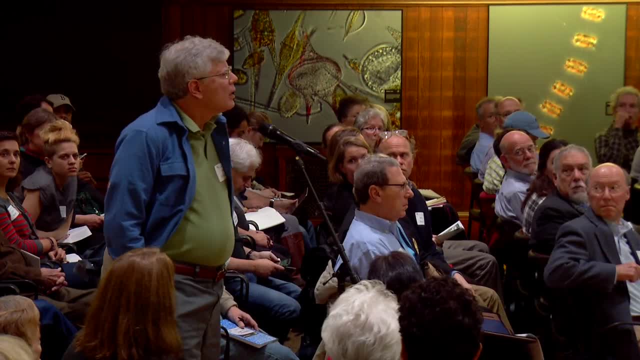 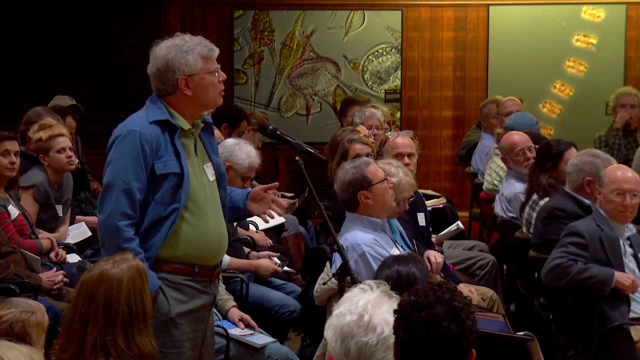 so we can talk offline. that's really exciting. My name is Tim Johnson and I am a software engineer and I have one, I guess, a futuristic kind of question in that it sounds like we are heading for sort of an alien world. we don't have to travel to another planet. 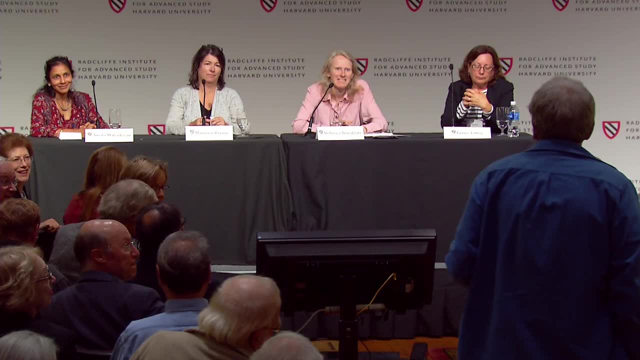 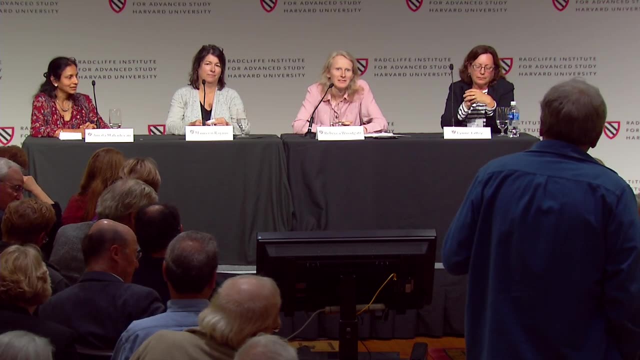 to find an alien world. we are going to get one right here. I met that somebody was from Kuwait and to me that seemed pretty alien and it seems to me that we are almost can't stop what you are describing, even if we became much more politically active. 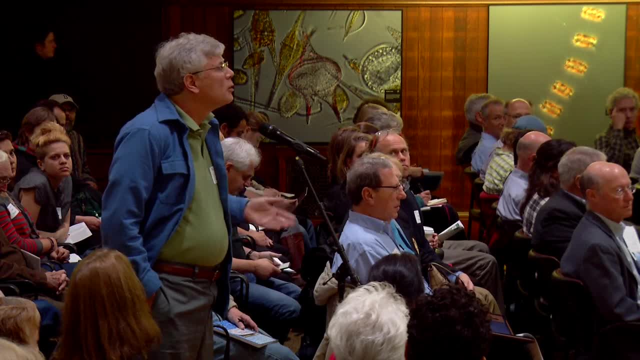 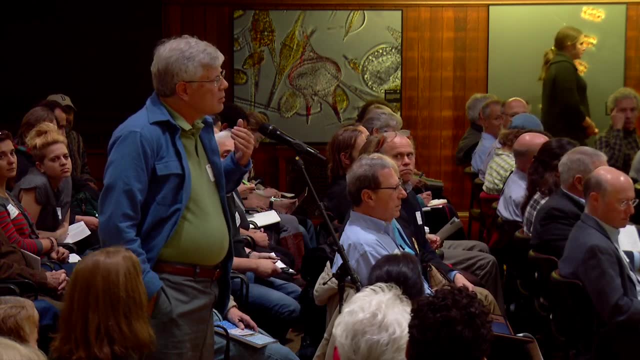 and the Republicans suddenly became totally different. we are still not going to change very fast, even if they change it tomorrow. passing legislation, changing things, and so it seems to me we have almost a whole new area of science of how to deal with the fact when the world is going to change. 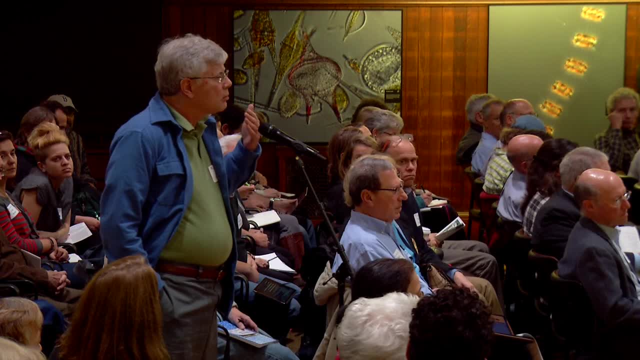 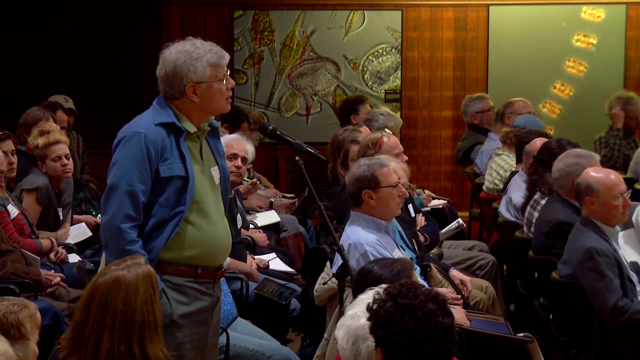 over the next century, because it really is. is this sort of something people are thinking about looking at how to make money? like you can have tours taking you through the Northwest Passage, which didn't exist before, but it seems like sort of a big area. I suppose it is a way to make a lot of money for some.